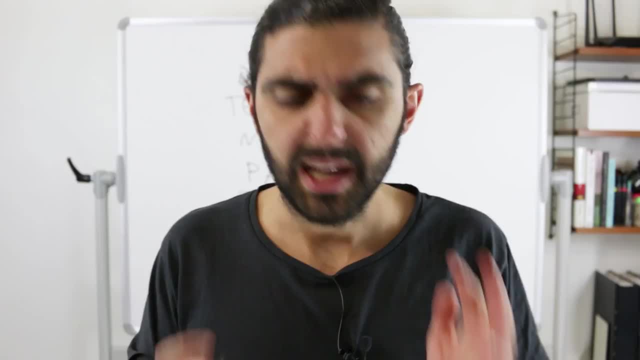 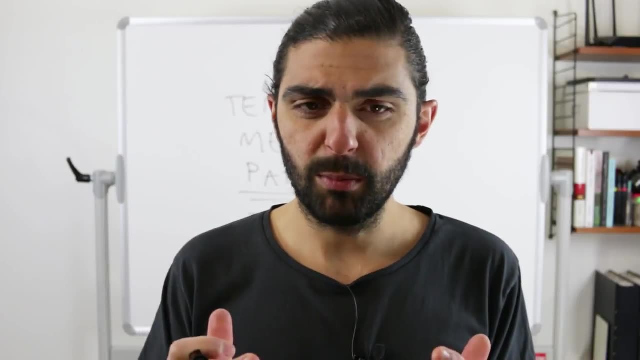 blueprint the class into an actual instantiation, And this might sound a little bit strange, but actually I think this pattern is going to be fairly easy to grasp because you are most probably intimately and intuitively familiar with the idea of a template. So let's start in that. 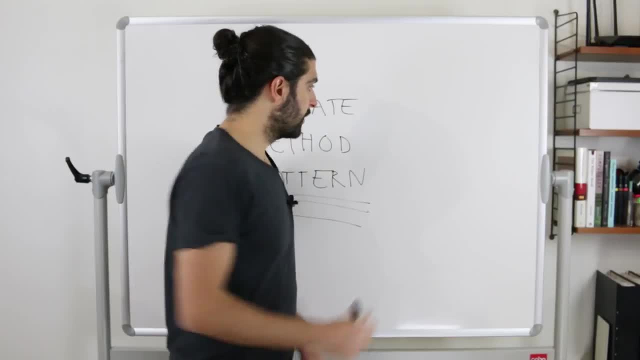 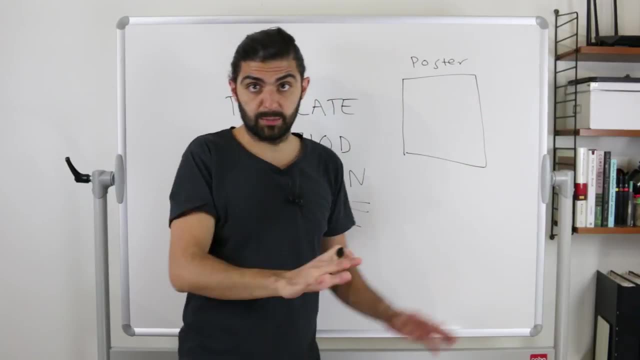 Let's talk about what a template is. I mean, think of it this way- Sorry for going all physical papers and 1990s on you, but think about a poster, a physical poster that you put up somewhere. If I'm not a graphic designer, for example, I don't know Photoshop or I don't want to spend 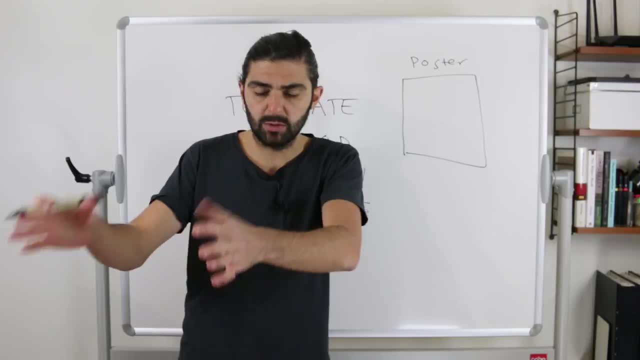 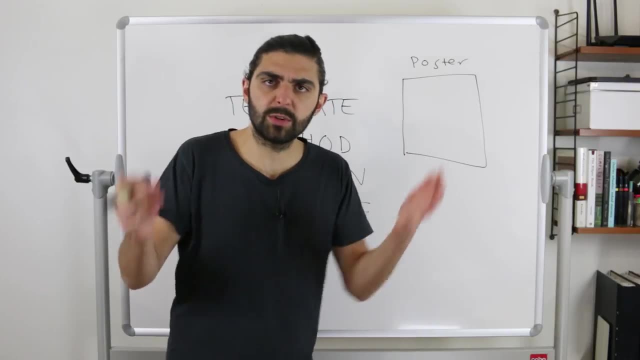 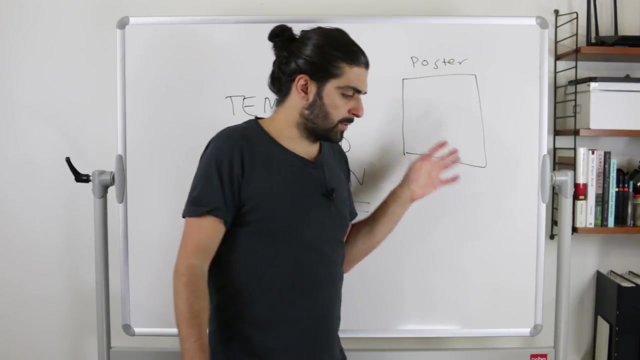 time doing it And I just sort of want to poster out, but I don't necessarily care too much about the graphics, Then I might employ a template. So templates exist for a number of different applications, such as word processing applications, for image processing applications or whatnot, But let's just think of this poster, right? So 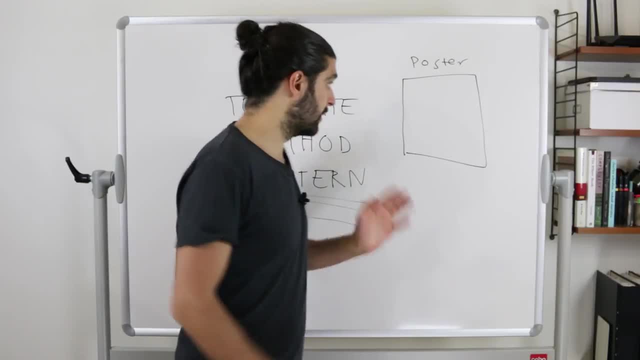 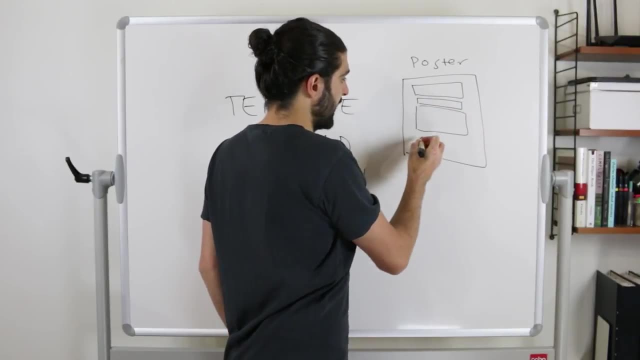 somebody might then hand me a template, right, And say, okay, this poster will have a title, let's say a subtitle, a huge image and then some text here. I don't know, I mean, it doesn't matter. 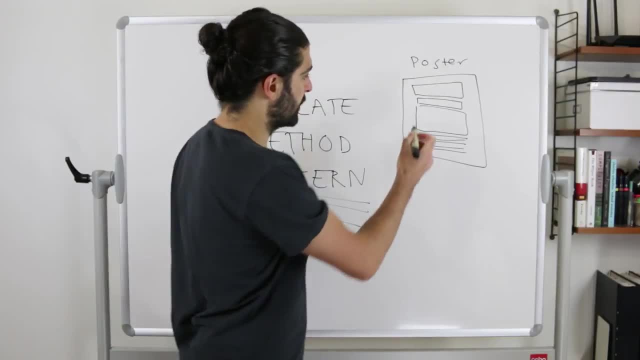 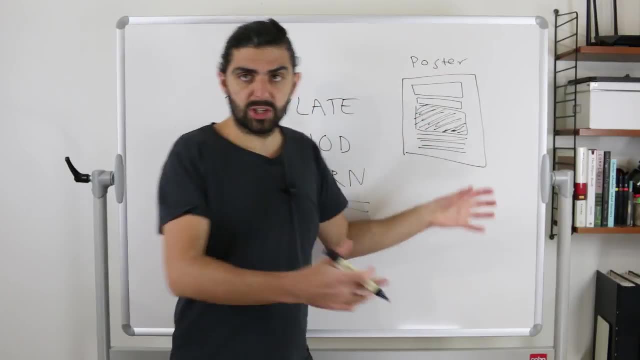 But the point here is that you have this template of a poster where you say that this piece here we need to have an image, But the person who designed the poster template doesn't know which image I, the poster creator, want to use. The poster template creator doesn't know which title I want. 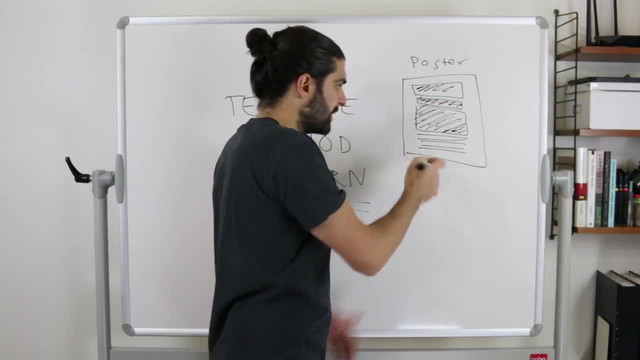 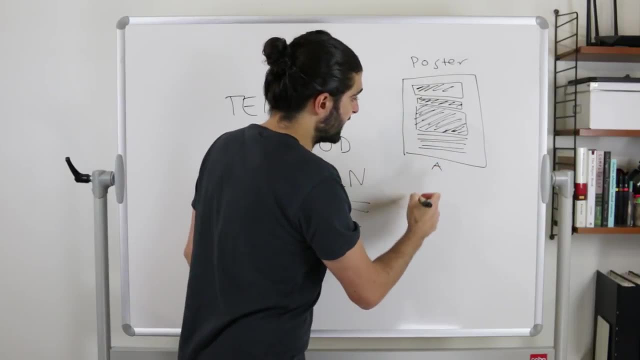 to use, nor which subtitle I want to use. Doesn't know the picture and doesn't know the text, right? But the template creator can say that actually we have a few different templates. This is template A, and then maybe we have template B and template C and whatnot, And I mean clearly. now this is. 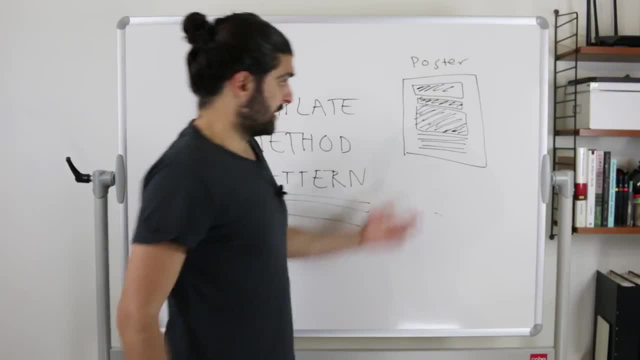 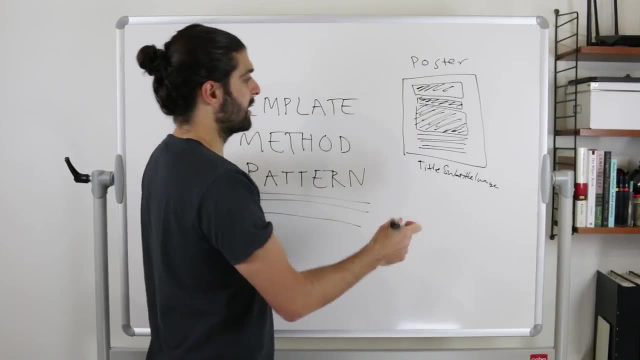 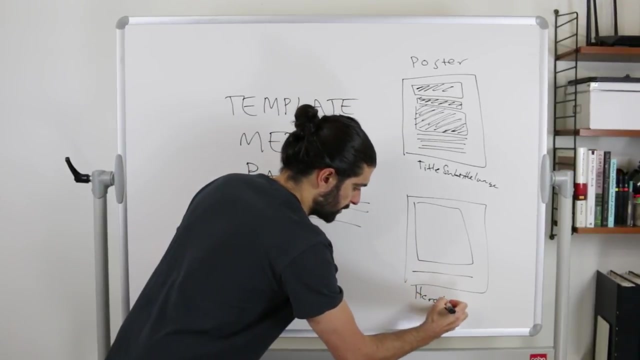 okay, to make the example a bit more sane, maybe they would say that, okay, this is a, you know, like a title, subtitle, image, poster Template, And then they maybe would have different one which is like title and image, And then maybe they call this a hero poster. 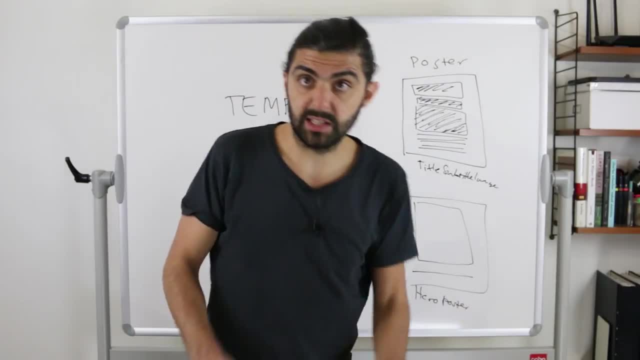 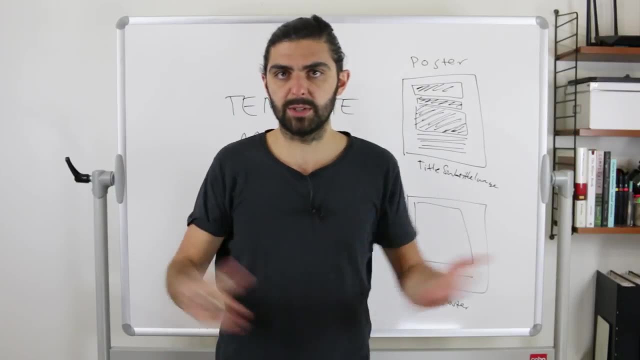 something like that. I mean, it's not strange, right? If you go to a printing agency, they might have a bunch of different templates that you can say, okay, you pick and choose and you say, okay, I want this one. Here's my text and here's my image. 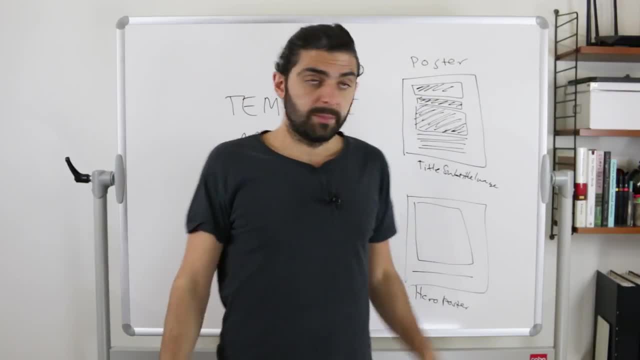 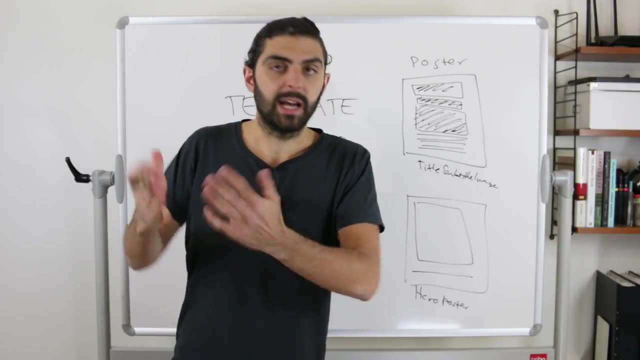 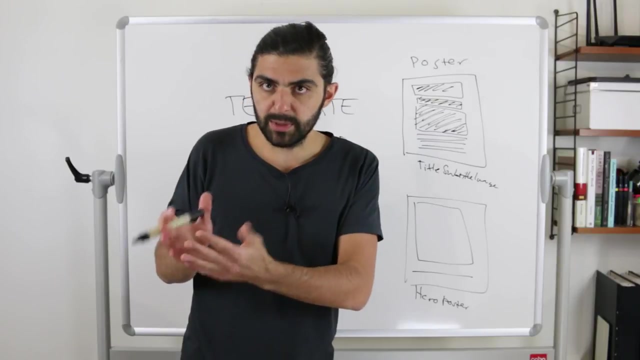 And then they compile it for you Enough from that example, right. But if you think about that, that intuitively makes sense. There's the notion of a template, a blueprint, a class, right. And then you can instantiate that and you can create instances of. you can take the blueprint and build something from the blueprint, or take the template and fill in the blanks of the template. 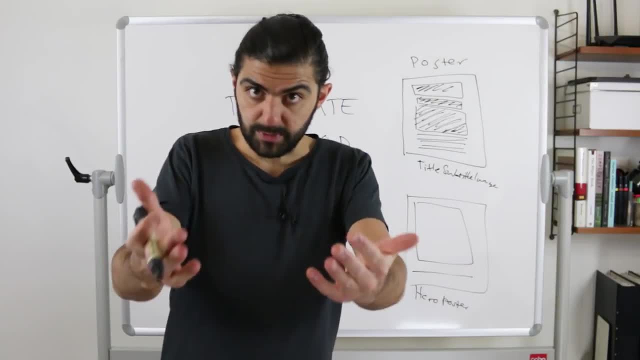 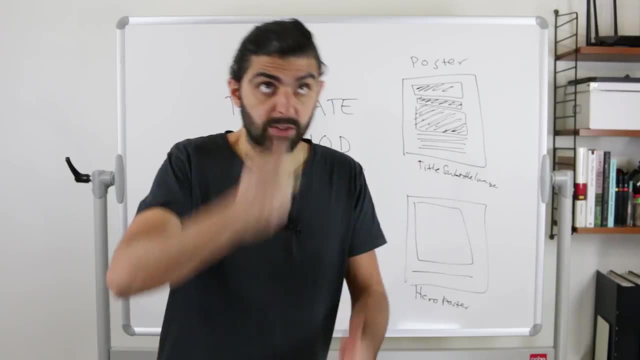 Ah, just think about it that way, right? Maybe you've received a PDF at one point where it's like: okay, start filling this PDF please. In some sense, that's a template. They're giving you a template, you're filling in the template and then you're handing in the document. 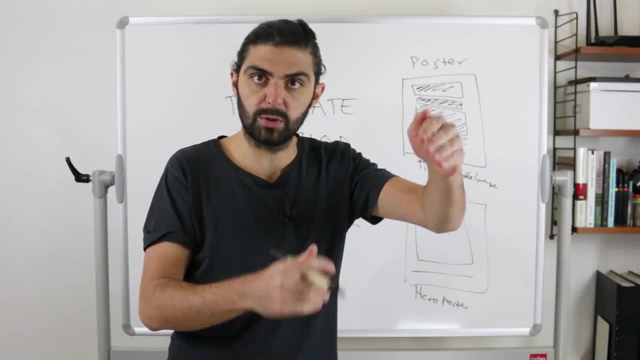 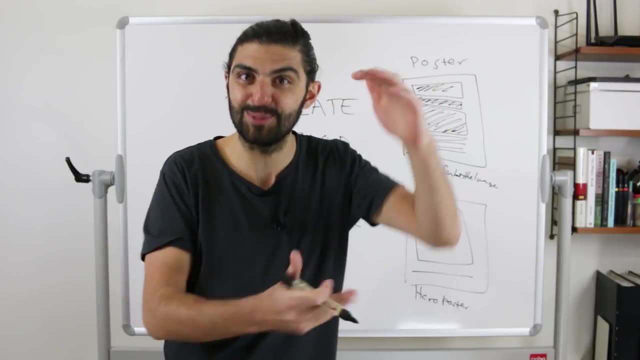 Because when you're handing someone that physical document, what they care about is that physical document and the information. They want it in that format. They don't want to have everyone who's supposed to hand in that paper to have to redesign that paper from scratch. 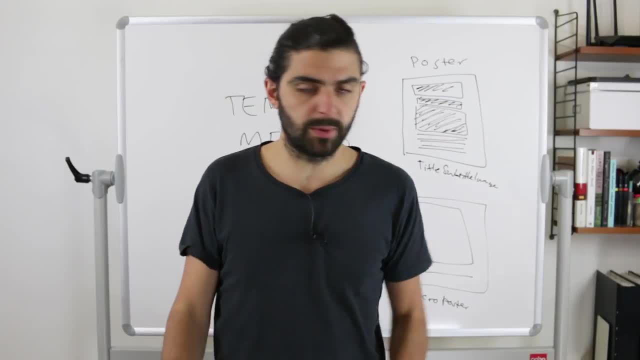 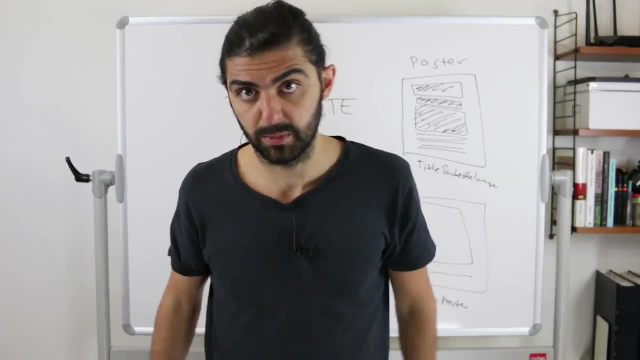 I mean maybe this is like, I don't know, applying for a job or reporting hours. or I mean this is a bit silly because in this day and age these things should probably happen in a system and not on a sort of document level. 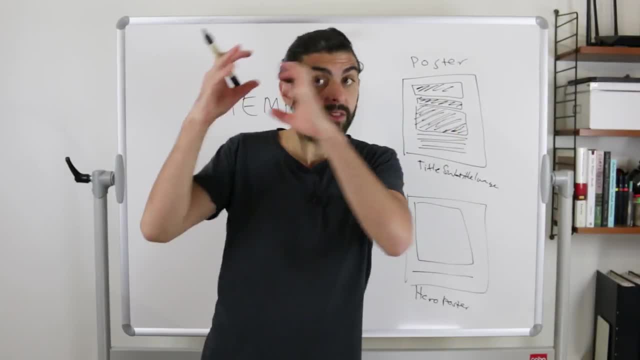 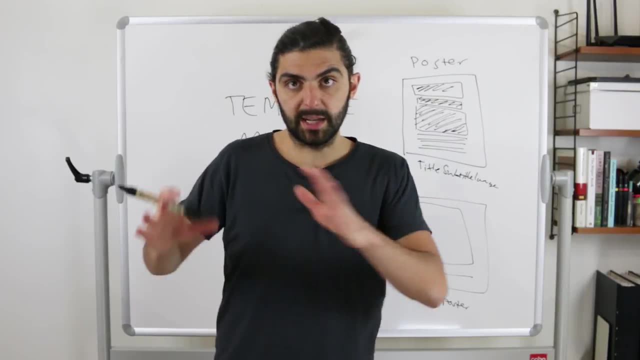 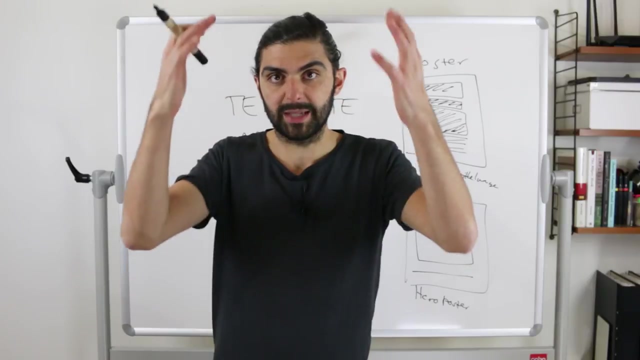 But then just think about the poster instead. So you have the template and then the thing created from the template, and a template might have multiple different instantiations. And you should note here that I'm using the word instantiation Here lightly or metaphorically, because you are familiar with object oriented programming and the notion of a class and an instance. 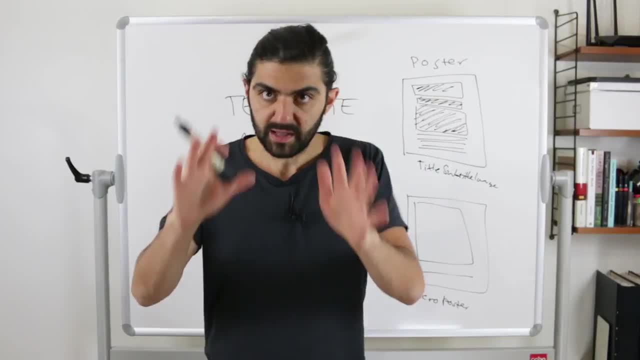 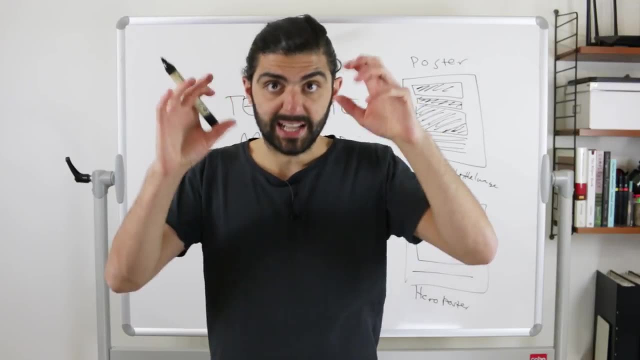 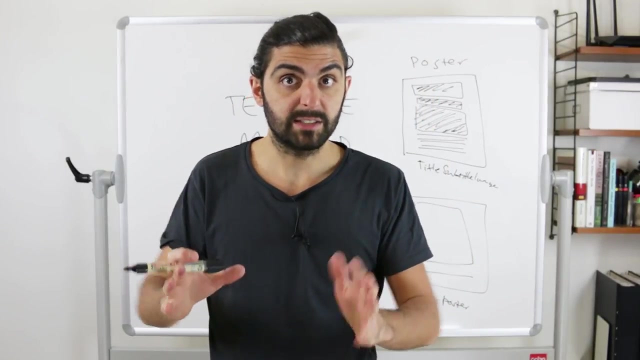 I'm using that notion metaphorically, because the template method pattern will actually make use of subclassing. So it's not that we have a template that then is instantiated as an instance. It's actually more that we have a template that you then subclass to create a specialization, a concretion of that particular template. 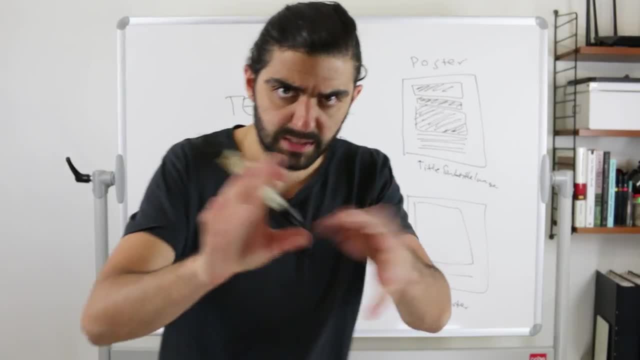 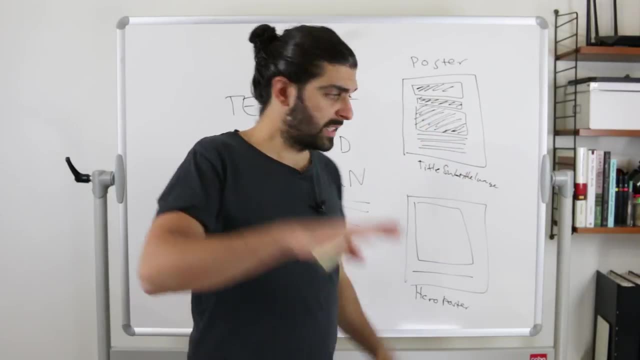 And then you can instantiate that specialization. But now we're getting a bit ahead of ourselves. So we've probably nailed this concept of like a poster and the template for a poster. So let's slowly move into the notion of the template, method, pattern. 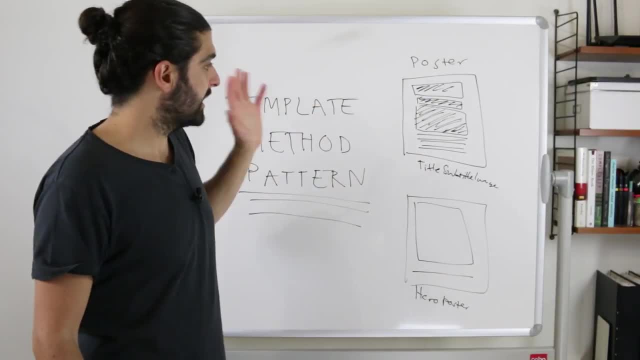 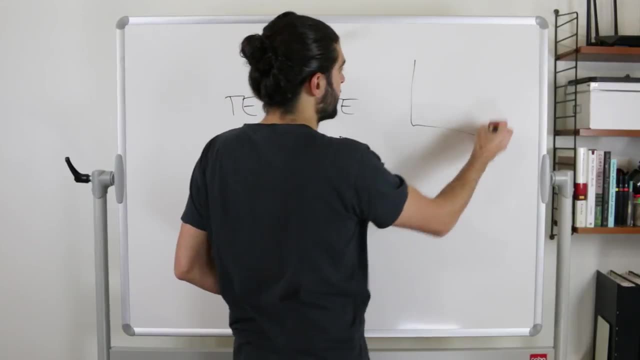 If you think about it hypothetically, you could have an algorithm that describes how to produce a poster. So, to simplify, let me just remove these two posters. Let's only care about the hero poster, for the very simple reason that it was simpler for me to draw. 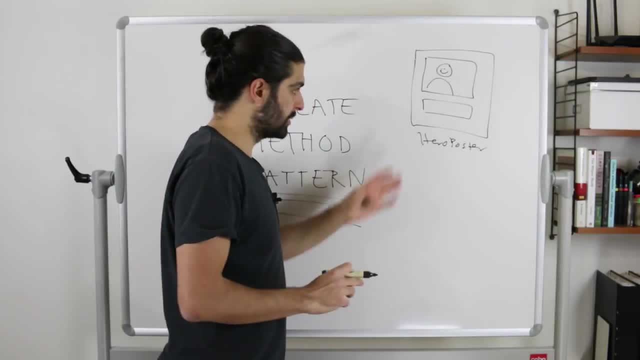 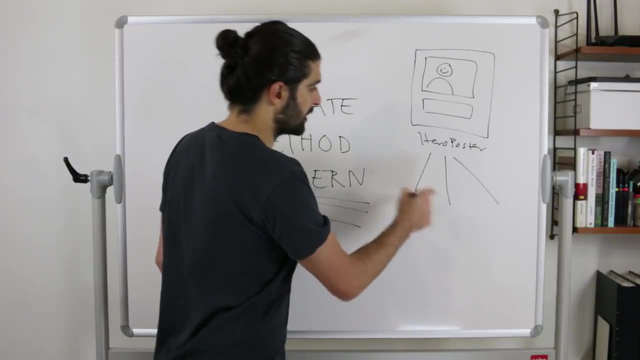 So I'm going to say this hero poster. Let's say that there is an algorithm to produce this hero poster And then we have a number of different clients coming to this agency and producing different posters. Let's say this could be poster one and poster two and poster three. 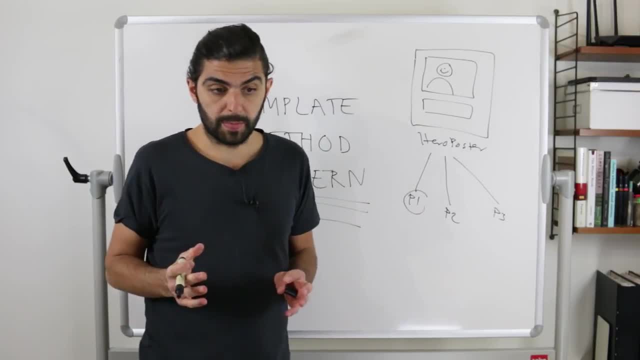 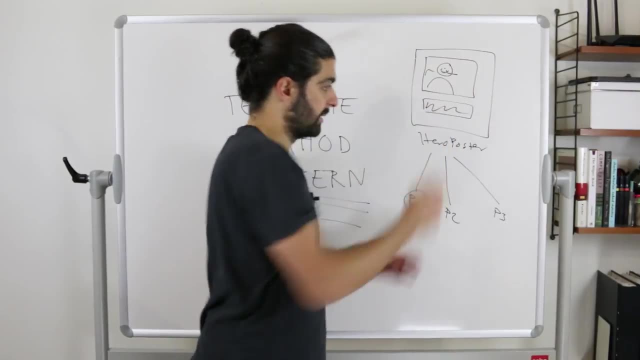 But just to exemplify, I mean, maybe poster one is: is a band coming into the store like a music band and they want to have the title of the band and then they want to have a picture of the band members here, right? 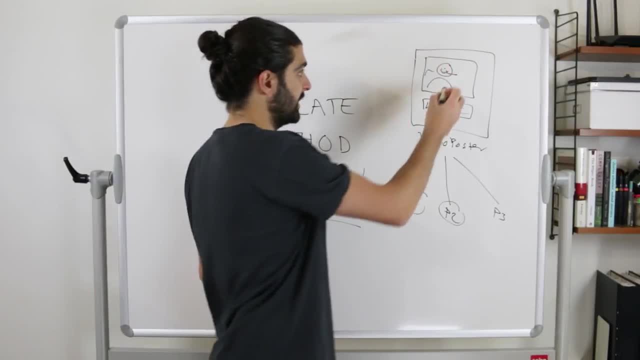 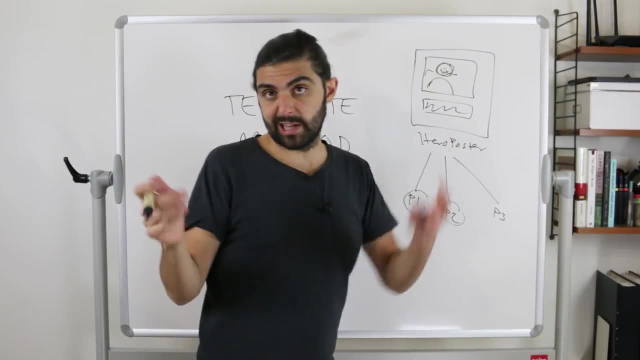 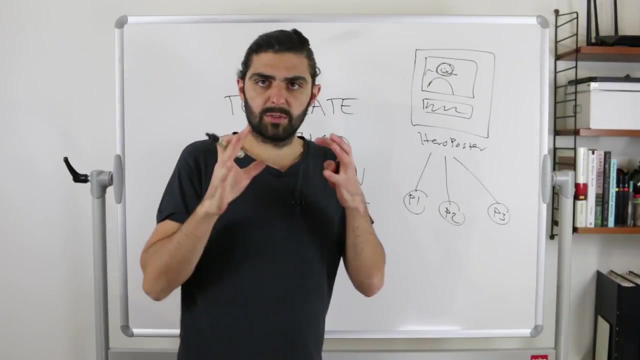 Poster to two is maybe Representative of: comes in and they want to have this politician depicted here and then some kind of election promise or whatnot, i don't know, or like a speech date or something like this. poster three is well, something completely different, right? so these are concrete scenarios of clients coming in and asking: 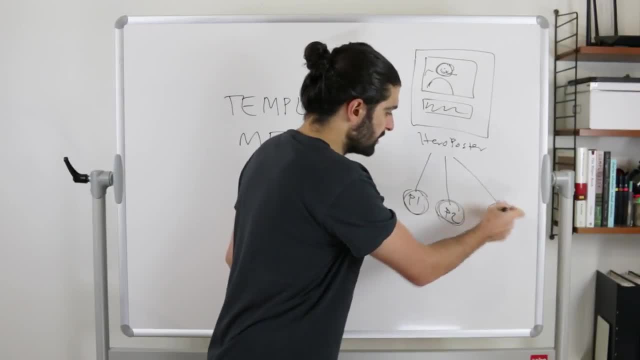 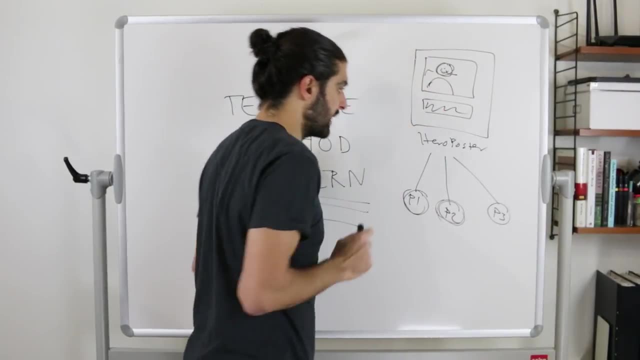 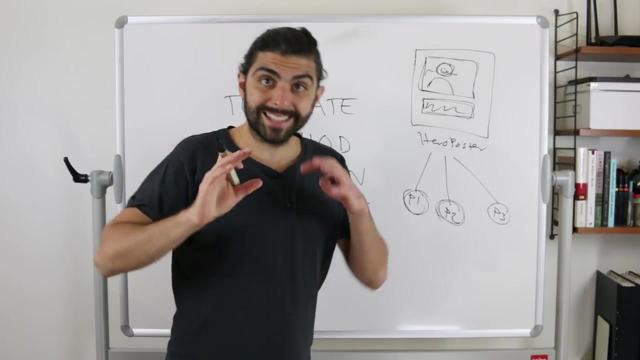 for specific posters now. so what varies amongst these p1, p2, p3, these different, three different posters? what varies is the contents, is the picture and is the text here. what doesn't vary is the fact we have a text here and the fact that we have a picture here. so if you think about it as an 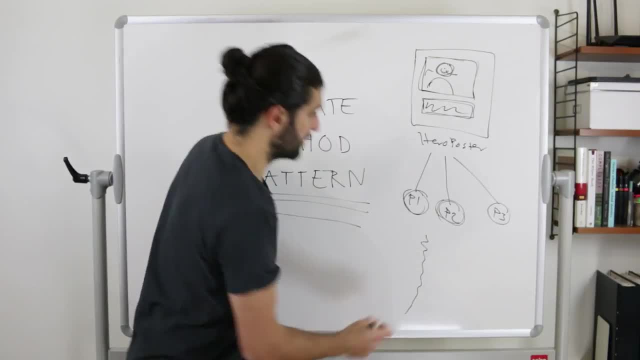 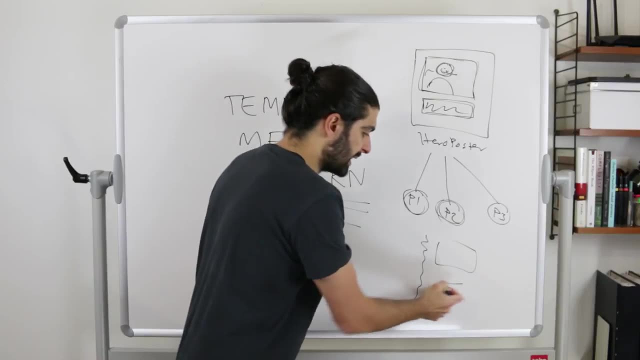 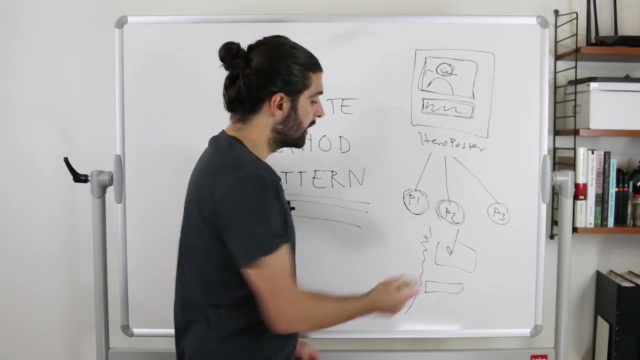 algorithm. there's an algorithm for producing this picture right. some of the pieces of the algorithm don't vary, such as put in a picture and put in a text. how to actually get that picture that varies, or what that picture actually is that varies, and further, how to actually get that text or what that 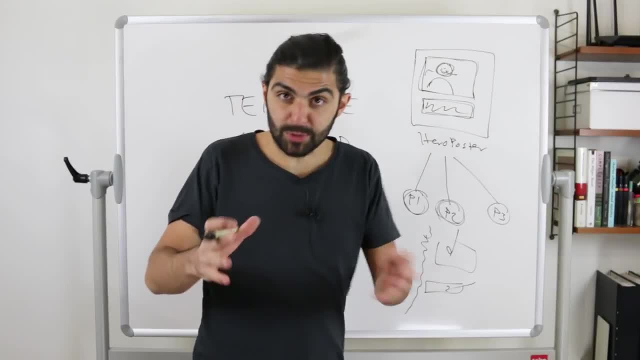 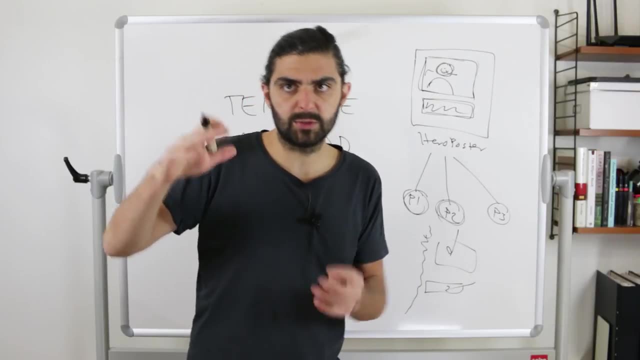 text actually is is what varies. so, as almost always with the design patterns- kiss instance- the case is that somebody noticed that I have this sort of reoccurring scenario where I have this one thing that varies while this other thing don't vary, And then they're trying to 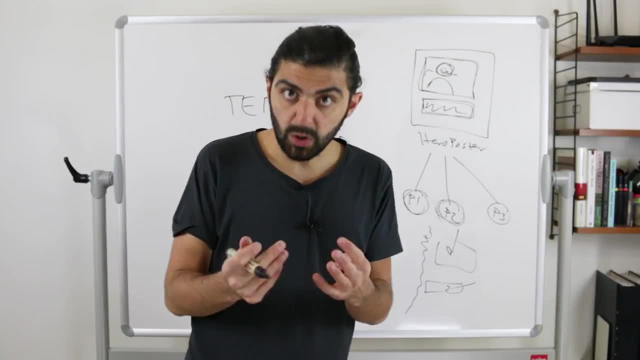 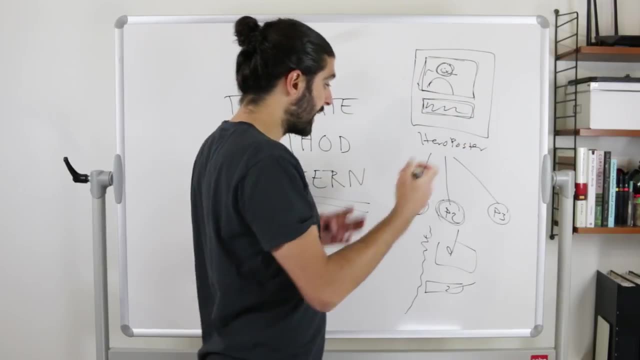 architect a solution such that you don't have to duplicate code for the thing that doesn't vary? The thing that doesn't vary is the fact that we have an image and the fact that we have a text. So how can we have an algorithm produce pollster? let's say, Produce pollster right is a method. 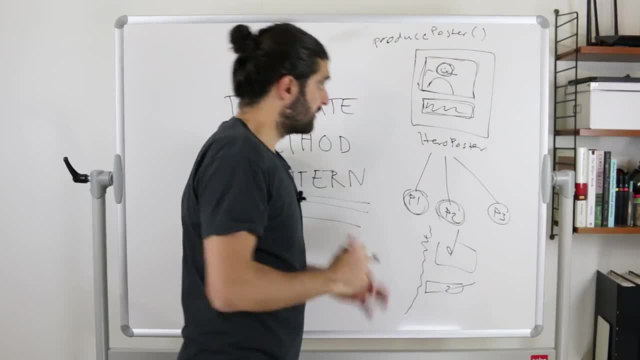 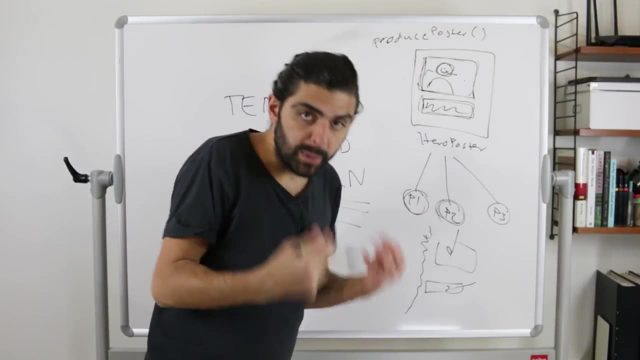 that somehow returns a pollster. How can some pieces of that algorithm, ie the notion of having a picture and the notion of having a text, how can we make sure that that's not duplicated across every occurrence of a pollster or every different specialization? 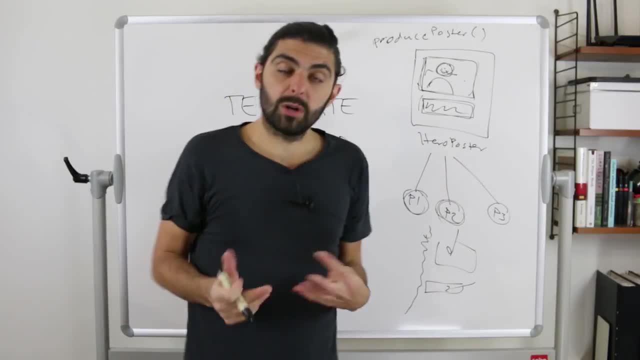 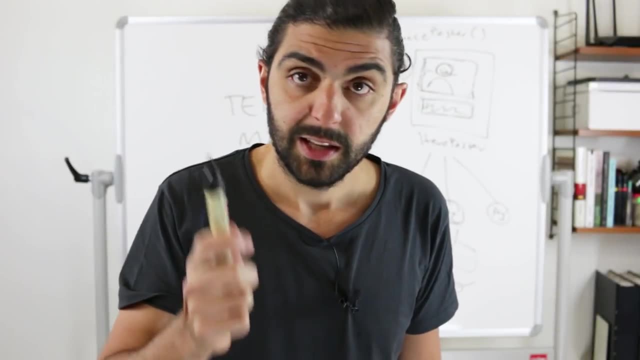 I should say specialization of a pollster. That's the job of the template method pattern. So we'll get into the definition of the template method pattern in just a moment. but I just want to mention that the example that we'll use later is from frameworks, Because if 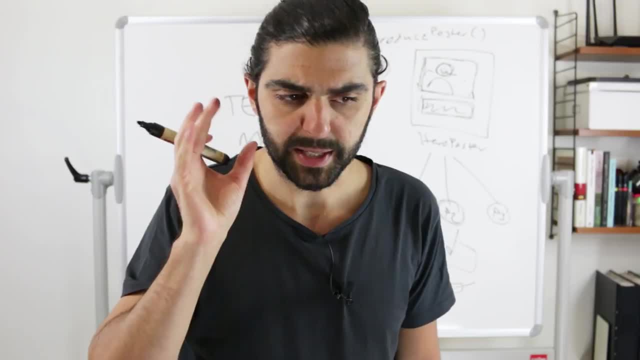 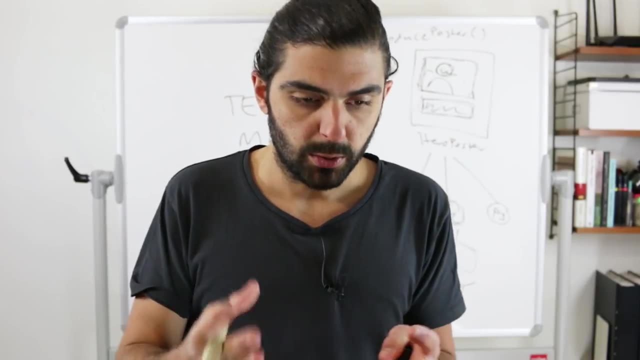 you're starting to see how this works, you might actually already feel that. wait a minute, this sounds like a lot of frameworks. For example, if you're familiar with Ruby on Rails, if you think about active record, the notion that when you're designing something, that's 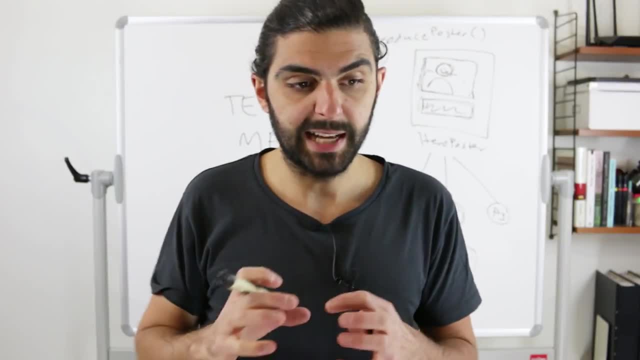 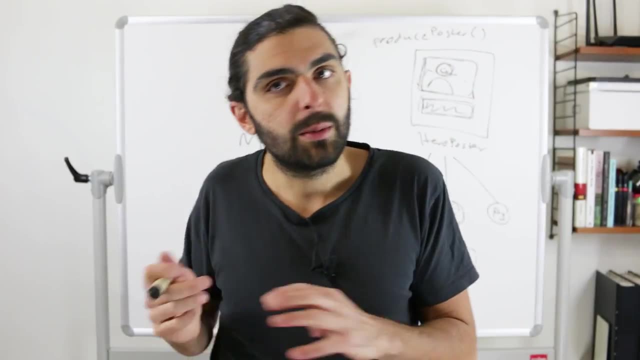 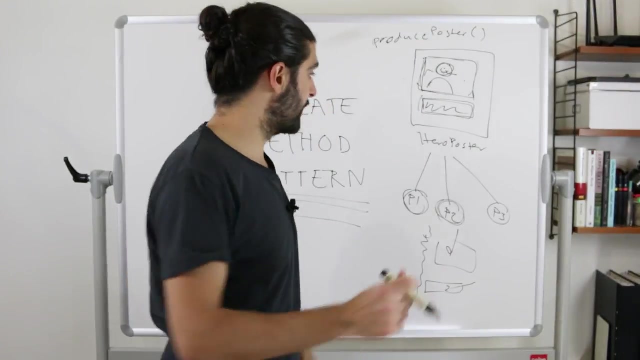 database record you then inherit from active record, and active record does a bunch of database-related things to your object automatically for you, but gives you a number of hooks that you can hook into to add special behavior, right? So we're jumping ahead a little. 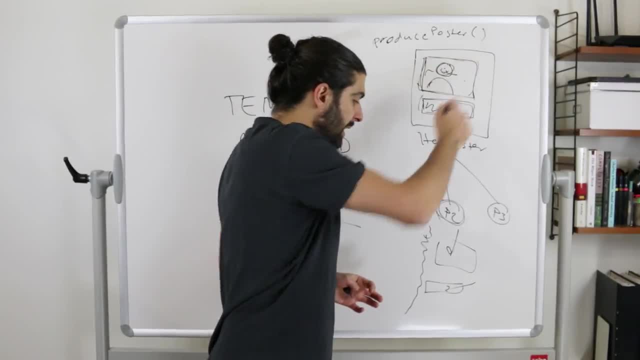 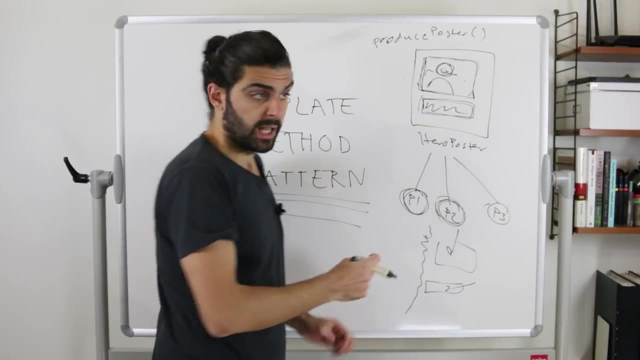 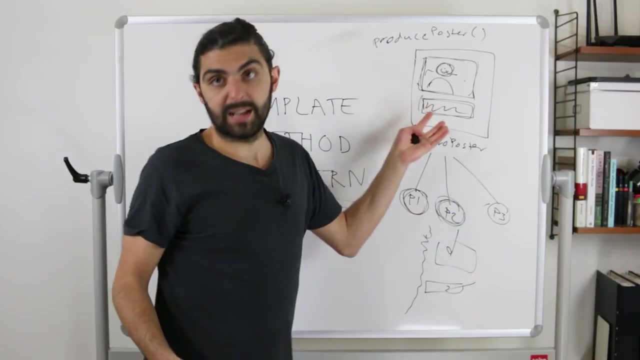 bit, But if this then is active record, then this would be maybe your user and this would be your pollster model and this would be your comment model, Because they have slight nuances but they have ways of hooking into active record, because they are subclasses of active record. But again, 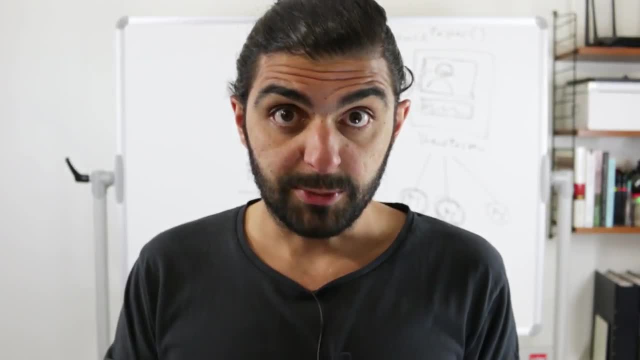 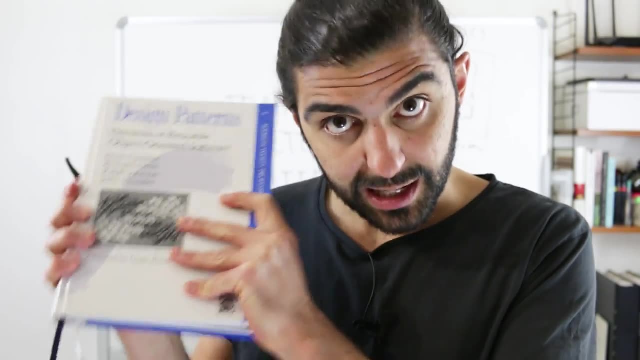 now we're getting ahead of ourselves. so let's look at the definition. So I'll read the definition from this book: Design Patterns- Elements of Reusable Object-Oriented Software by Gang of Four. This is like the classic design patterns book And, by the way, I'd highly recommend that you get this book or this book. 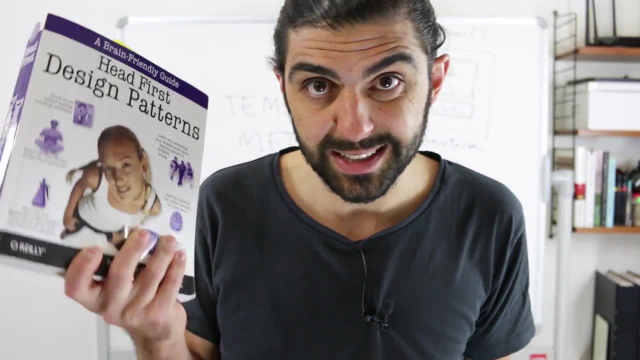 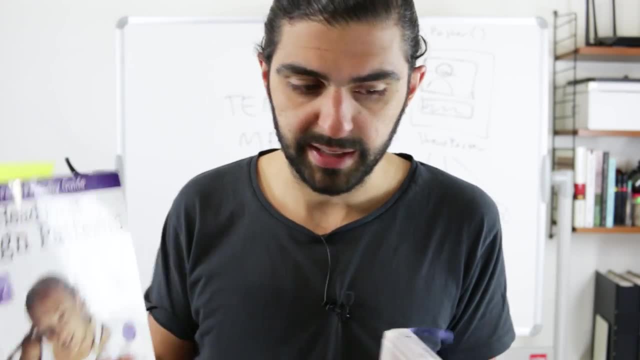 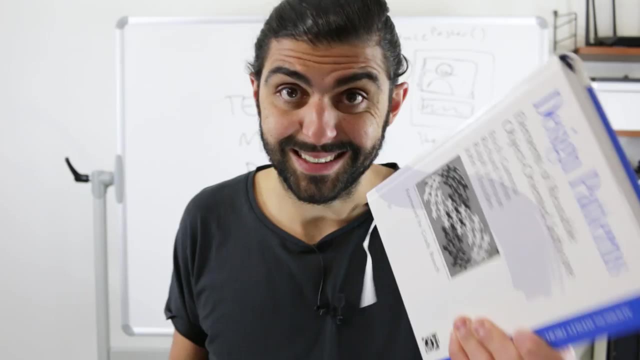 This again is the Gang of Four book and this is headfirst design patterns. So this is slightly simpler because it has more pictures, more jokes, less text and all that stuff. But this is more complete because it touches on more patterns And it's also sort of the- again the classic. 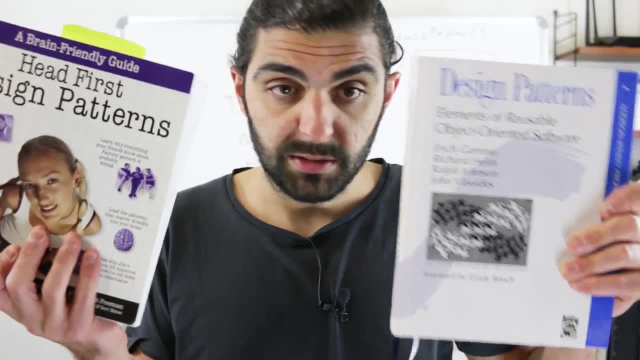 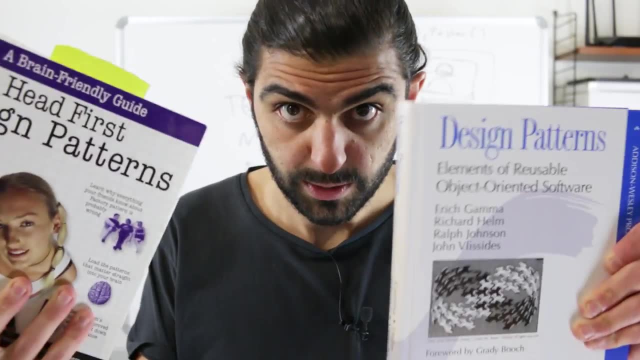 design patterns book, But I'd highly recommend that you get any of these books. Links are in the description. These are affiliate links and they're all in the description, So if you're using these, I get a small kickback. Massively appreciate it. Anyways, links are in the 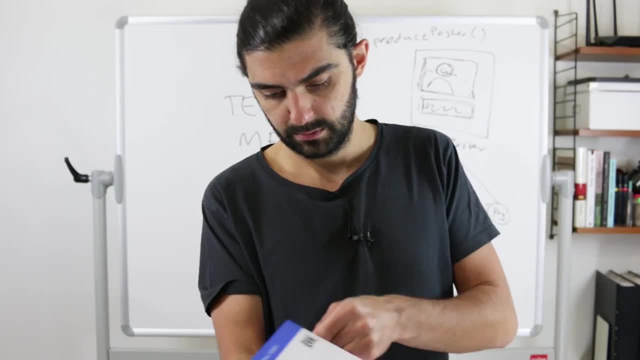 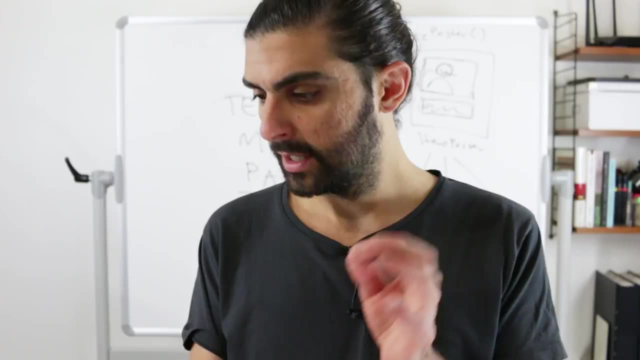 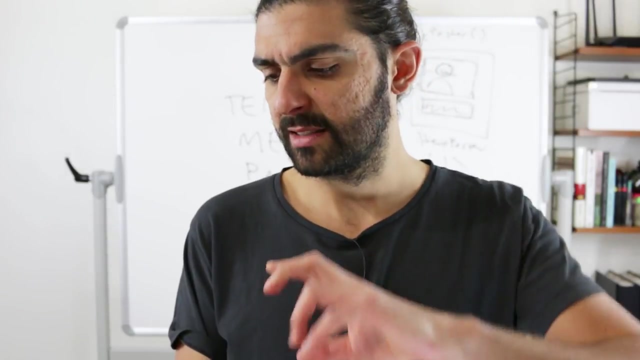 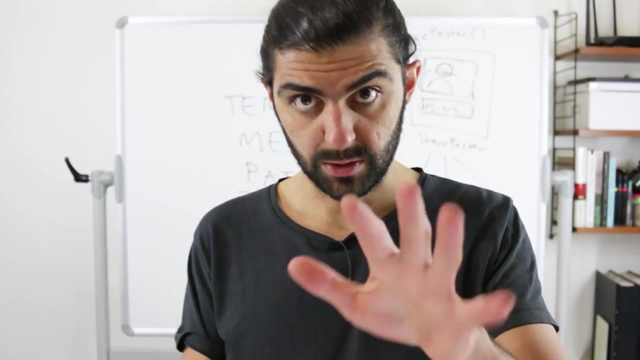 description. Let's move on. So let's read the definition. The template method pattern defines the skeleton of an algorithm in an operation, deferring some steps to subclasses. Template method lets subclasses redefine certain steps of an algorithm without changing the algorithm structure. So I mean, hopefully. 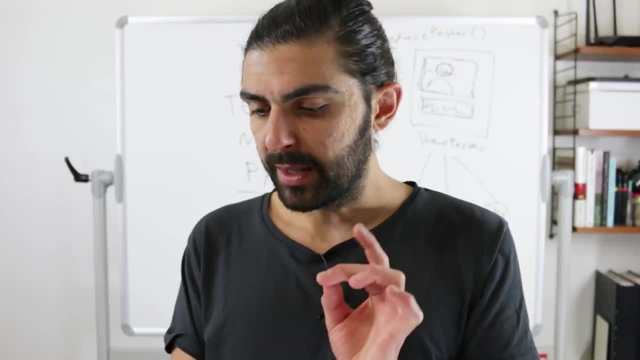 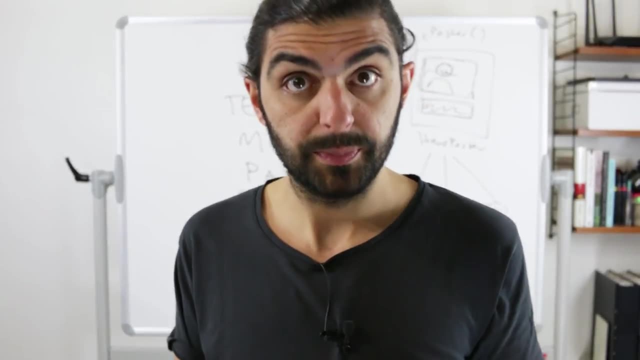 that sounds a bit familiar from what we were talking about before. Think about it: Template method defines the skeleton of an algorithm in an operation. I don't know why they say in an operation. Let's just say defines the skeleton of an algorithm. So this is what, when we were saying 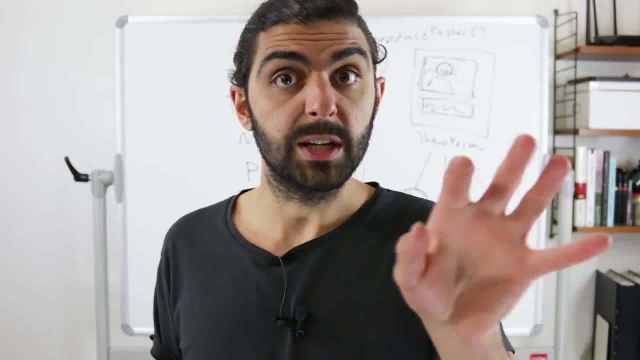 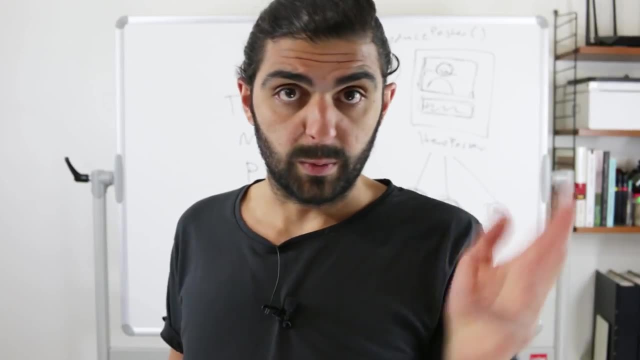 some of the portions of the algorithm might not vary across different specializations. So, whether you have the poster of the politician or the band or the music artist or whatever, some of the portions of that might not vary, such as that you might want to have a picture and that. 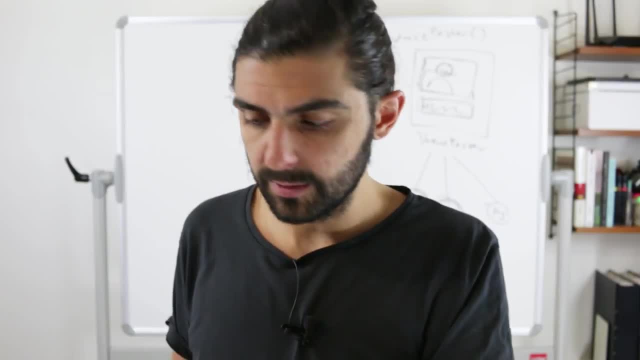 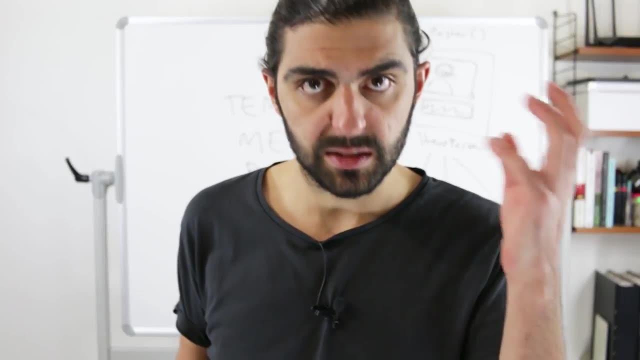 you might want to have a text That might be like invariant, It might be constant, But some steps might vary, And this is what we talked about as well: The actual picture of the politician, which is not the same as the picture of the band. So that's why the second portion of this sentence- 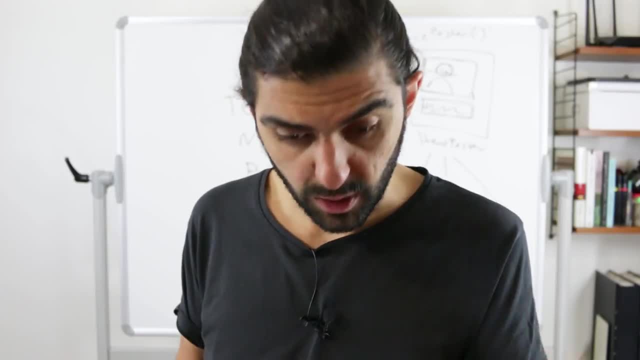 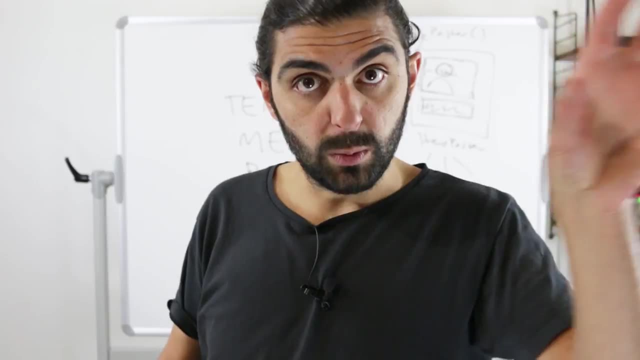 says deferring some steps to subclasses. So what's invariant is in the base class. Invariant means it's always the same. What's invariant is in the base class And what's variant- what varies- is in the subclasses. So there's a subclass for the politician. 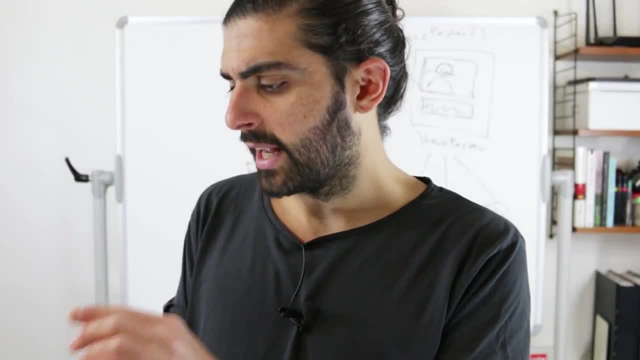 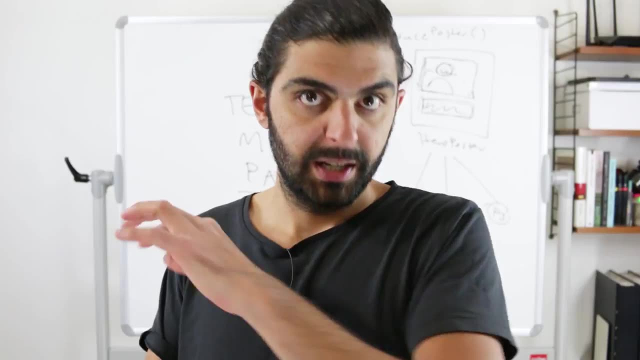 there's a subclass for the band, And then they're sort of just making this clear again. Template method lets subclasses redefine certain steps of an algorithm without changing the algorithm structure. So the point is, the structure is the same all along. So the template method. 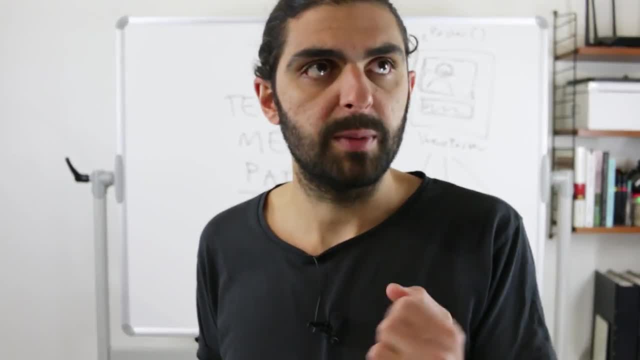 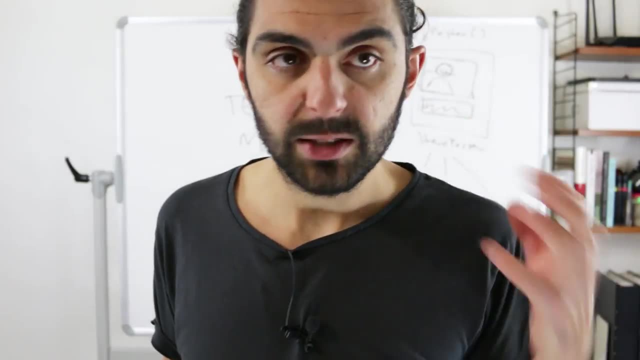 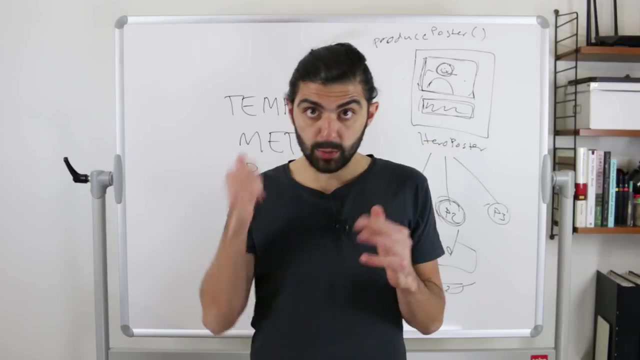 helps you to enforce that structure. I shouldn't say enforce, I should maybe say helps you reuse that structure. helps you reuse that structure across cases, But it gives you a nice way to be able to change what varies from case to case. So that's the definition from this book. So let's look at the UML diagram and then let's talk. 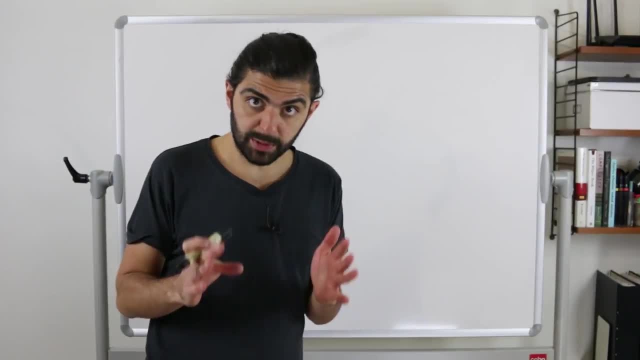 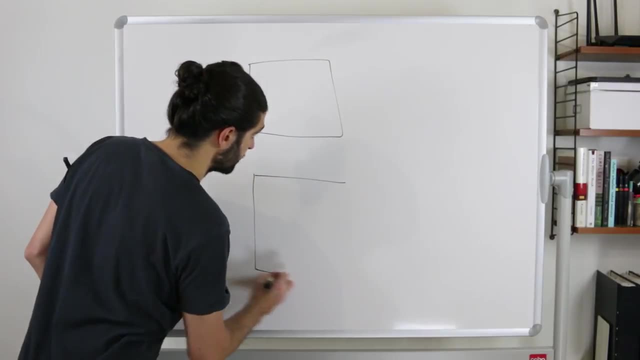 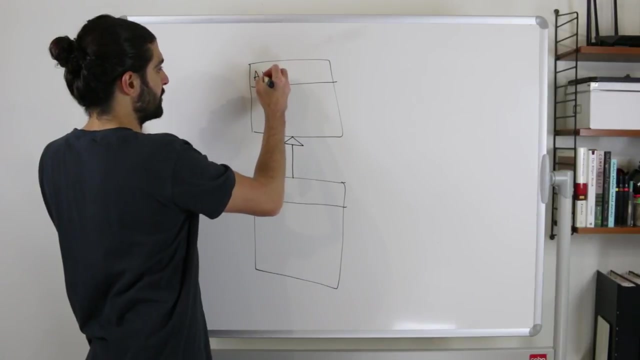 about an example. Let's start by removing this. So the template method pattern is essentially built from two pieces: One abstract class and one concrete class, And then, of course, the concrete class inherits from the abstract class. So let's just write abstract here. abstract class. 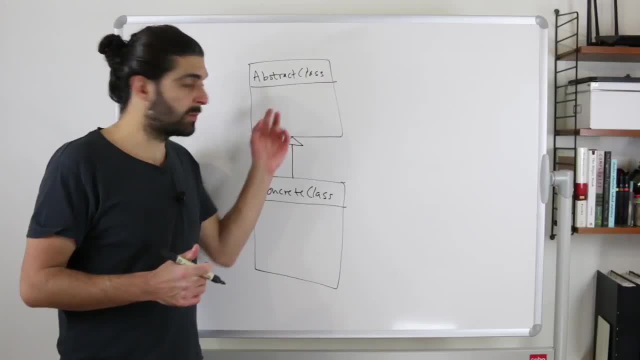 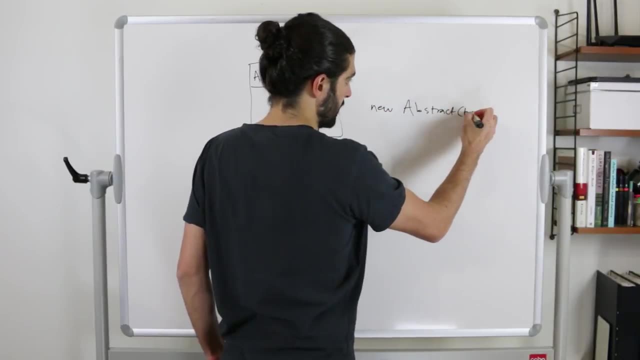 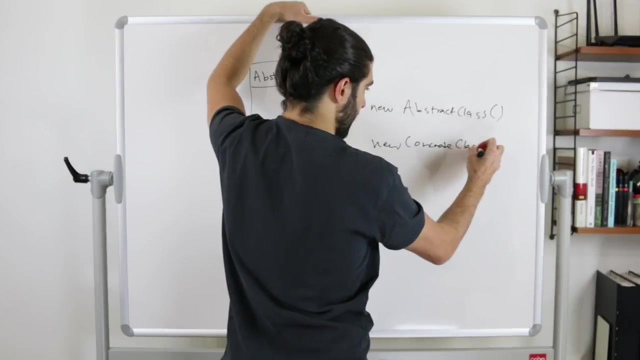 and concrete class here. Okay, And remember: an abstract class is a class that has a concrete class. class is a class that you can't instantiate. so you can never say new abstract class, not valid right, because you can't instantiate this. you have to say new concrete class and this concrete class. 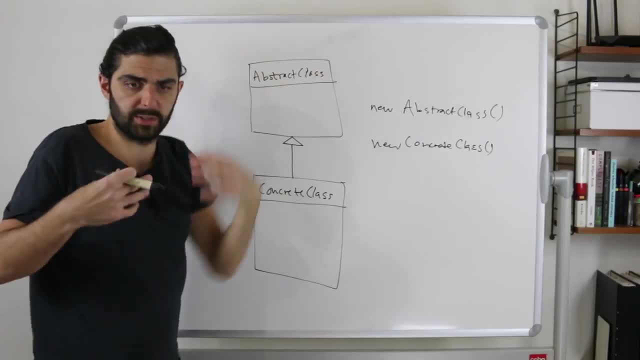 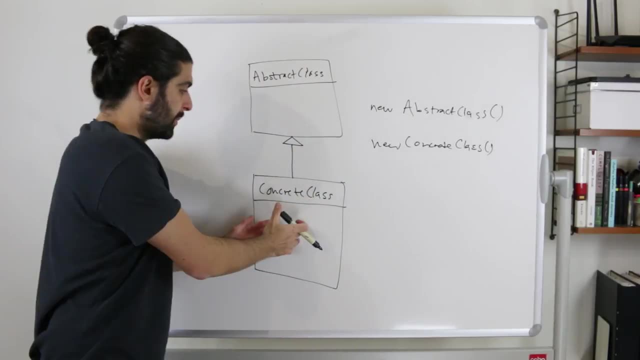 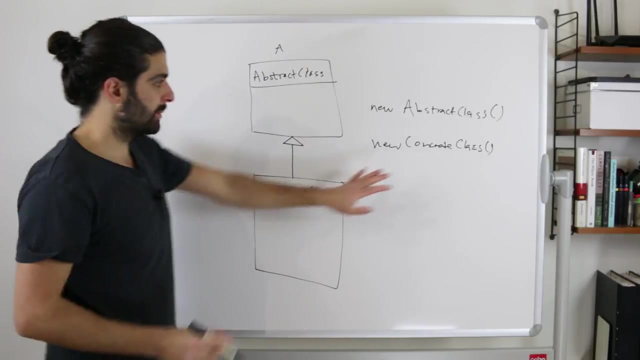 of course, is an abstract class, but it's funny for me to say it is a abstract class, because it's not actually an abstract class in in the sense of the idea of an abstract class, but it is a abstract class in the sense that this is named abstract class. right, if this was named a. what i mean is 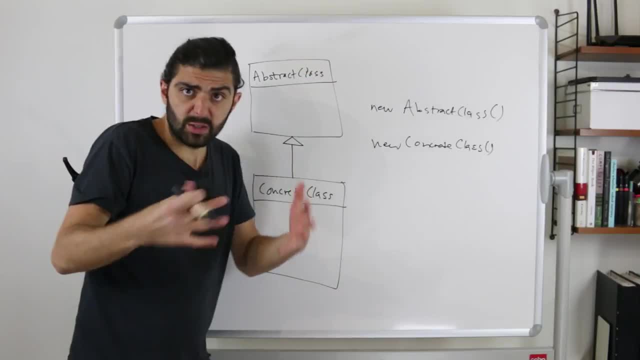 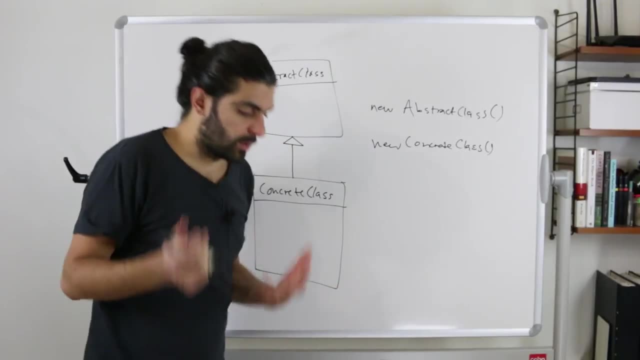 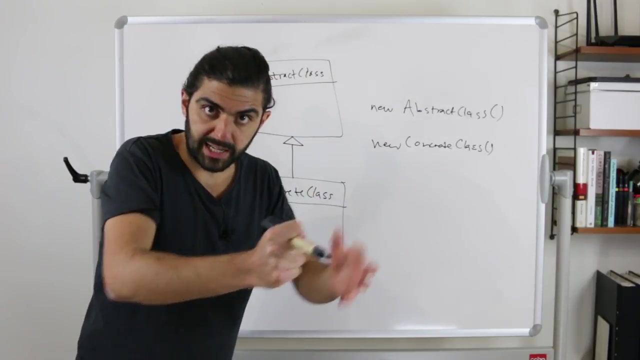 that new concrete class is an, a. so that's the only way to to get hold of an instance of this thing that we that we termed abstract class. but generally, the only way to get an instance of an abstract class is to derive from it, is to subclass from it and then instantiate the subclass any of 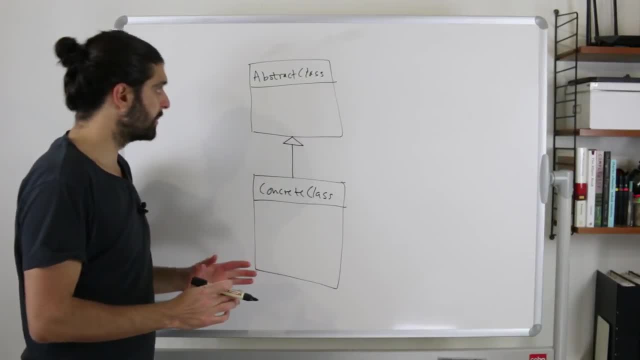 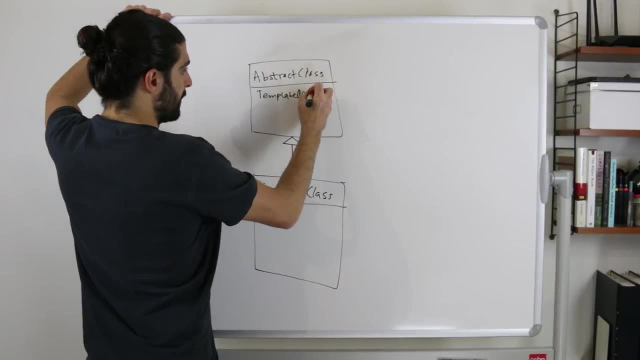 the subclasses. but just a quick reminder back to the template method pattern. what happens next is that you can't instantiate any of the subclasses, but you can't instantiate any of the is that this abstract class has a method that we call template method. sorry, i should learn to use. 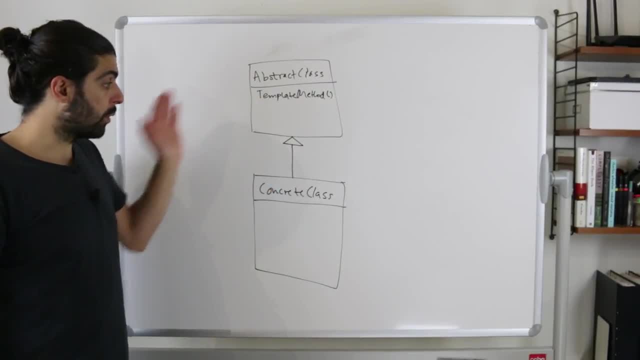 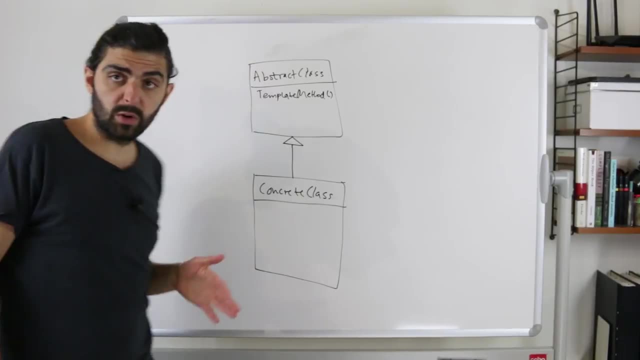 more space on the whiteboard. anyways, the abstract class has a method called template method and clearly the name of this method could be anything that you like, as well as, of course, that the name of the abstract class and the name of the concrete class could be anything that you like, i mean. 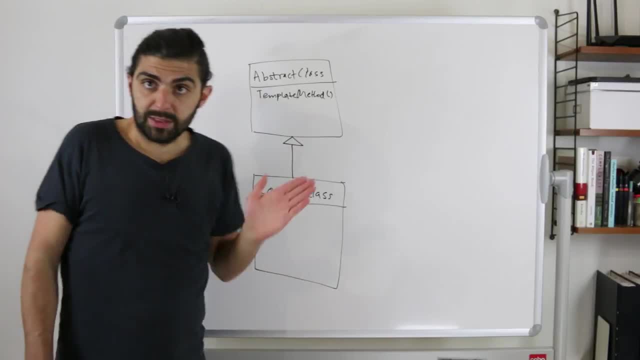 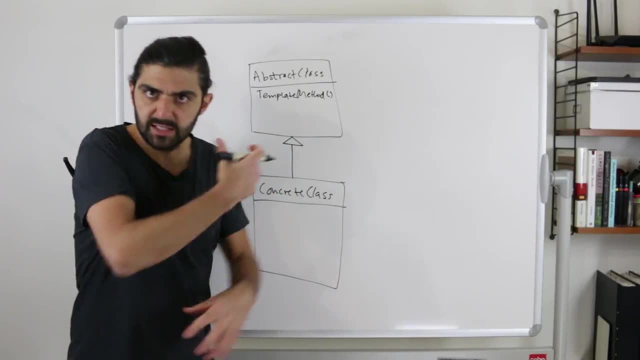 it's completely dependent on your scenario, but we're naming a template method here to to denote or to indicate that this is the method from which the name template method is derived. this is sort of the heart of this pattern. this method, this method is the method that we're trying. 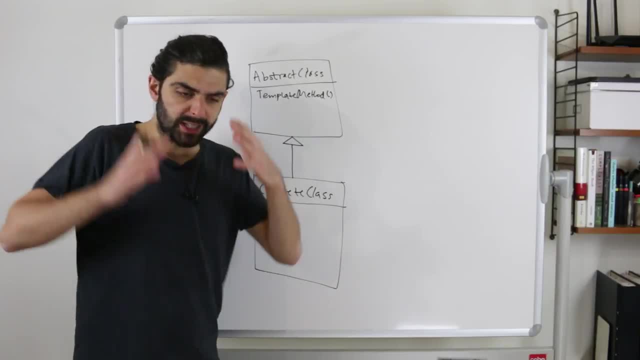 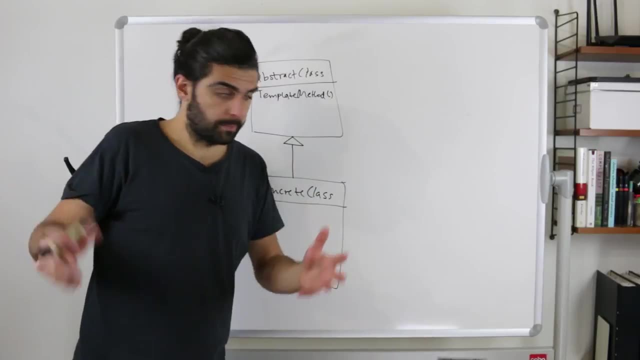 to turn into a template that can be reused. we're trying to turn this method into a template that subclasses can hook into and alter particular pieces of. by the way, quick side note, i believe, if i'm not mistaken, that this is a example of how you could implement the notion of the open. 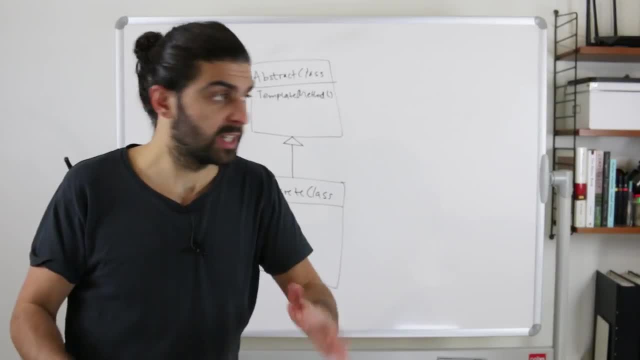 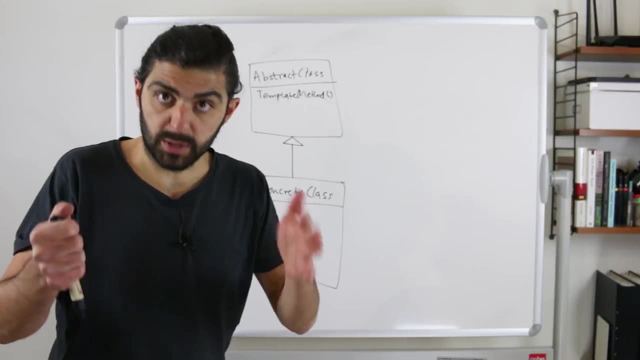 closed principle. the open- closed principle is from the solid principles. check out the links in the description for for more videos on the solid principles, the solid design principles for object-oriented programming. but the open- closed principle essentially states that you should be open for extension but closed for modification. in other 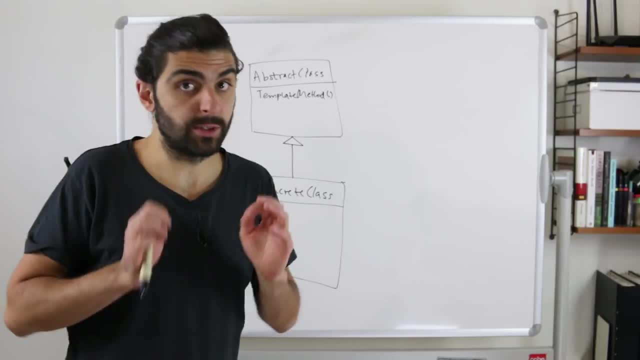 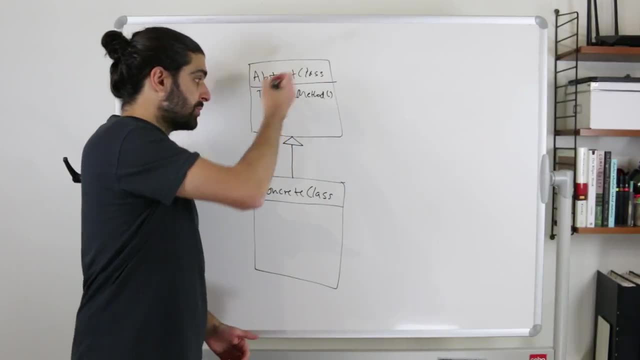 words. behavior should be able to be changed without having to change the source code, and this is one way of doing that. so the template method pattern allows you to change the behavior of this abstract class by introducing new concrete classes. so open, close principle tends to be one of these. 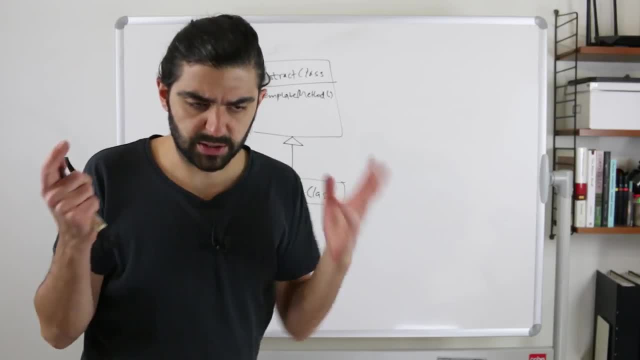 principles that's easy to understand in theory, but then, like when you're actually trying to apply it, you're like: but how in the world can you apply it in a way that's easy to understand in theory, but then, like, when you're actually trying to apply it, you're like: but how in the world? 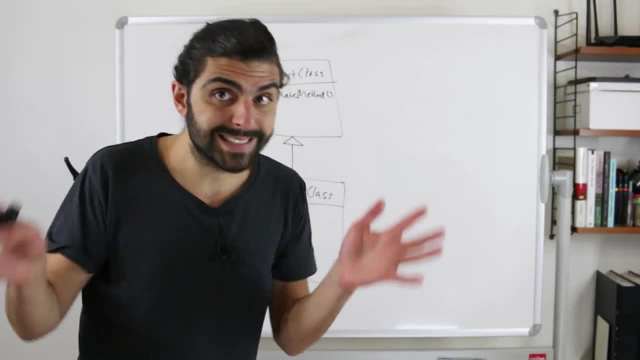 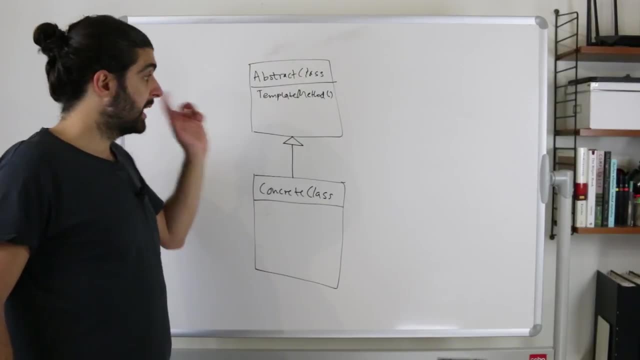 would this work? but then you can think about the template method pattern as one example of how this could work. anyways, end of side note. so the template method is only piece number one from from this pattern. piece number two is that the abstract class then introduces a number of operations. what? 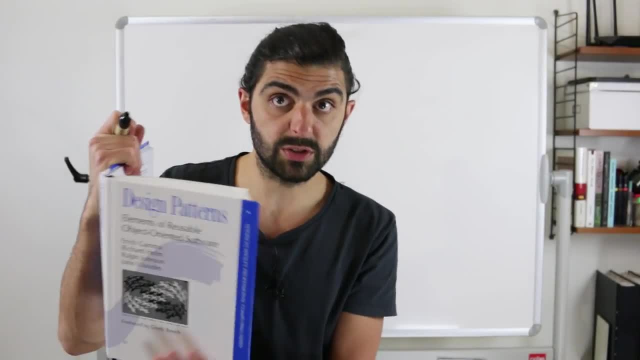 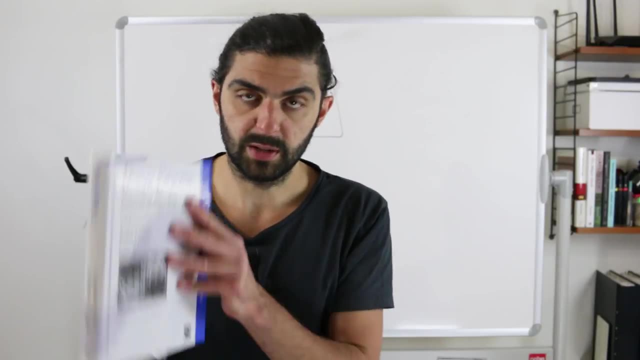 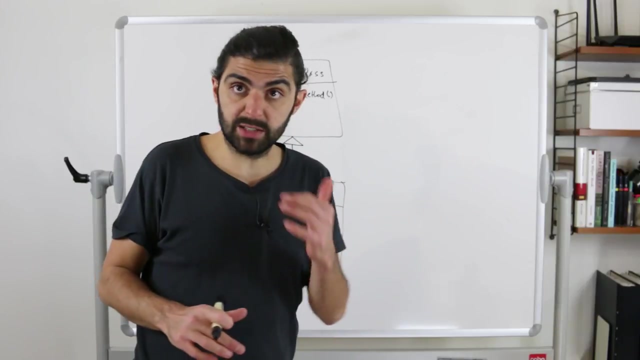 in this book are called either primitive operations or hook operations. they have a few other types of operations mentioned in this book as well, but for more information about that, see the book. but primitive operations are essentially abstract operations and, to make our life simple, let's simply mention two operations and let's call them operation one and operation two. 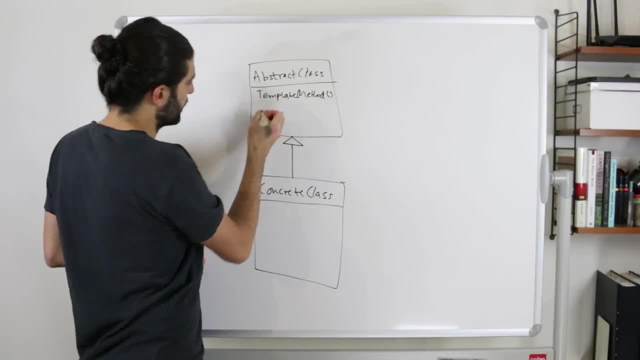 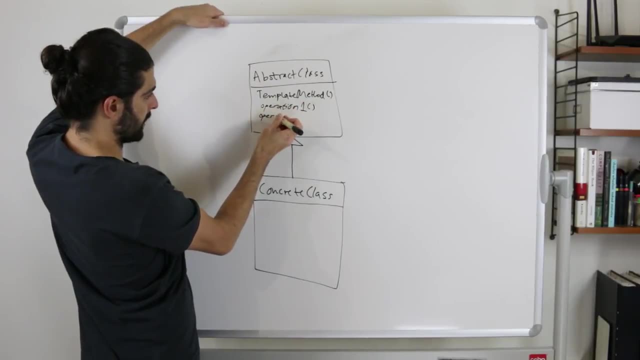 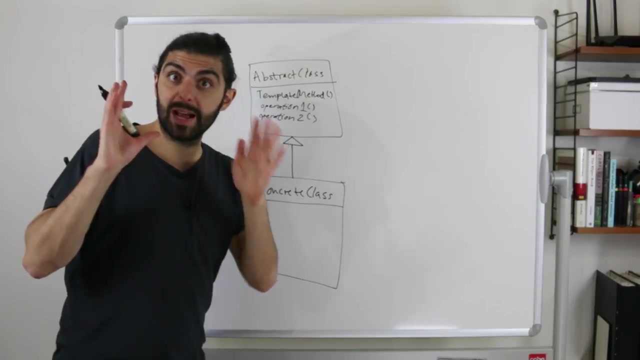 and since these are abstract, let me sort of try to write this in italics. so we write operation one and then operation two. yeah, so i guess italics was never meant to do in handwriting. anyways, i tried to use italics to denote that these are abstract methods. so, if you think about it, ten: 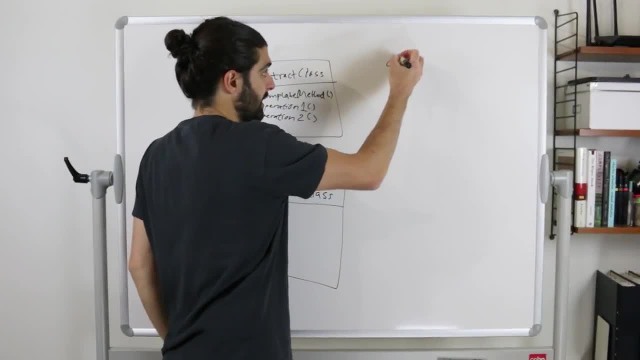 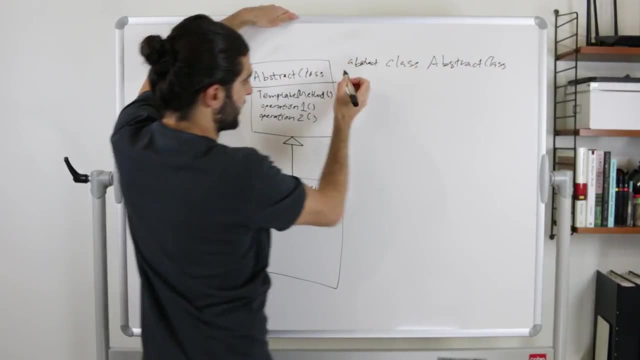 to the method in this class, right, when actually writing out this class, right, like saying class, abstract, class or sorry. actually i need to use the word abstract here to know that there's an abstract class. now we're trying to like pseudocode, right, there's an abstract class named abstract. 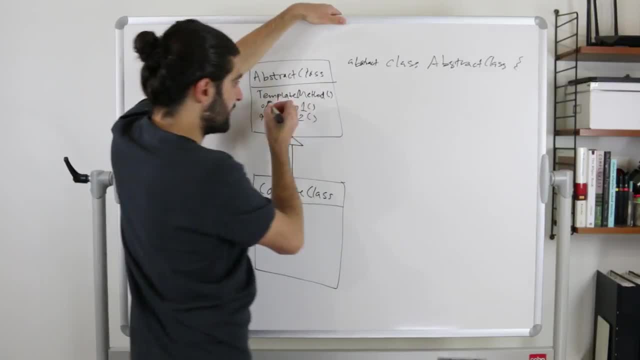 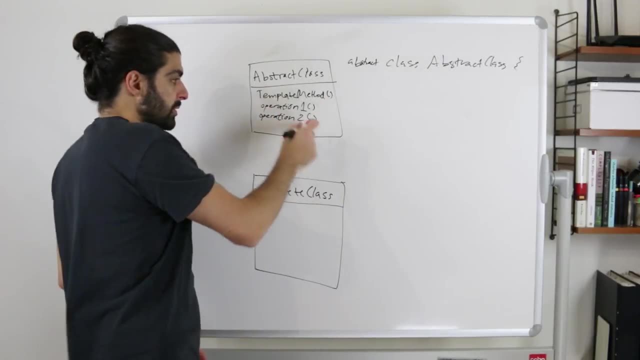 class and here's its implementation, and then i would write the method, template method. right, then i would actually supply an implementation for template method, but operation one i would not supply an implementation for and operation two i would not supply an implementation for. instead i I would denote them as abstract. 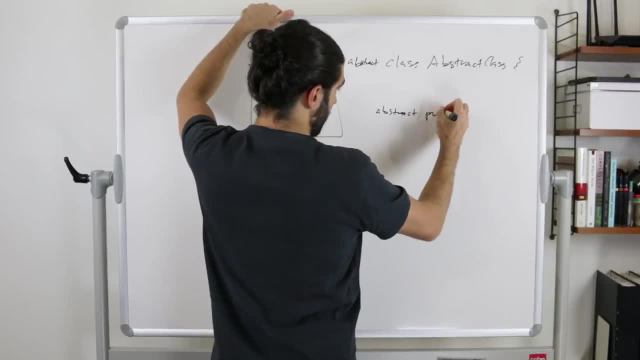 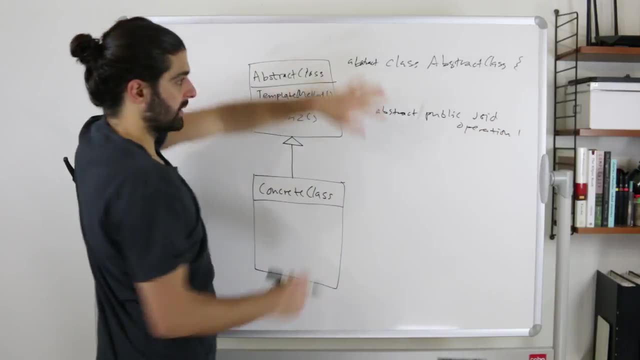 Depending on your language, you might do this something like abstract, public, maybe void- I guess this is a void method- and then operation, operation one, et cetera, et cetera, I mean. but that depends on your language. 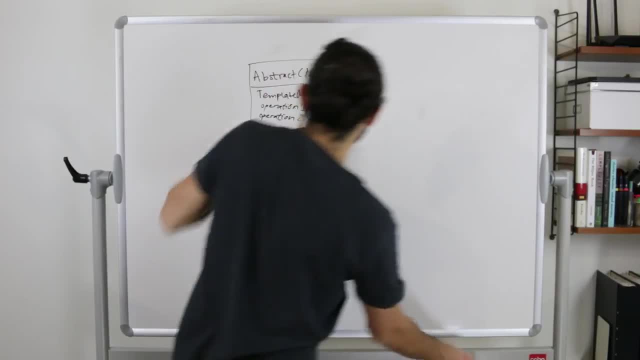 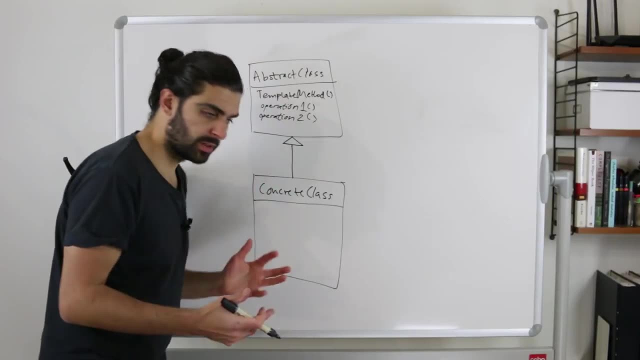 how you would actually write that. But essentially, when defining that class, you would simply state that there exists a method called operation one, It has a return type, it takes some arguments, but there is no implementation in the abstract class, because this class is an abstract class. 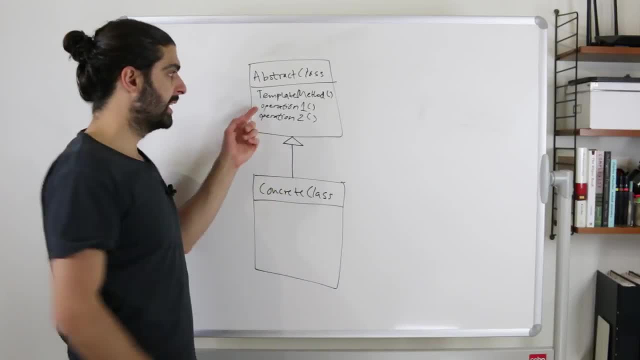 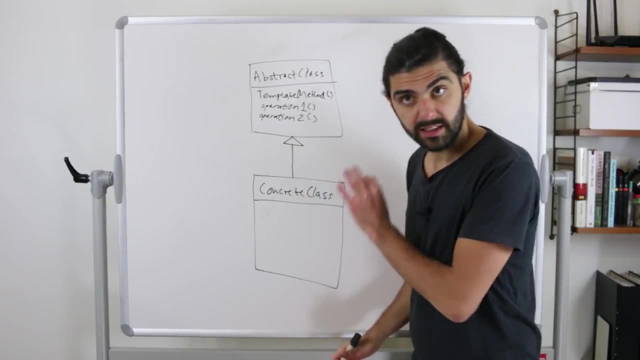 Instead, subtypes necessarily have to define the implementation for that abstract method. But let's move on. What does this then mean for the concrete class? Well, this means that the concrete class has to implement these abstract methods. So we'll state that here. 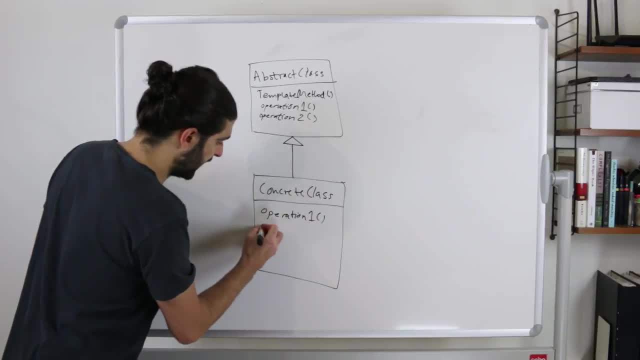 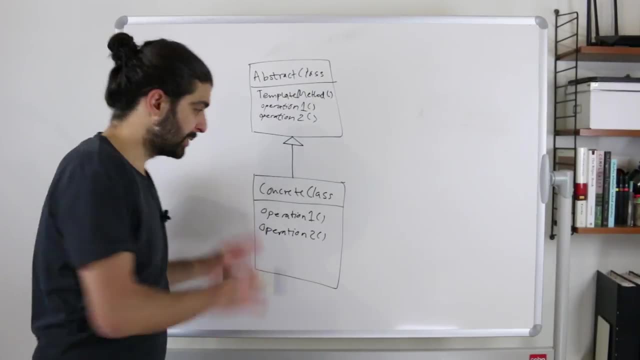 We'll say operation one and operation two. Note that I'm not using italics here. Clearly it's not super obvious that I'm not using italics here, but let me tell you that I'm not trying to use italics here. 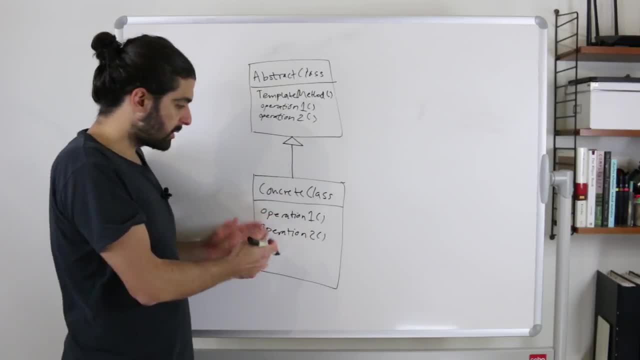 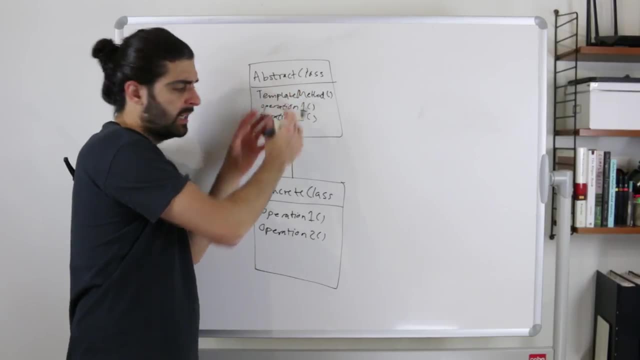 So the point is that the implementation in the concrete class of operation one and operation two is now concrete, whereas in the abstract class it was abstract, meaning it didn't have an implementation here, but here it has an implementation. So what does this mean? 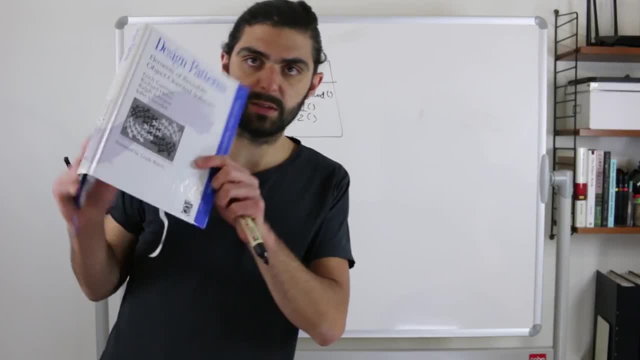 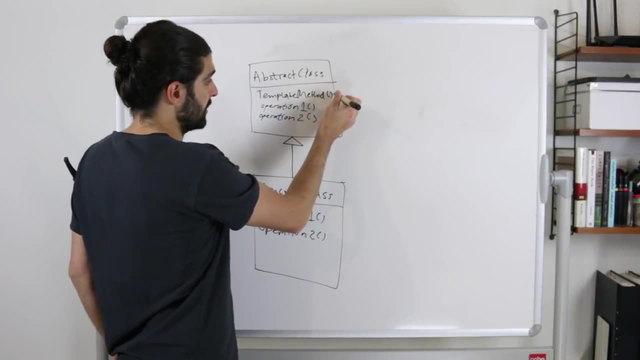 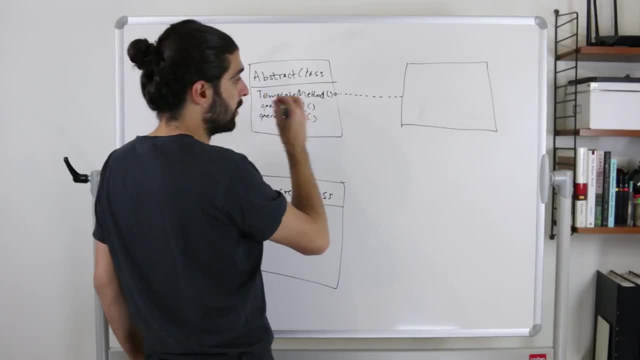 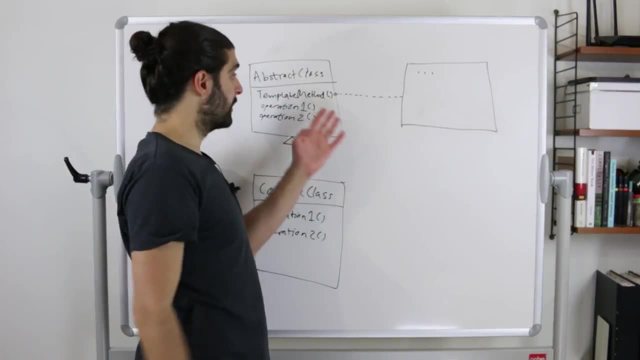 and then they're showing a piece of the implementation of the template method, And what they're saying here is that let me just say dot dot dot. they know that there is some start of the implementation of this template method and then something happens. 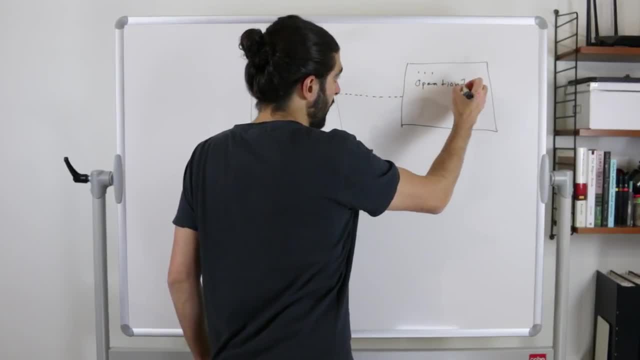 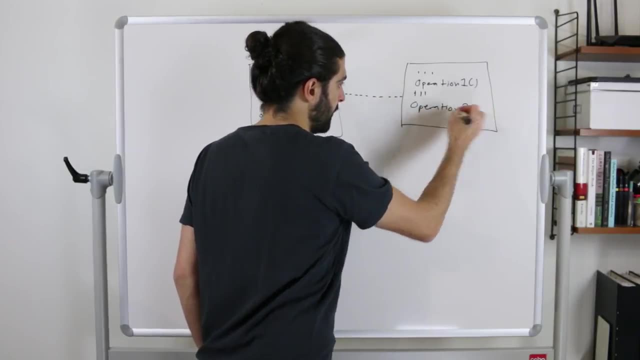 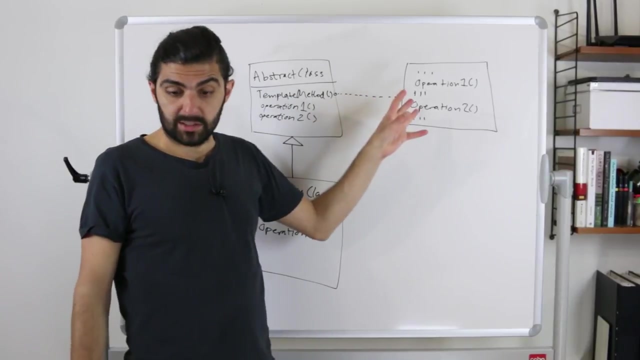 then we call operation one And then there's some more implementation of this method, and then they call operation two, operation two, and then dot dot, dot. there's potentially some more implementation. Now, clearly This is non-exact. They're writing dot dot, dot and operation one, etc. Indicatively. They're trying. 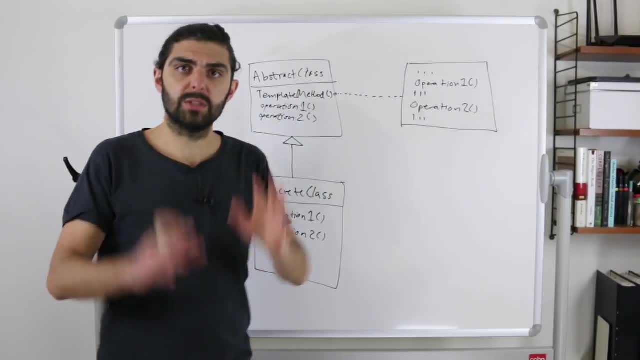 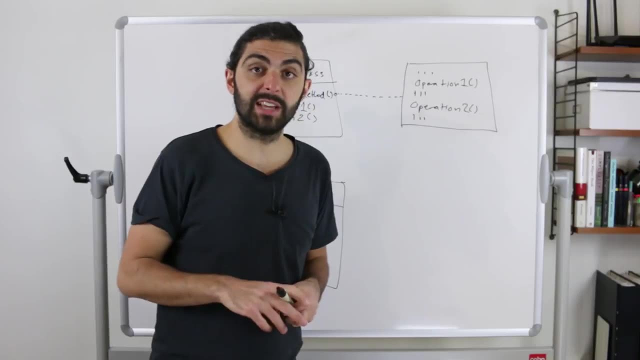 to indicate what the template method does. In other words, what the template method does. let's think about that. What it does is that it has some implementation. There's some algorithm. This is back to the idea of the algorithm. This is the poster producing algorithm. But there are some. 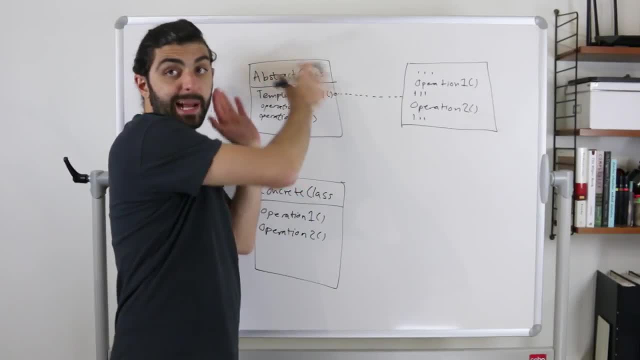 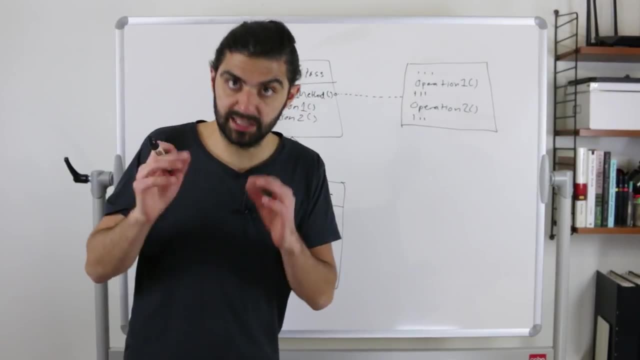 pieces of the algorithm that can't be defined at the abstract class level, And these operations are then deferred to. or let me put it this way: There are some pieces of the template method that can't be specified in the template method on the level of the abstract class, In other words, 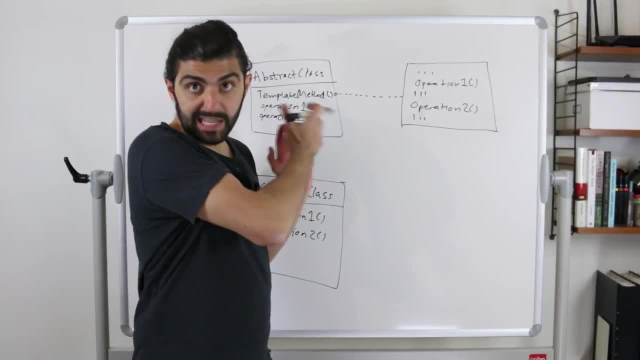 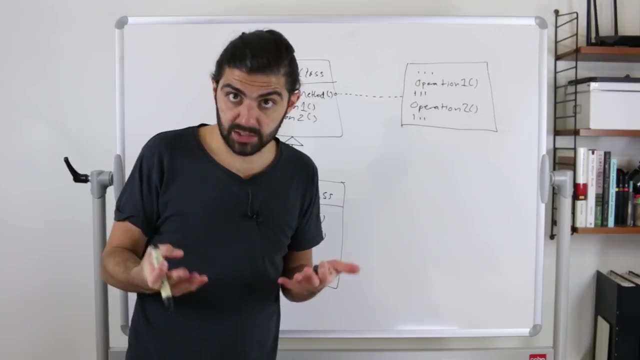 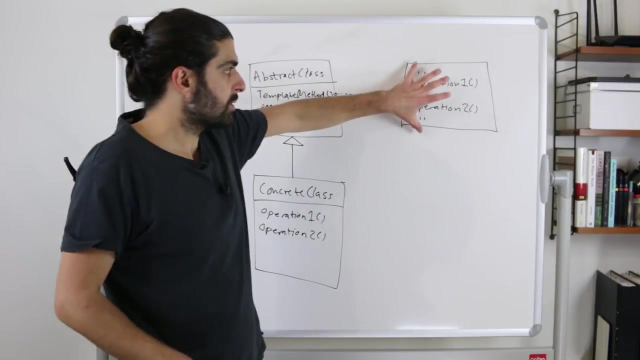 in the general case we can't say what the algorithm does. We can say structurally what the algorithm does. We can say structurally what the algorithm does in the general case, But we cannot say in detail for every step what the algorithm does. So this completely depends. 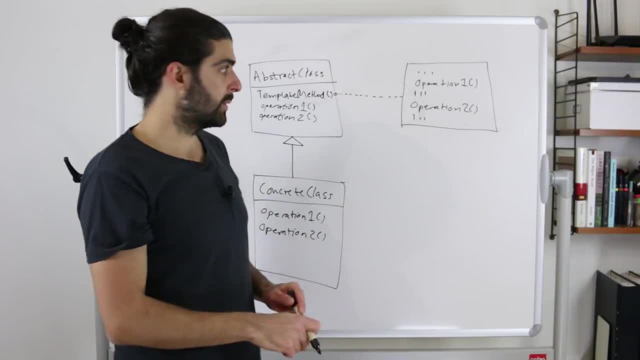 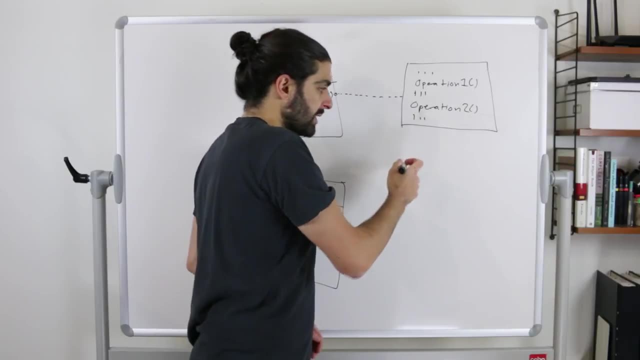 on what algorithm you have. But here, If we think about the poster scenario, it would possibly be like to set the dimensions of the paper, draw some kind of border, set the margins and then create a placeholder for the text and then actually insert the text. And here we delegate to operation one which is maybe to 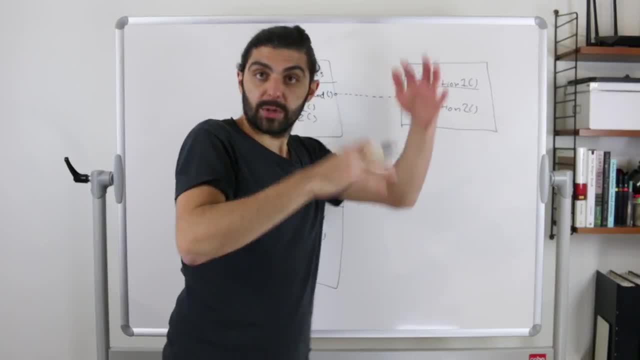 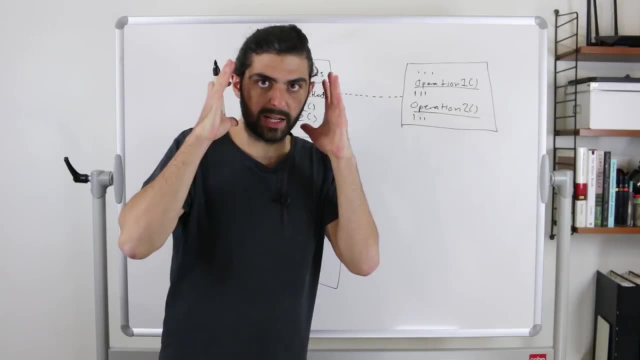 insert the text. Then some more stuff happens. We're constructing more portions of the poster and then we delegate down to operation two. So essentially what we're doing is that we're thinking about our algorithm. We're saying, okay, let's think about our algorithm, What's general? 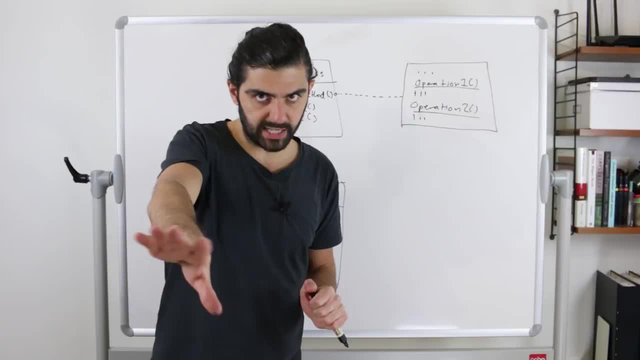 We can directly say: well, let's say t is equal to t, So let's say t is equal to t, which comes down to t. So if we have t at t at t, then if we look at t at t, 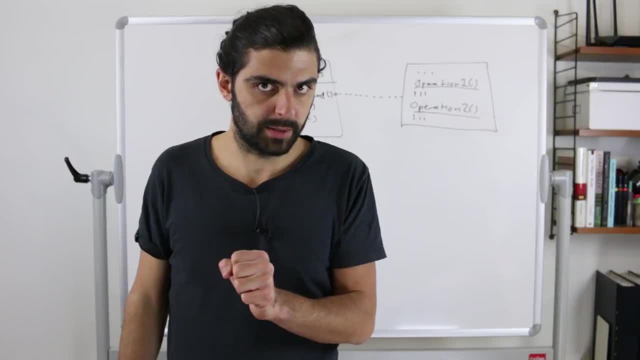 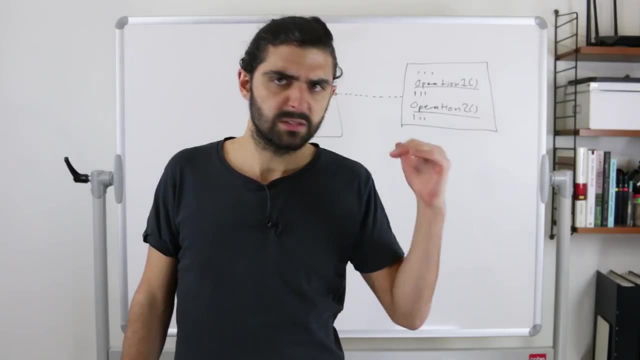 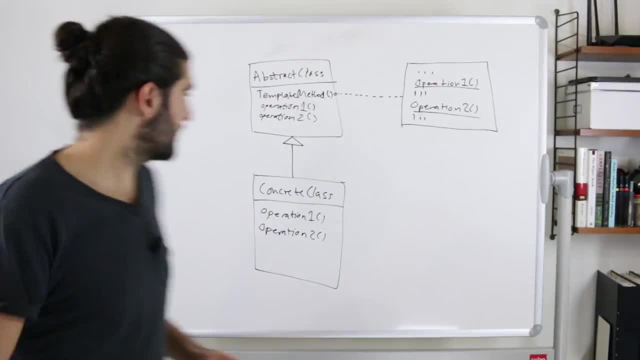 And this is the sameえば we did in the last example. So here we can say that we want to use t at t at t at t. So let's say t is equal to t, t at t, And the algorithm is not going to directly use t at t, at t at t. 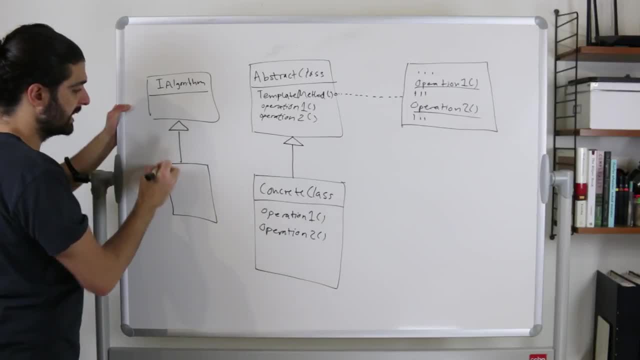 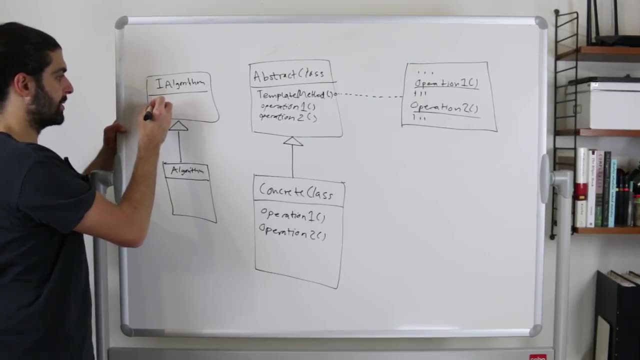 Okay, that's then implemented by. it's an interface, right, it's implemented by some algorithm, and then we have some, some method here. so so let's just- I mean, let's name this algorithm as well, or maybe that would be confusing. so actually is, let's name this operation, operation and then operation. here I just 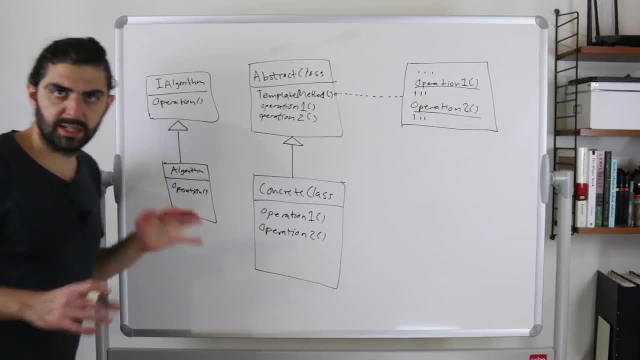 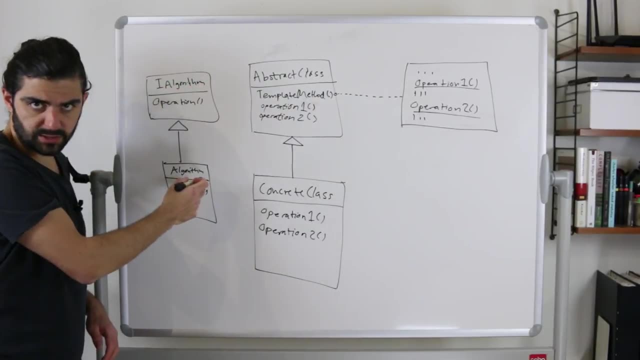 realized actually. I mean I used out I algorithm and algorithm here, but but clearly when we've talked about the strategy pattern or in most of the literature, they actually call this I strategy and then concrete strategy. sorry about that, but I mean doesn't really matter- strategy or algorithm or 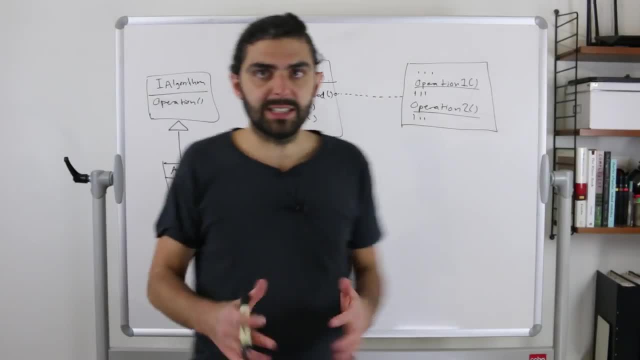 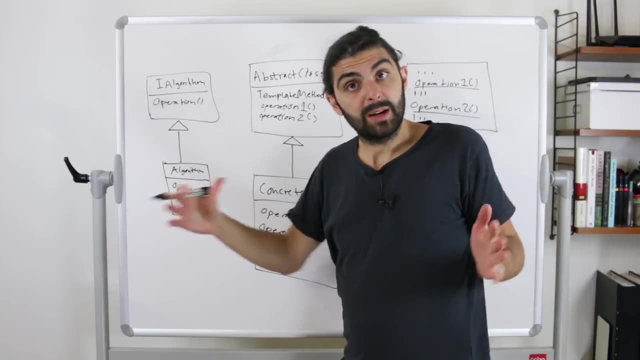 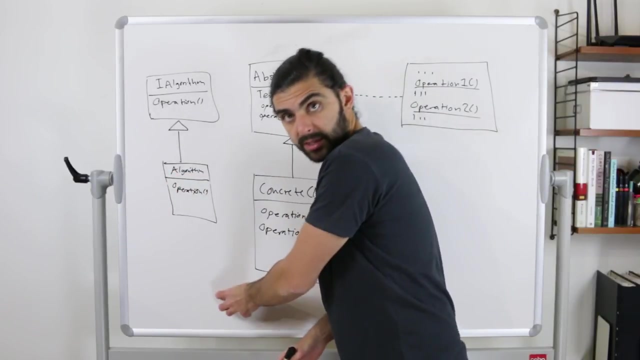 whatever. the point is that the strategy pattern. what it does right is it defines a family of algorithms, it defines an interface that can be used across the whole family of algorithms, and then you define concrete algorithms so you can have algorithm a, algorithm B, algorithm C, algorithm D, etc. and they all implement. 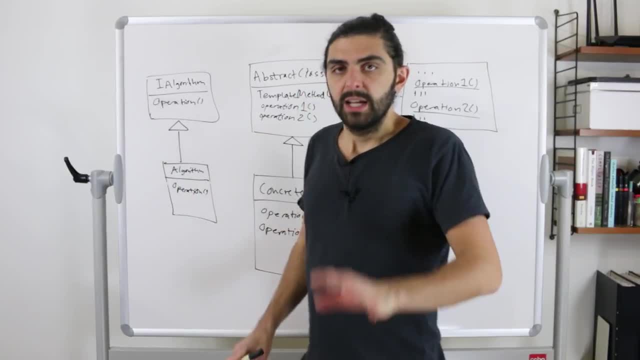 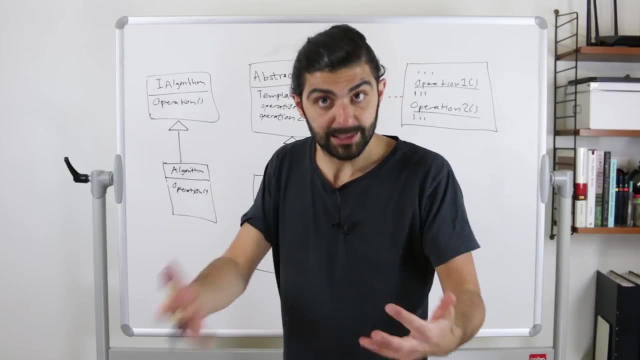 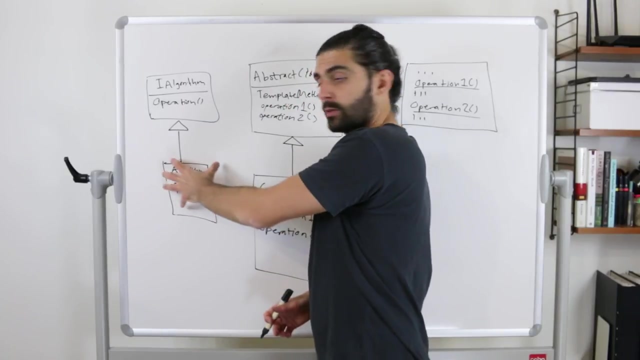 the interface I algorithm, which means they can be used interchangeably. now the point, or let's say, the massive power of strategy pattern or generally, I mean, if you think about it, dependency injection, the massive power of that is that you have superb composability, because everything, every algorithm, every strategy, does a single thing. there's one. 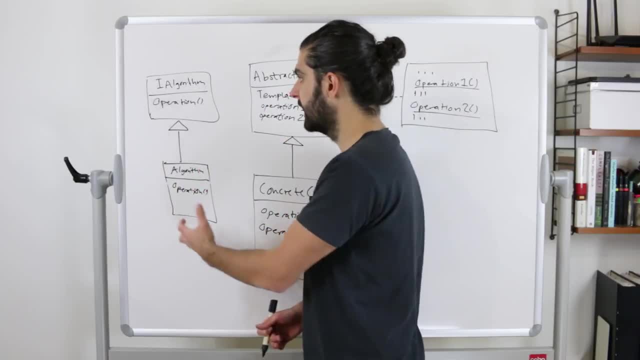 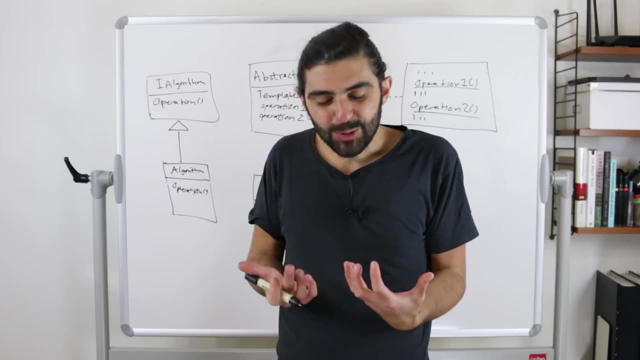 method and that's what it does. that's a concrete implementation of that, and then it follows its, its interface, and this interface also specifies the need for a single method. so there are very, very few assumptions about the future, whereas in the template method pattern, if you think about it, 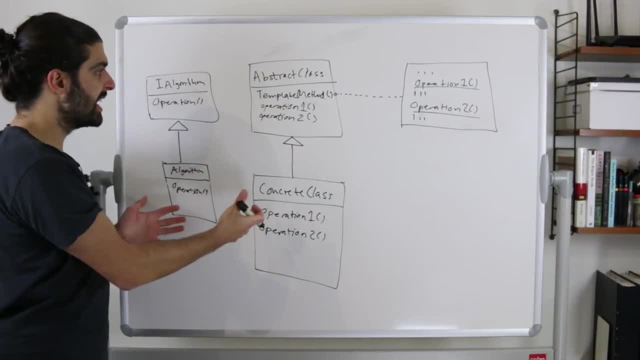 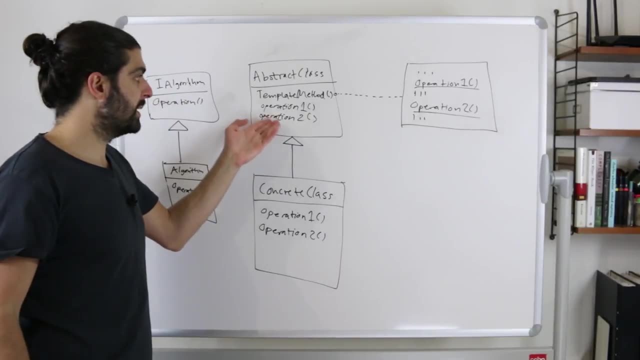 actually this is why I brought this up right, because these look essentially the same, except that here. okay, yeah, here we introduced operation one and operation two, but but actually I mean, it could be, could be that we have only a single operation one here. so if we had only two- template method and the operation one, 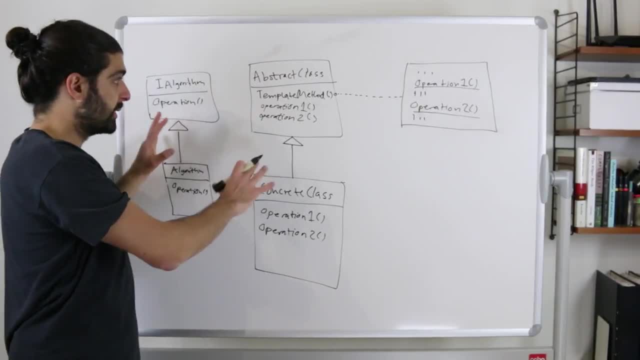 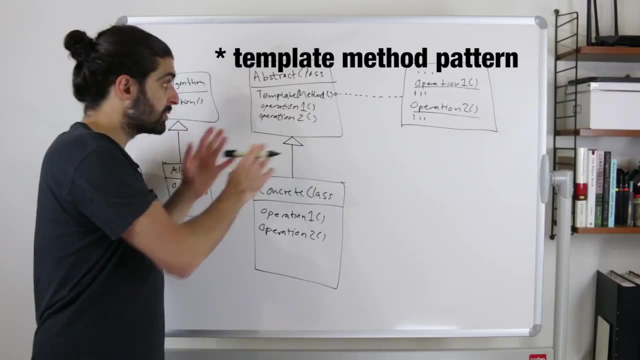 and then operation one here in the concrete class, then the only difference between these two would be the template method. but that's the crucial difference, right? the crucial difference between these two cases is that in the abstract method pattern we also have a template method in the abstract class. 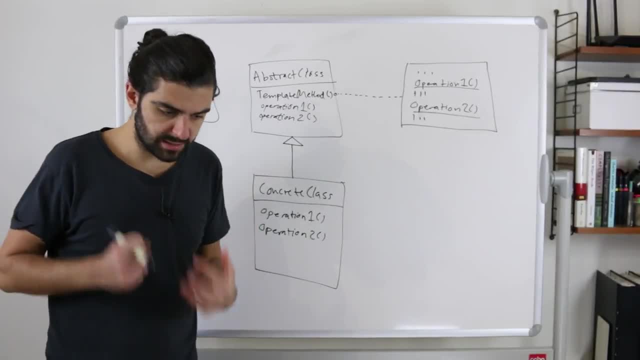 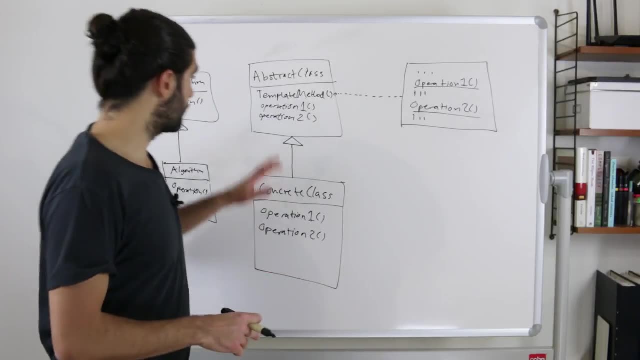 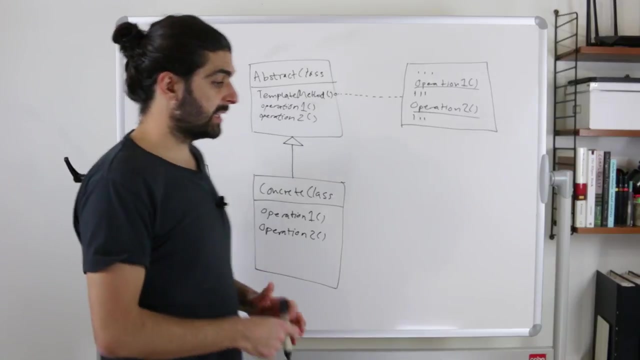 so we are making an assumption about the future. we are making an assumption about how the structure of the algorithm will remain invariant over time. now, clearly, we could of course redefine the template method in the concrete class. that subclass is from the abstract class and actually I mean, I think, in the in. 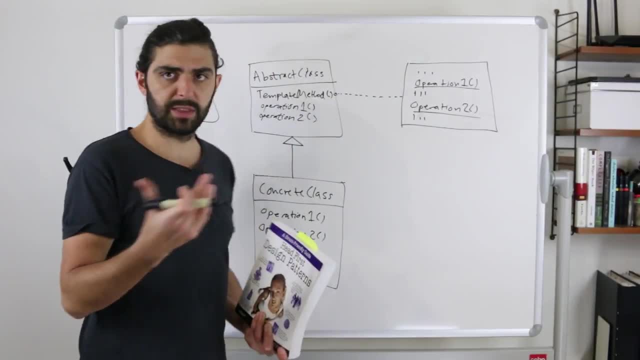 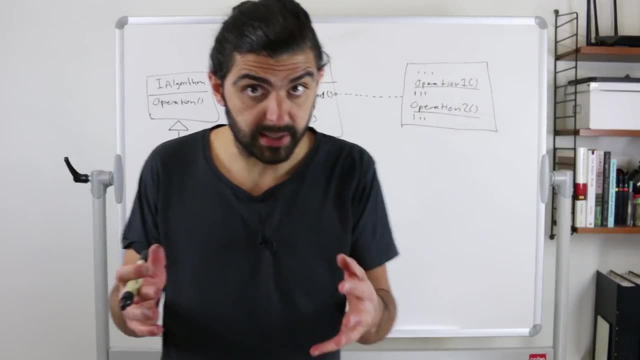 the head first book, they actually suggest that you mark the template method as final as so as to restrict sub classes from being able to change the implementation of the template method. I wouldn't necessarily say that that's a good idea. otherwise, you could, of course, change the implementation of the template method and I wouldn't necessarily say that that's a good idea. 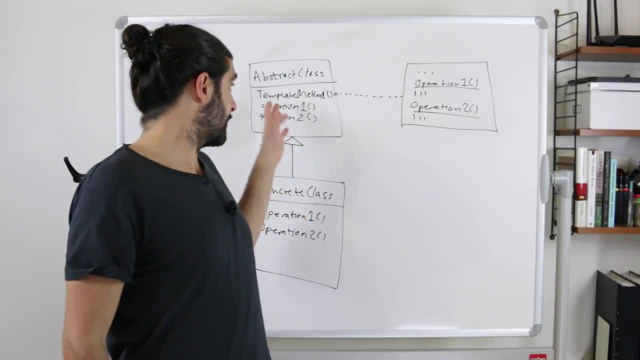 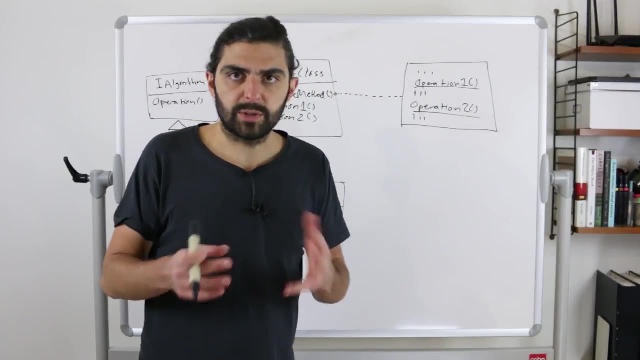 as subjectively But clearly. I mean, if the idea is for the template method to actually remain truly invariant, then that's a good idea. But you know that just to me seems unnecessarily strange and dangerous. But back to the topic here. So we are making the assumption that the template 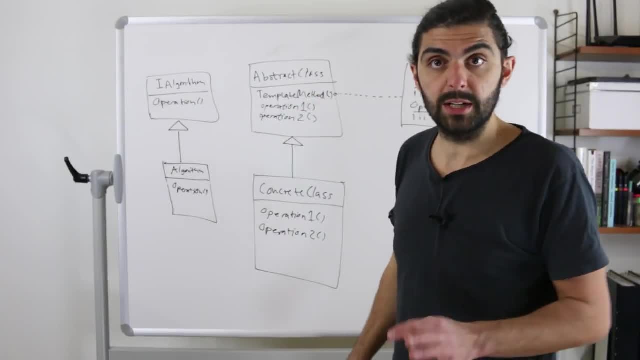 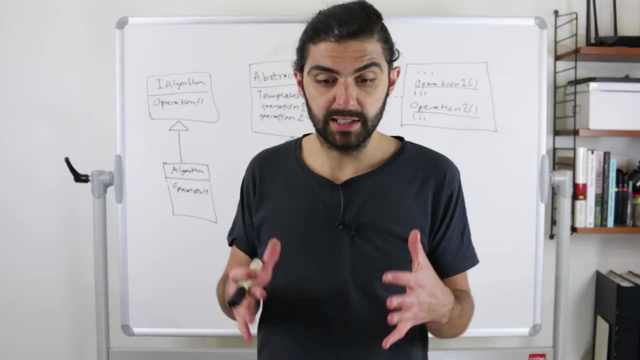 method will remain invariant, The structure of the algorithm will remain invariant And of course, I mean, in some cases we might actually know that And this is why many sources, when you read about this pattern, mention that this is a common pattern in frameworks, Because there it might. 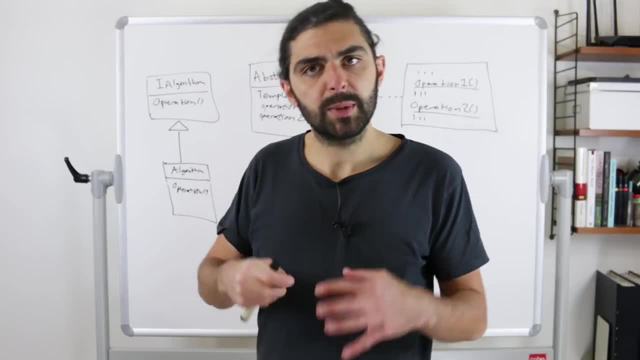 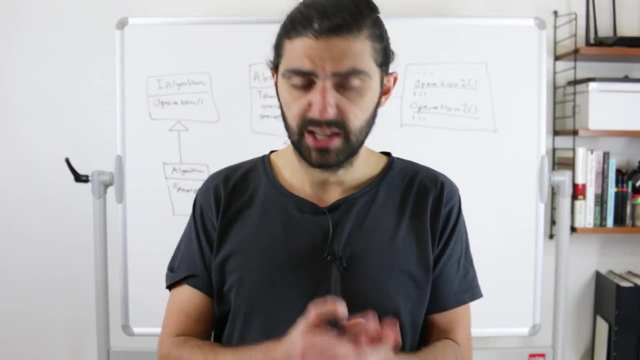 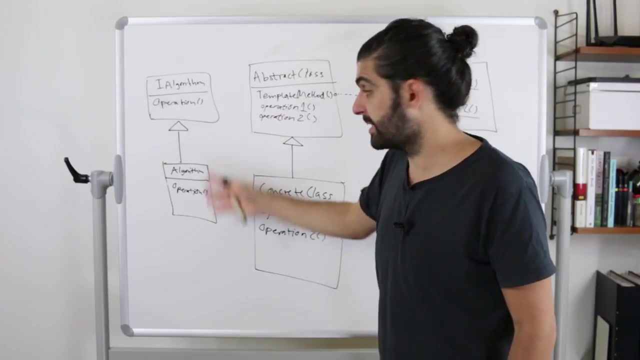 actually make sense to assume that the structure will remain invariant because you don't want to change the interface as users are using your framework. But from my perspective I would caution you to think about whether your scenario is actually truly applicable for template method pattern before sort of jumping into it, Because we can achieve a lot with simply strategy pattern. 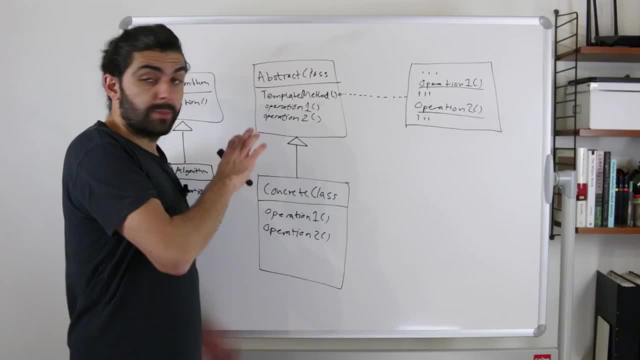 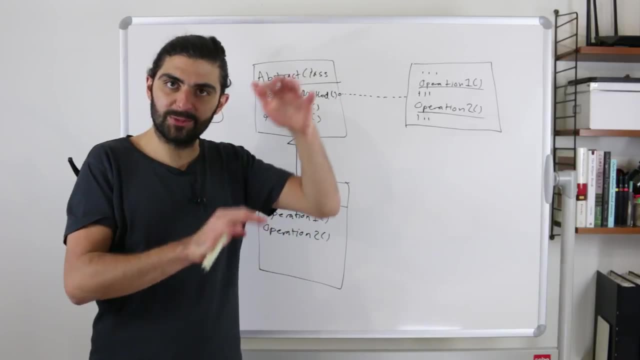 alone. I mean, if you think about it, what we're saying here is because, if you think about it, I mean in the template method pattern, we actually want to be able to compose different pieces to together, But we want them to happen in a particular order, right? So we want this thing to happen. 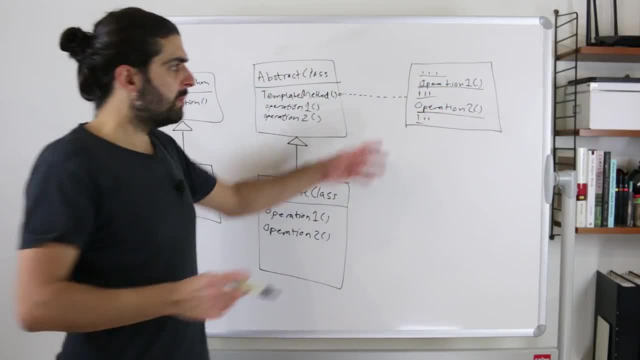 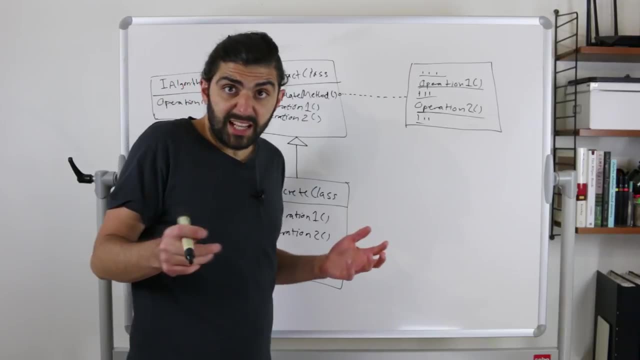 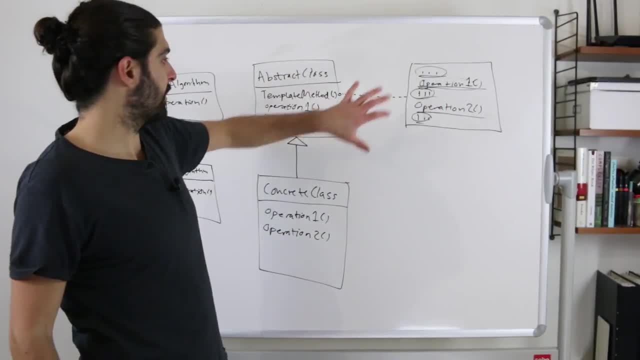 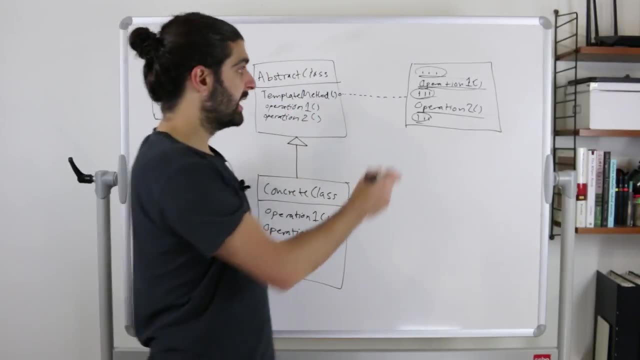 piece is invariant. and this piece is invariant Because I mean, if you think about it, that's what we're doing in the template method pattern. We're saying that all specializations of this particular piece are invariant. So we want to first do this thing, then do something that varies, and then do 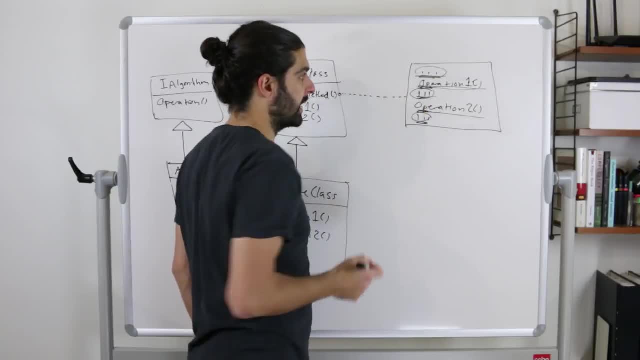 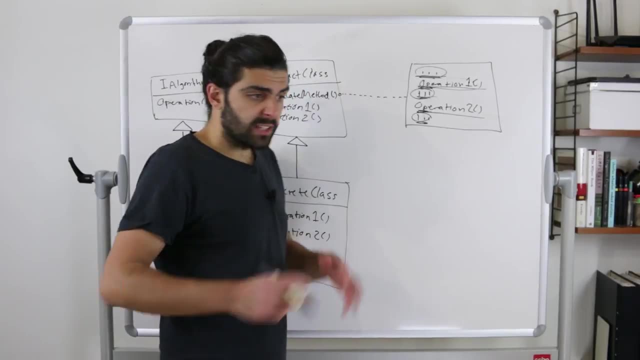 this thing and then do this thing. that varies and then do this thing right. But I mean, how would we, how can we be super certain that that's actually the case? If we're not super certain that that's the case, just use normal dependency injection, right, And this is a strategy. So 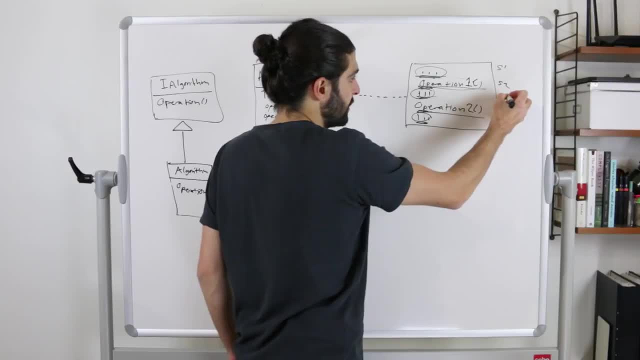 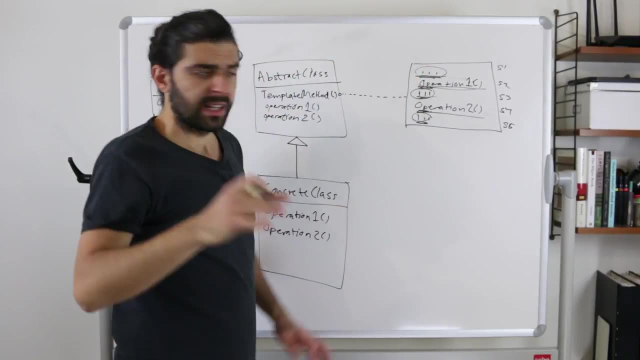 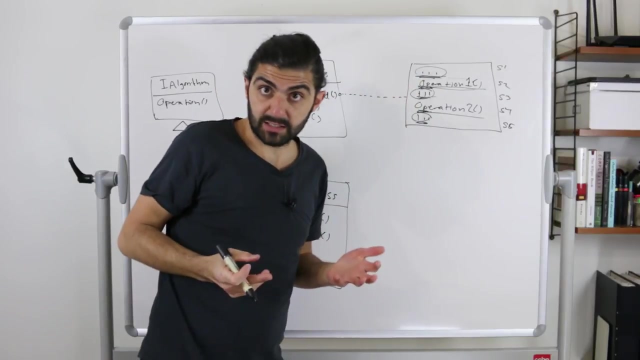 strategy placeholder one, strategy placeholder two, strategy placeholder three, four and five, And then you inject these five strategies and then you run this algorithm. Clearly still, the algorithm would be fixed, The order in which these strategies are executed. that would be fixed. 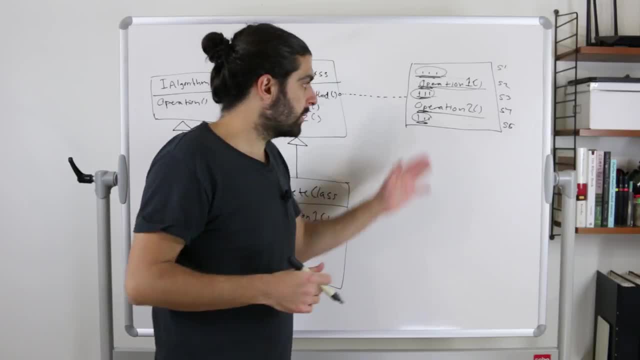 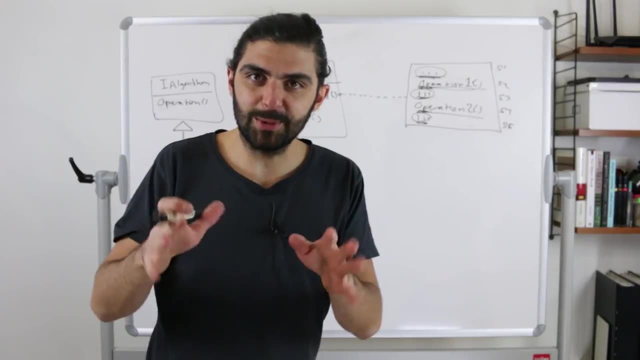 But you know, I mean, if you push towards, if you push in this end, you could probably see how you could figure out solutions where even the order could be altered. So that's just to caution you that generally this is when we get into this classic notion of that composition should be. 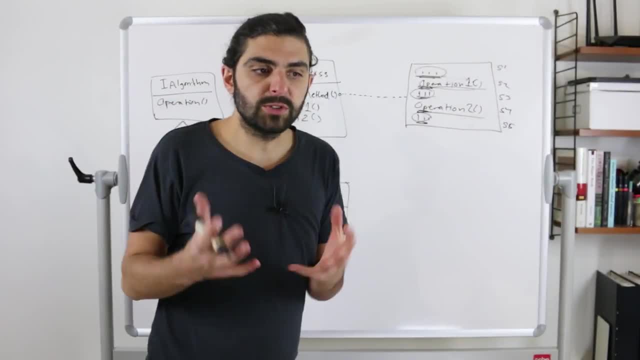 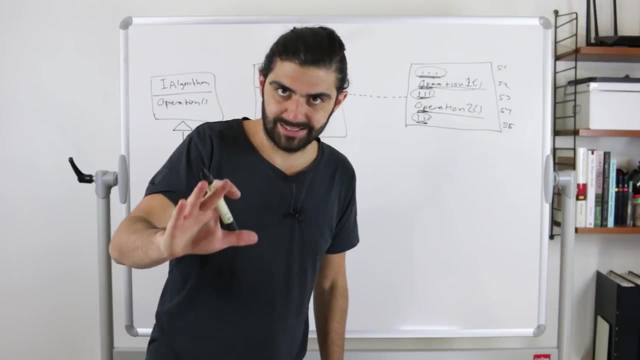 favored over inheritance, And template method pattern is built around inheritance. So in my subjective opinion, I would say that it's inherently dangerous to use, unless you're a specialist. You have a scenario which is super appropriate for the template method pattern If 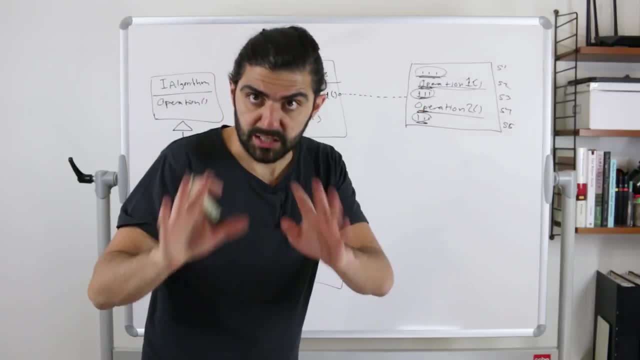 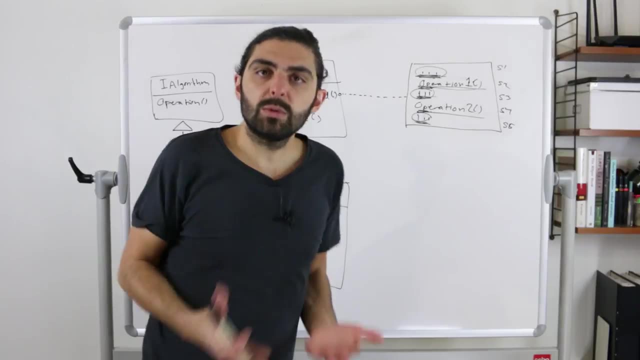 you know that the structure of your algorithm is invariant, is fixed, and if you know that these operations, these portions that you're assuming won't change, that they won't actually change, then by all means template method pattern. But if you have concerns about whether that's true or not, 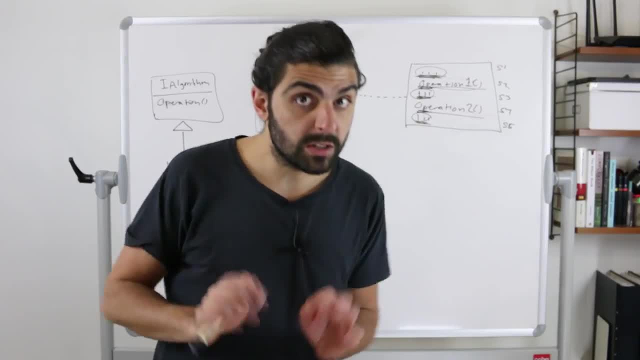 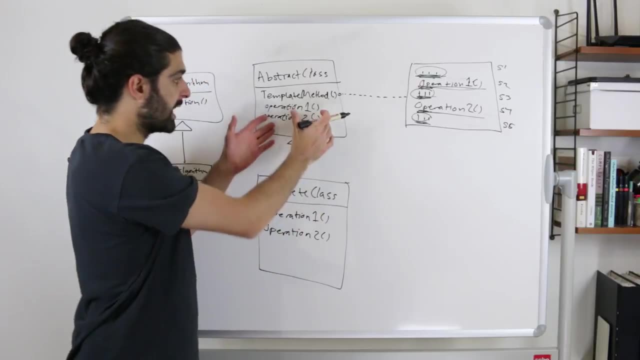 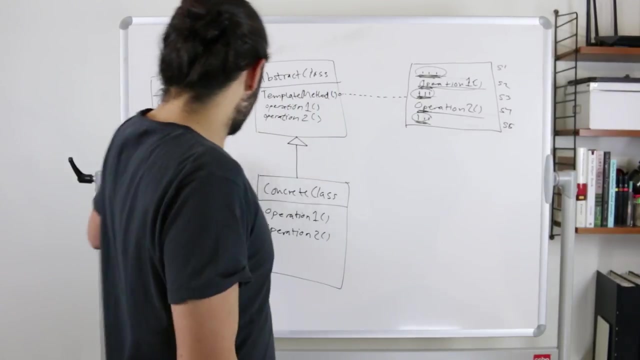 then maybe template method pattern is not appropriate for you, right, Because of inheritance. And again, if you think about it, another problem is that all specializations, all concrete classes that inherit from this abstract class, they have used up their spot for inheritance. if you're in a language that doesn't have multiple inheritance, When you're 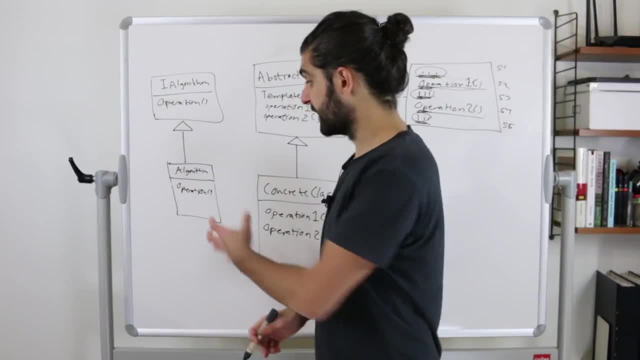 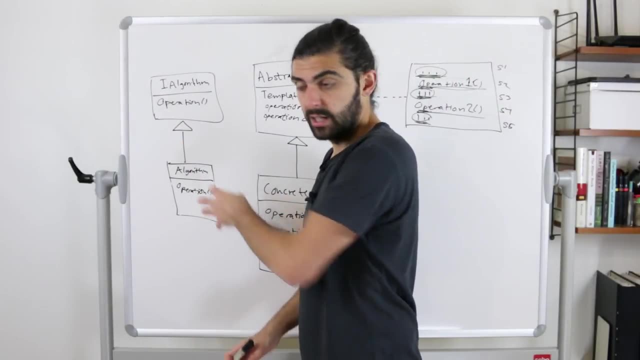 talking about strategy pattern algorithms, apart from the fact that they only do a single thing right, So it's unlikely that they will want to inherit from multiple things because they were doing a single thing. Apart from that, you're also implementing it using interfaces rather than 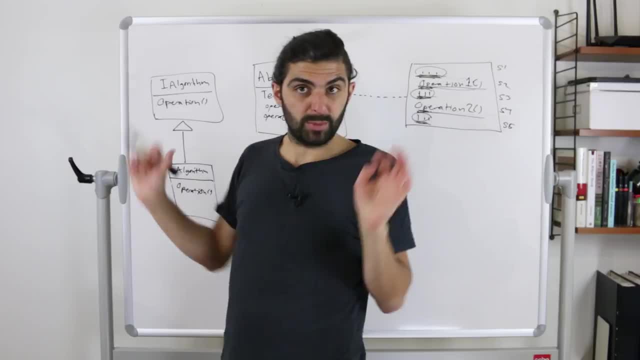 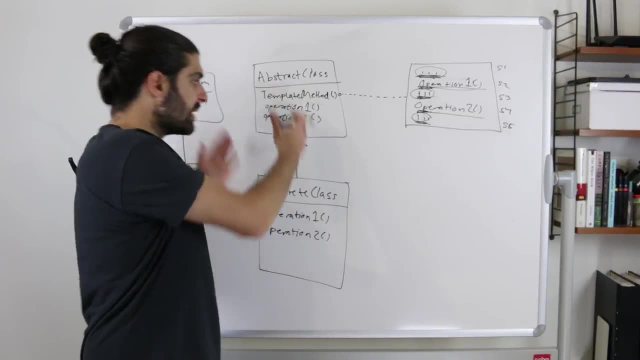 inheritance, which means that the algorithm could implement multiple interfaces, hypothetically, if you would want to, But the concrete class in the template method pattern. it has already used up its space for inheritance, so it can't inherit from anything else. Surely, yeah, you could use, you could tack. 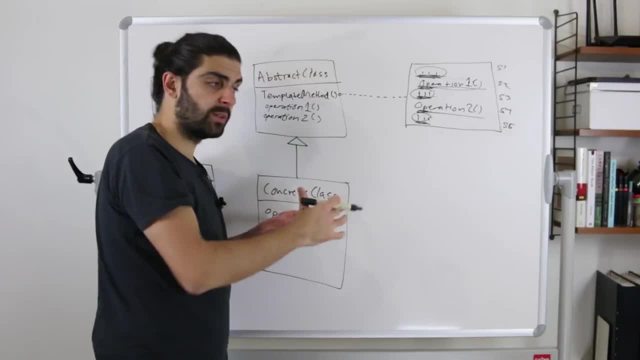 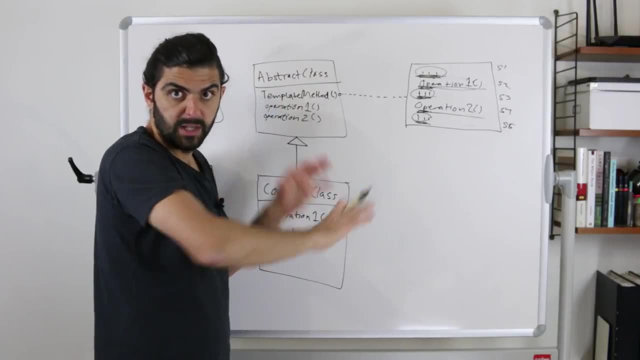 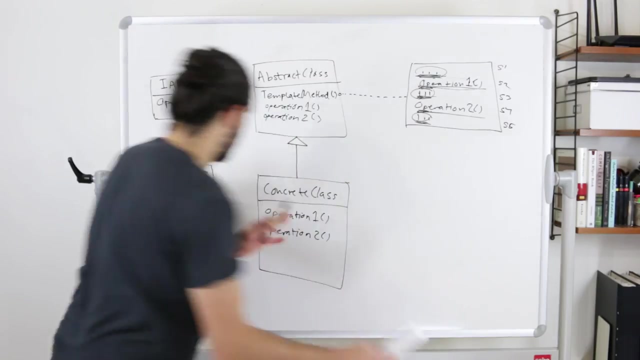 on interfaces to it. But if you have another pattern that also makes use of inheritance rather than interfaces, then you could not make this concrete class play nice with both of these patterns simultaneously. So again, be careful when using inheritance rather than composition. Anyways, let's get back to the program. So there's too much confusion going on. Let's now remove the. 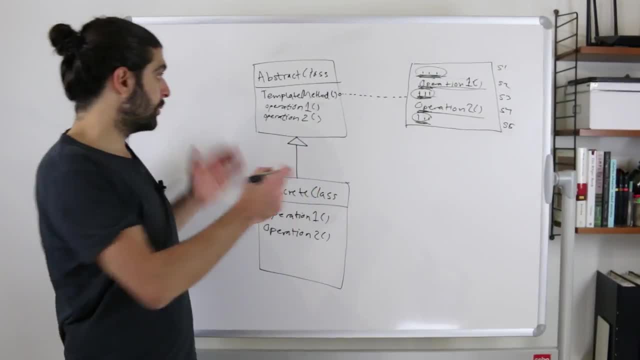 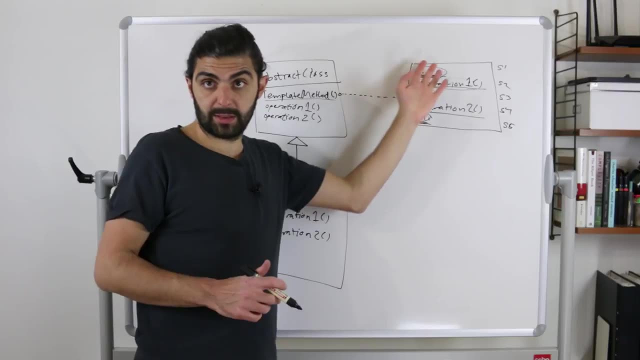 strategy Pattern. So this is the template method pattern. You have a template method that is concretely defined in your abstract class And the implementation of that template method is that you have some pieces of implementation, some you have some pieces of an algorithm. 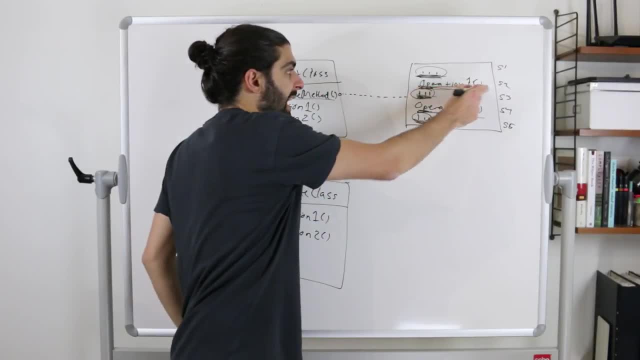 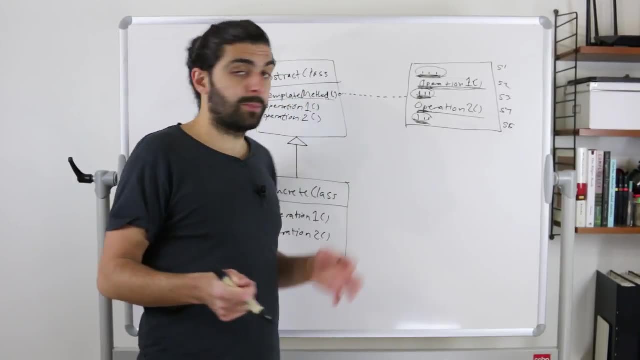 that you want to do, but there are some pieces of that algorithm that you can't know. You can't know what they will look like or how they should be performed in any particular specialization of this template, in any particular concretion of this template, in any particular use case for. 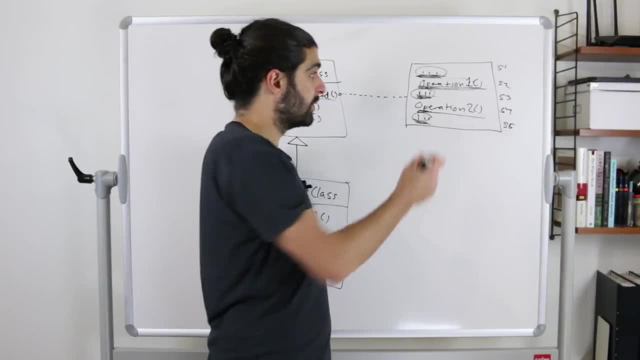 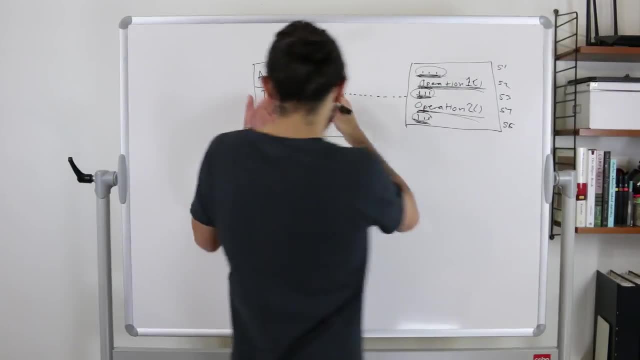 this template. So these you defer. you defer down to the subclass. you simply call an operation which is defined in the same class, which we hear call operation one and operation two. So you defer down to these operations. But these operations are marked as abstract because you don't have 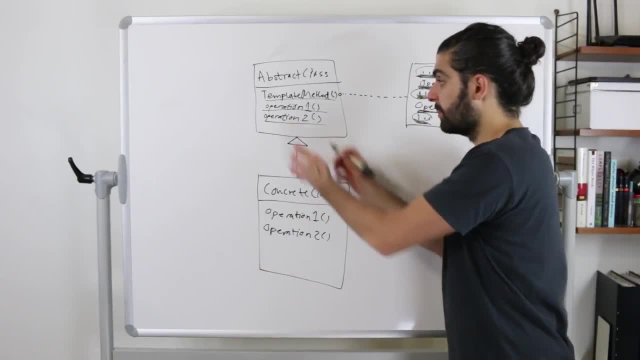 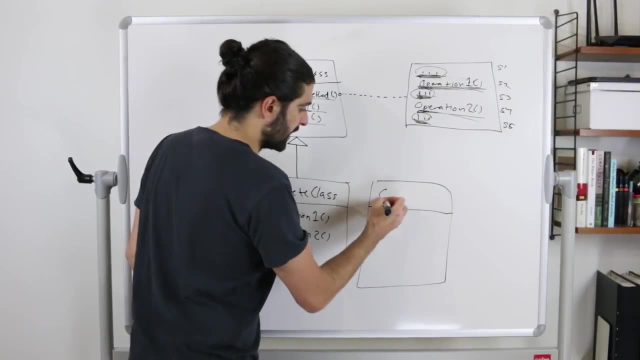 the implementation for them yet And instead you let some classes simply implement implementations for them, And clearly, of course, this means that you can have multiple concrete classes. So here we have concrete class one, and then let's say we have concrete class two, This two. 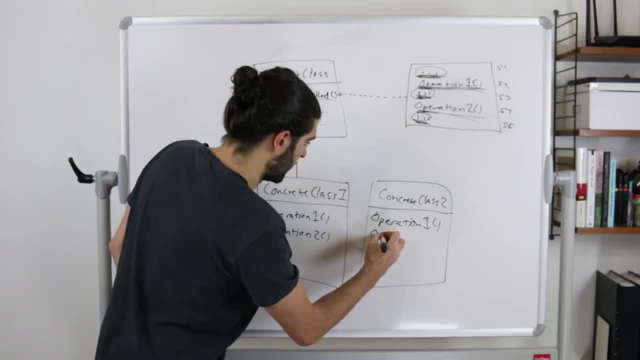 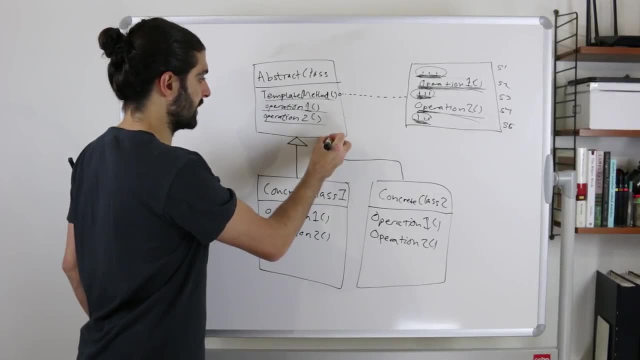 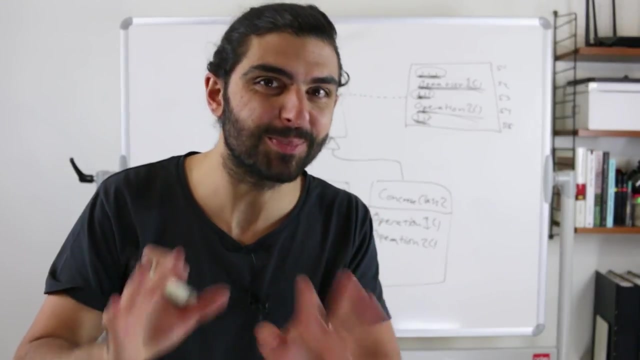 has to implement operation one and operation two, And this would then of course also inherit from the abstract class, And then you could keep on stacking multiple concrete classes. I'm sorry, I said we should move forward, but another problem that you could see: 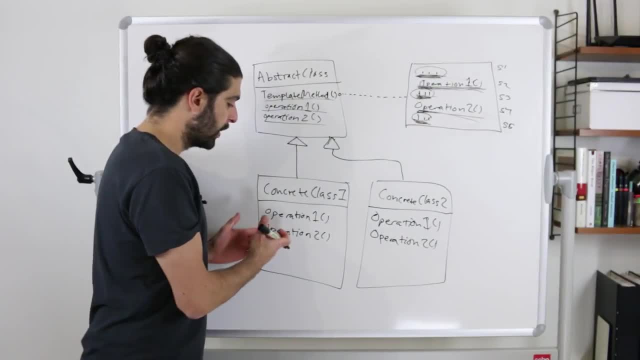 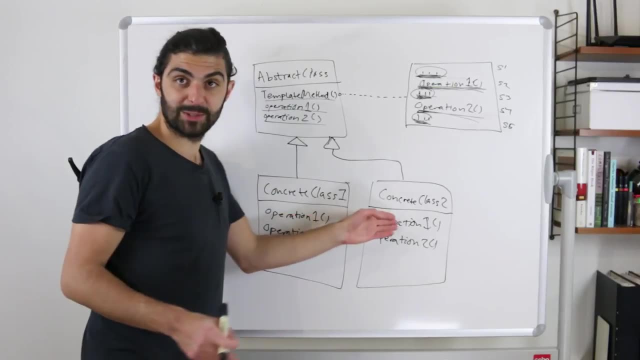 with the template method pattern. right is what if you end up in scenarios where operation two here is the same as operation two here, but operation one here is not the same as operation one here. But clearly of course you could find other ways. 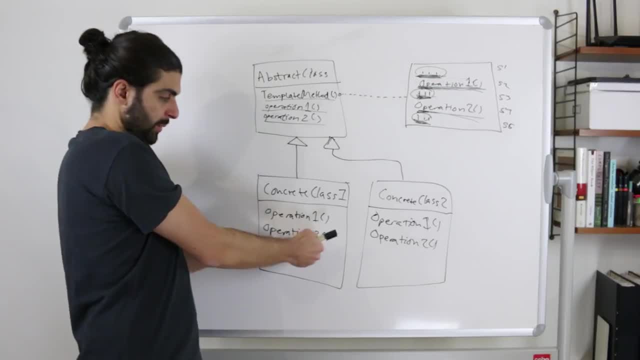 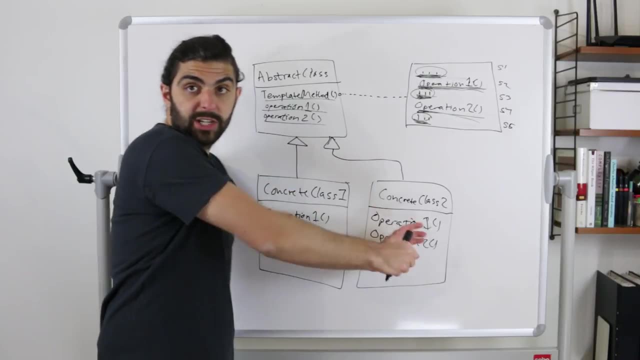 of fixing that scenario? I mean, you could, for example, inject operation two into concrete class one and inject operation two into concrete class two, So you would have a single implementation for that operation. to inject it here and inject it here, and thus you've only written it once. 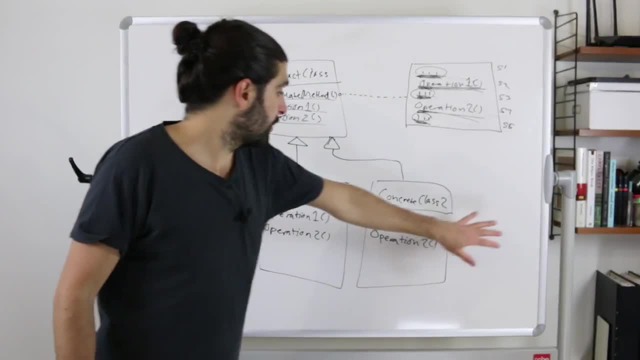 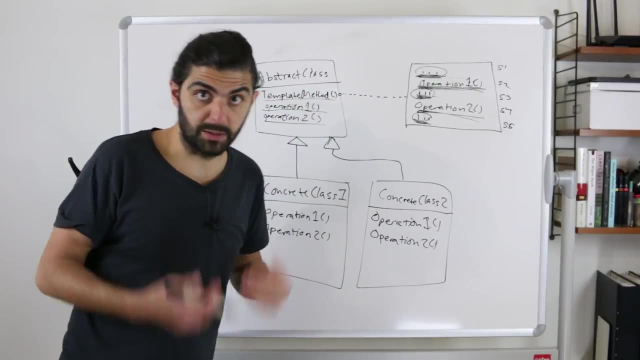 But I mean, now we're talking about something else. Anyways, you would have a number of concrete classes that all inherit from this abstract class and that supply implementations for the operations that are missing, that are missing from the abstract class. So you would have a number of concrete classes. 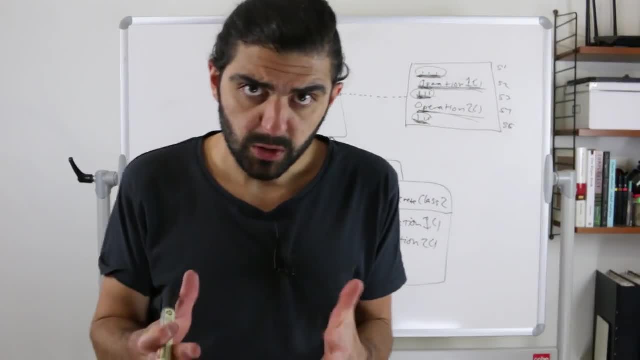 that all inherit from this reused algorithm. Now, I mentioned that we would talk about Rails, or more specifically, ActiveRecord, But actually I mean, if you're not familiar with Ruby on Rails, never mind. I mean, it was just an example. 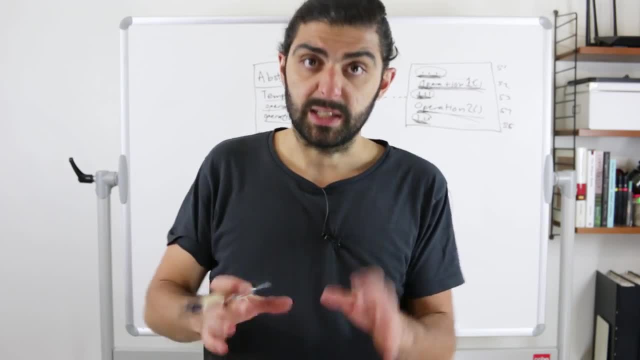 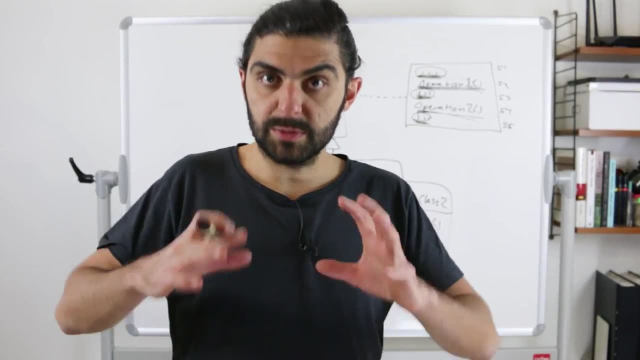 so that those of you that are familiar gets into the right mindset. But anyways, here's the point. Consider a scenario where you have some kind of object relational mapper, some kind of ORM right, some interface that acts as the bridge between your code and your database. 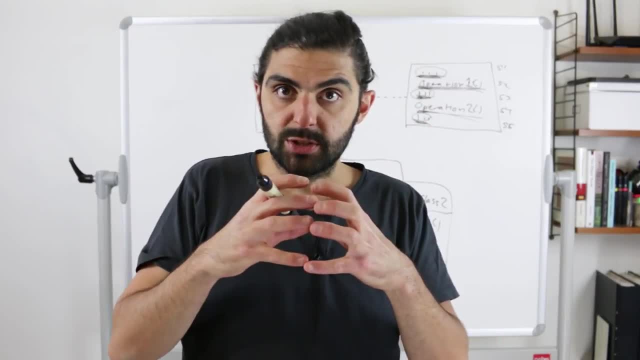 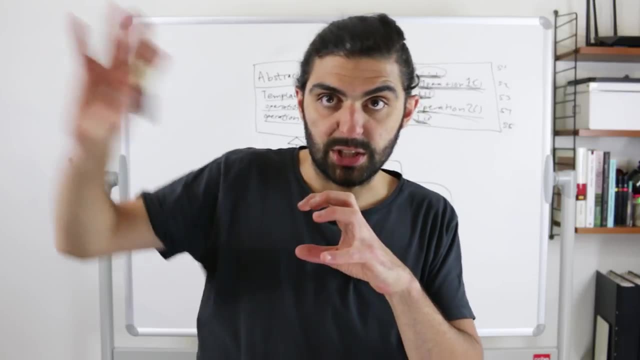 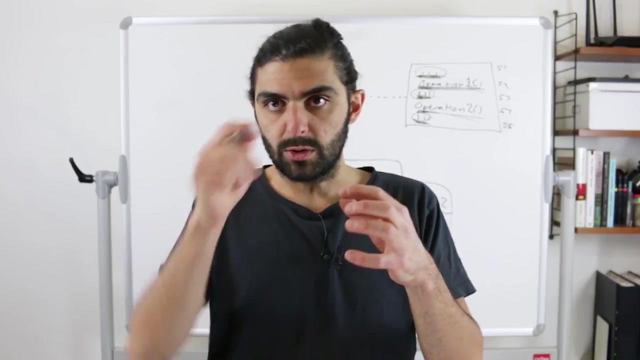 So you are handling objects in memory in your application, but when you call save, when you call save on these objects, they are actually saved, They are actually persisted in the database. So like if you create a new record, you make a new instantiation and then you say save. 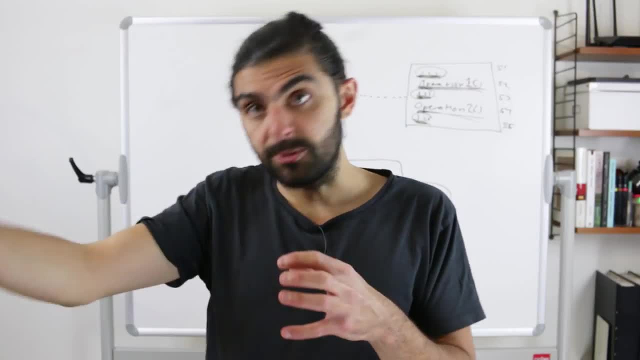 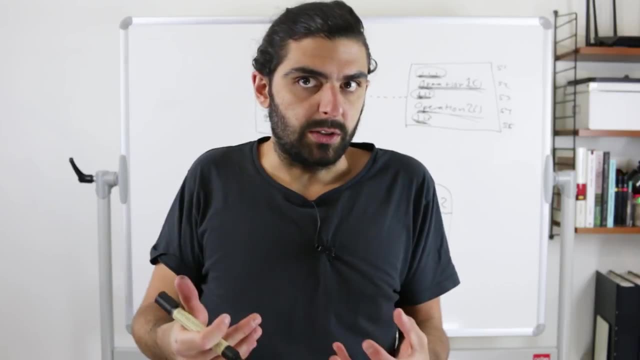 you call save on that record, it's actually saved in the database. Or if you get something from the database, you have it in your memory and then you alter a field of that record and then you say save, which would then be analogous to update. 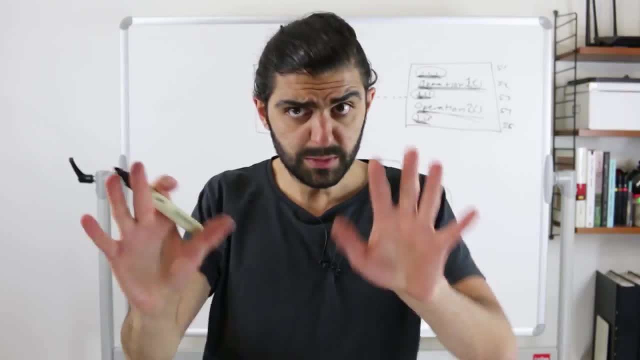 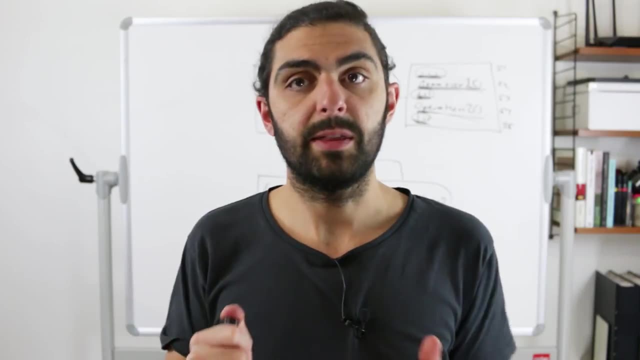 you would actually execute an update query in the database. All right, this is just an example. The reason I'm saying this is: think about this, Whoa. The reason I'm saying this is think about this. There is some method in this base class. 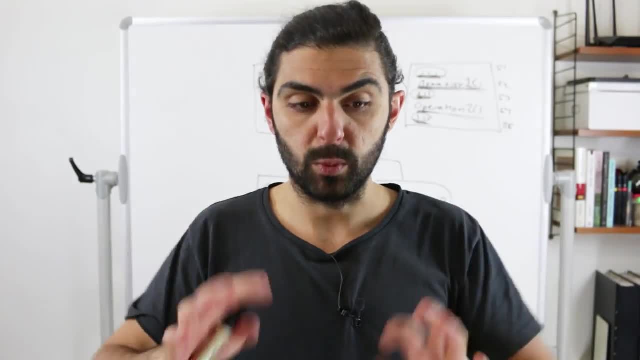 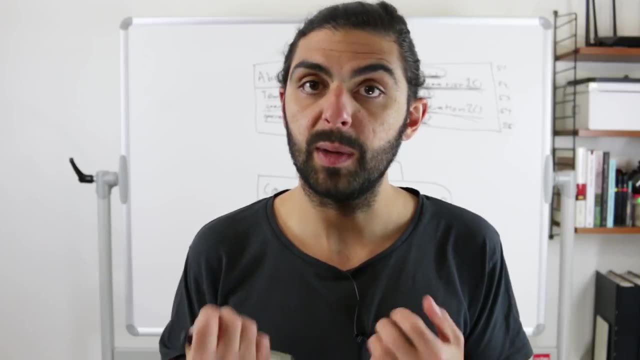 like you have think of it this way, you have an abstract base class that whenever you want to create some kind of record- and when we say record here we mean database record, We mean a model that you want to be able to save- 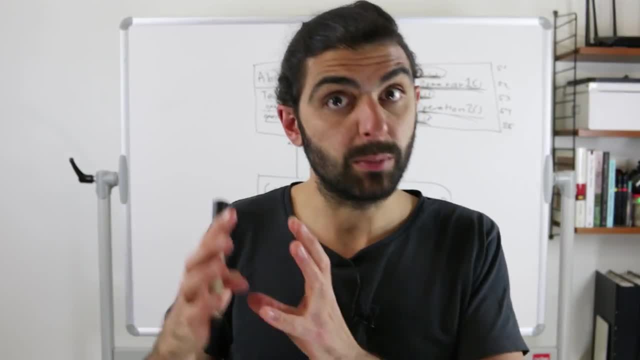 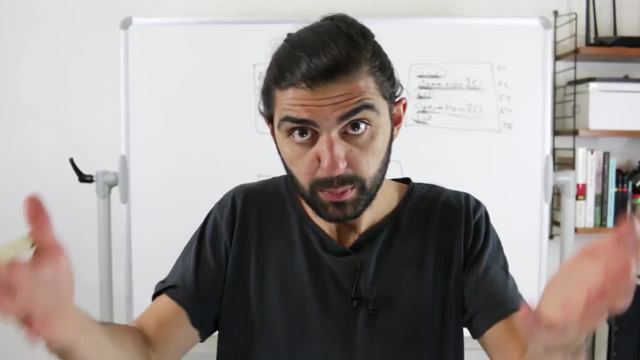 in the database. Think that has a one-to-one relationship with a table in the database, if it's a relational database. So your model could be a user or a comment or a post like a blog post or whatever you're modeling in your scenario. 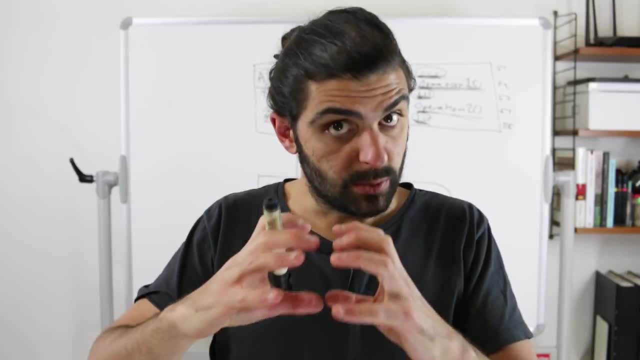 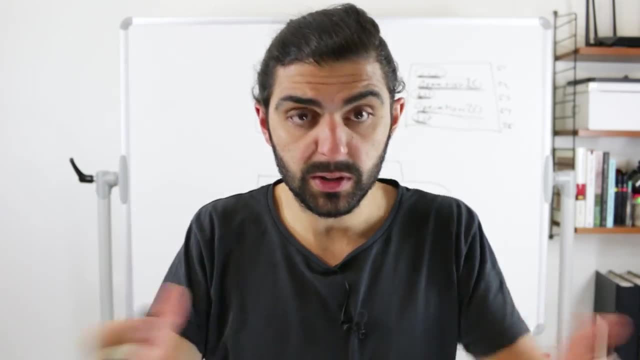 But let's say user right. So you create a class which is user and this user class inherits from your model base class and maybe you call this model. I mean, if you're building your own sort of database connection layer, maybe you would call this model. 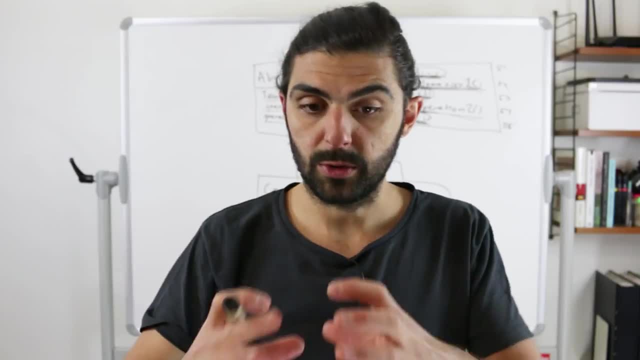 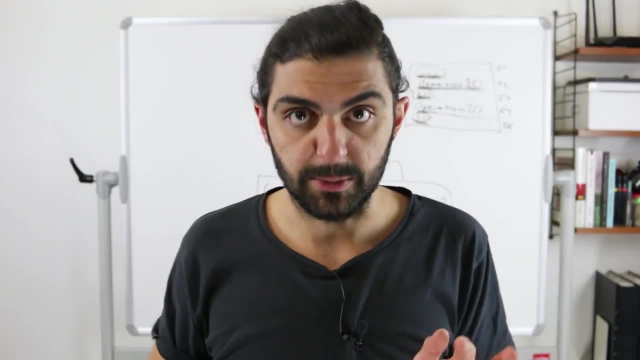 But if you're using Rails, for example, this would be active record, So your user inherits from active record. By the way, I haven't been in Rails for a long time, so I apologize terribly if things are completely different now, But again, I'm just saying Rails. 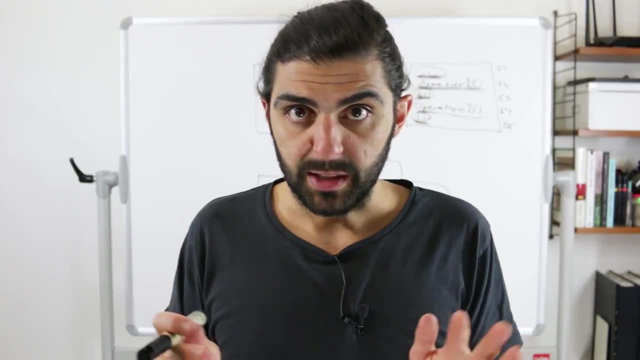 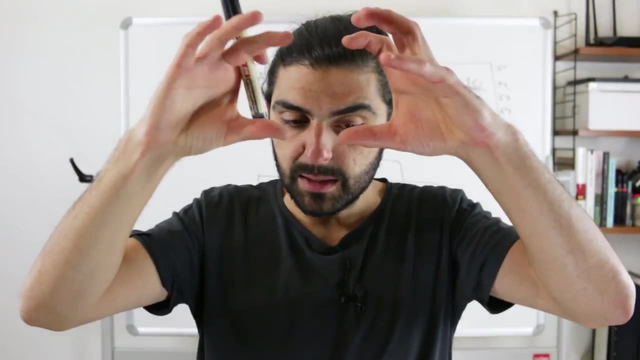 to put you in the same mindset. I don't necessarily mean that any of the following things that I'll say have anything to do specifically with Rails, but by analogy, Either way, you have this base class of a model and this base class. that base class would construct. 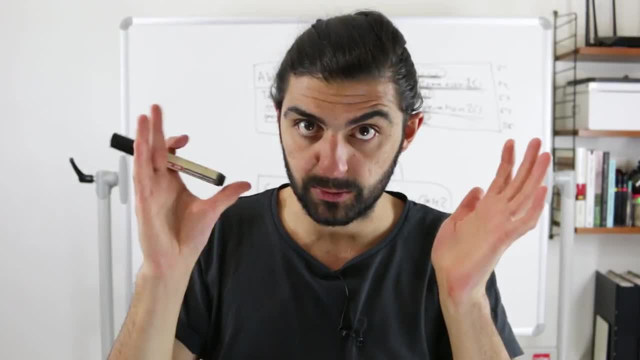 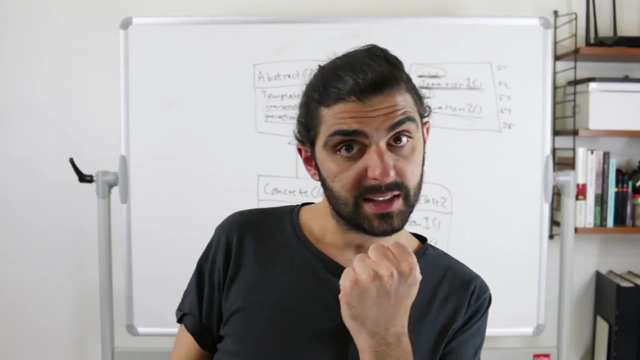 an implementation or would have an implementation for, for example, the save method. So you want to be able to take any particular user right. You have the user class and you have an instance of the user class And then on that instance you would say save. 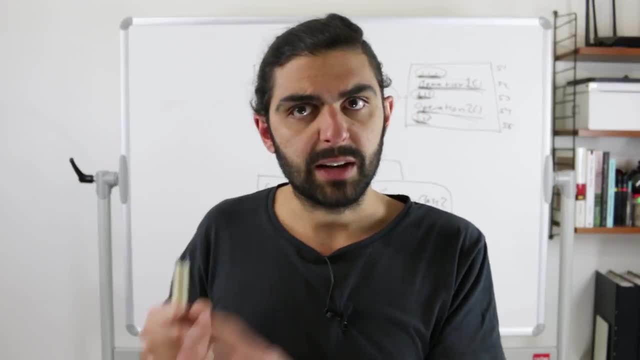 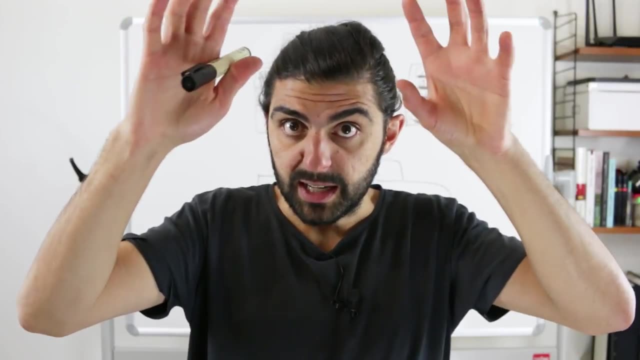 You would call the method save, And when you call the method save you don't want to have to implement that save method in the user. You probably want to have to implement that save method simply in the base class. So you want to do it once so that you can use it for. 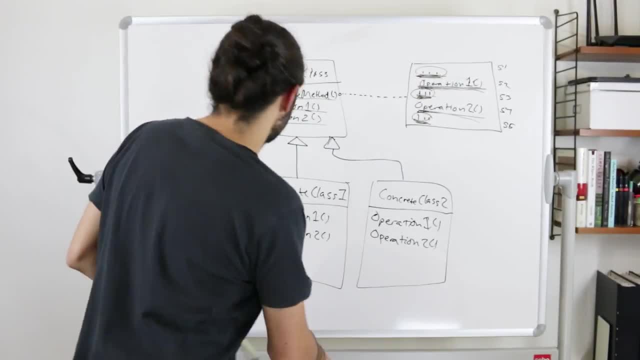 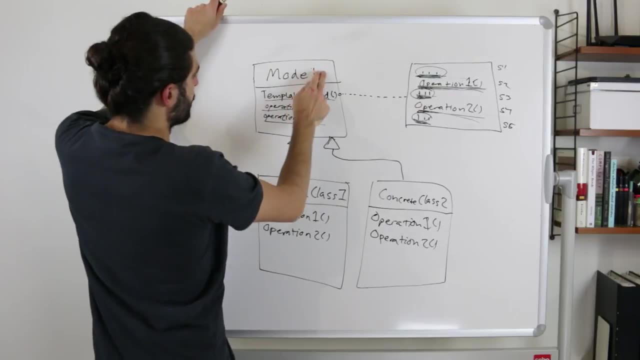 reuse it for all of your different models. Let's redraw this to think about it in those terms, right? So instead of abstract class here, we call it model, a record, right? Maybe we should actually call it record. Let's call it record. 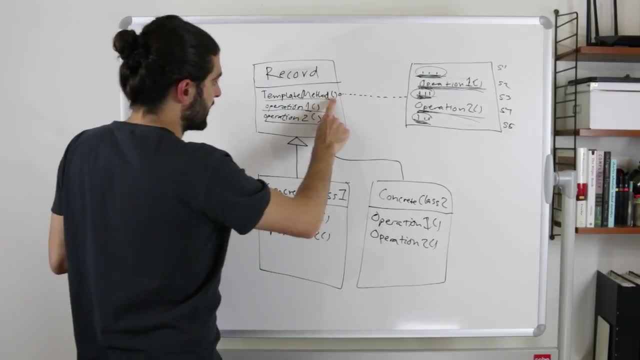 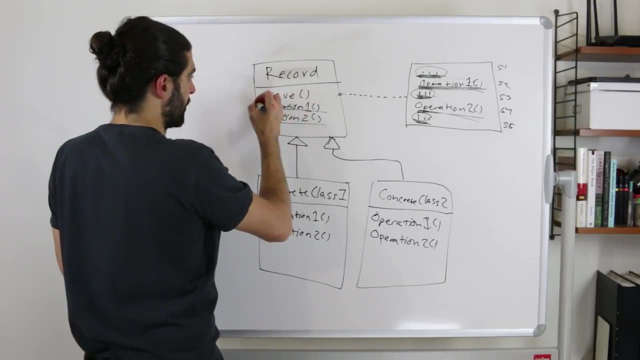 So it's super clear that it's a database record record And instead of this template method right Now we have, we have an actual template method And this template method is what It's: save. save takes no arguments. 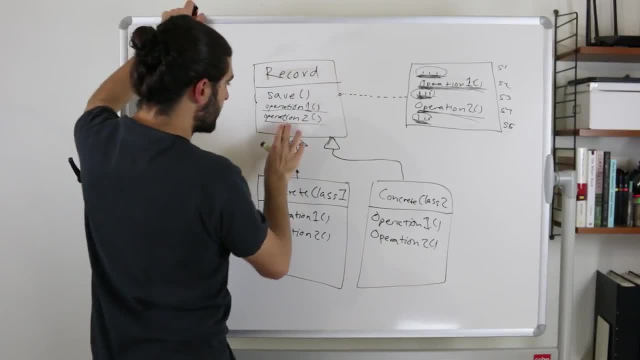 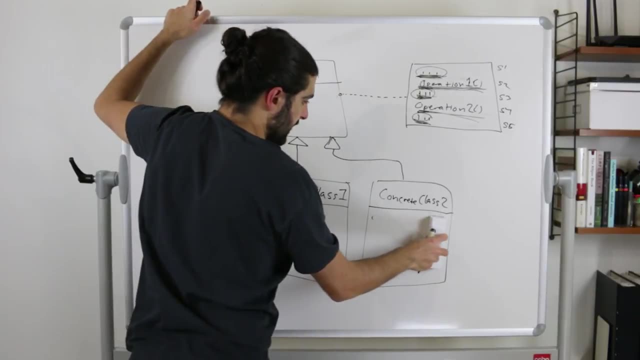 essentially takes the record and saves it to the database. We don't know what these operations are yet- operation one and operation two- So let's remove these, which means that we'll remove them from the concrete class number one and the concrete class number two. 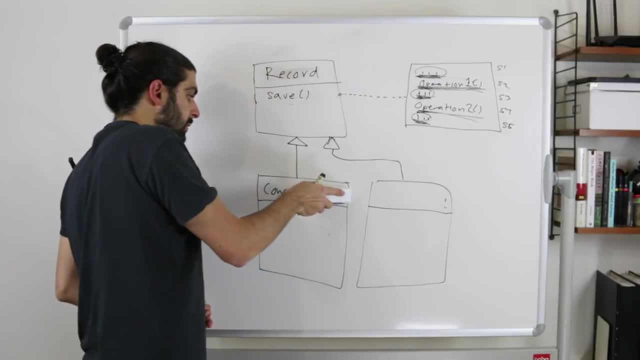 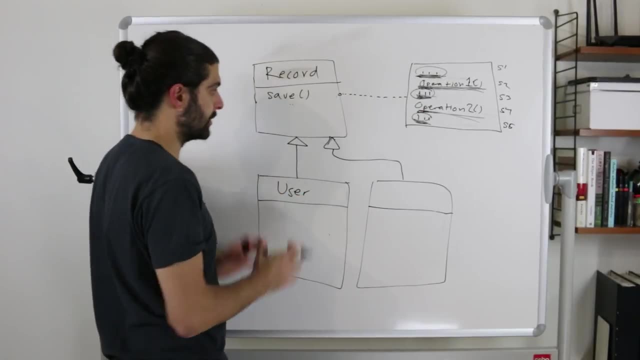 But also let's remove the names concrete class two and concrete class one And let's give these actual names. So let's think of this as the user, a user right, The model of a user, a user record right. 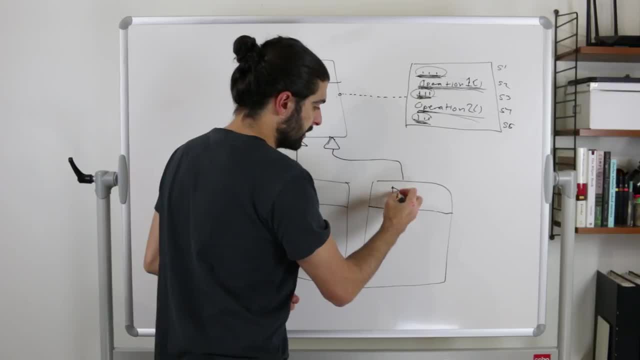 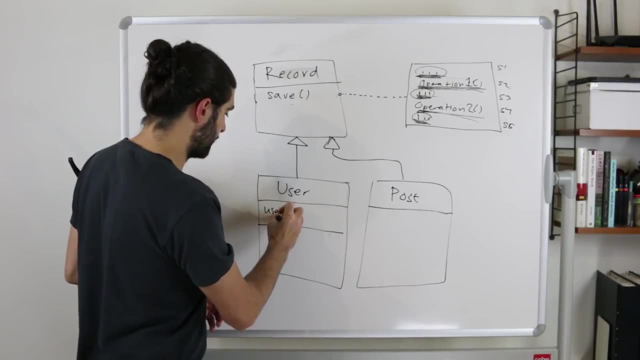 The user record is defined by this class, And then maybe let's think about this as a post. So I mean, what would be? what would be specific to these? Maybe users have a user name. Let's not go complex, Let's just put the username here. 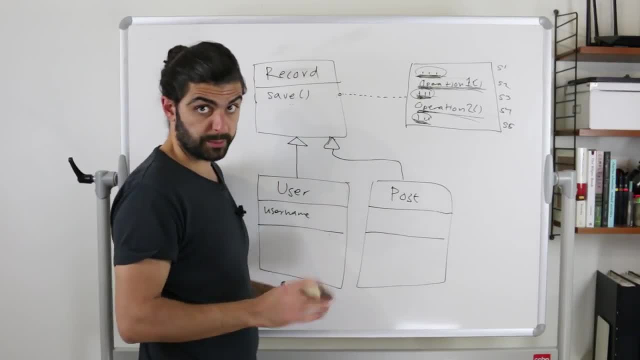 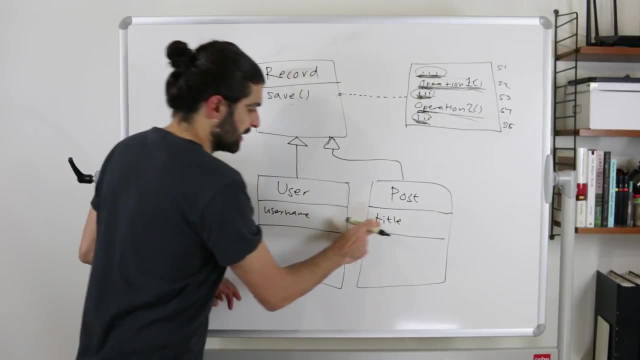 And maybe the post actually maybe belongs to a user, but let's not think about that. in order to not make the scenario complicated, Let's just say that a post maybe has a title, or actually, again, if you have a title, maybe you would have a body of text. 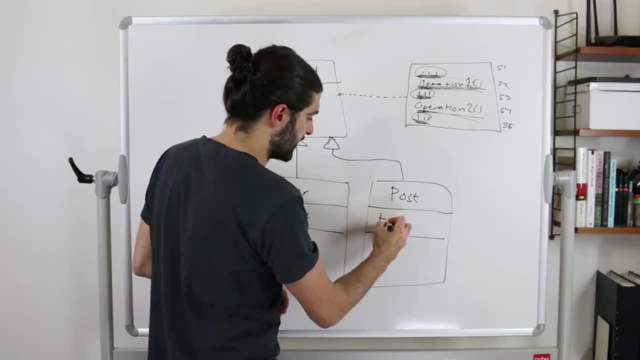 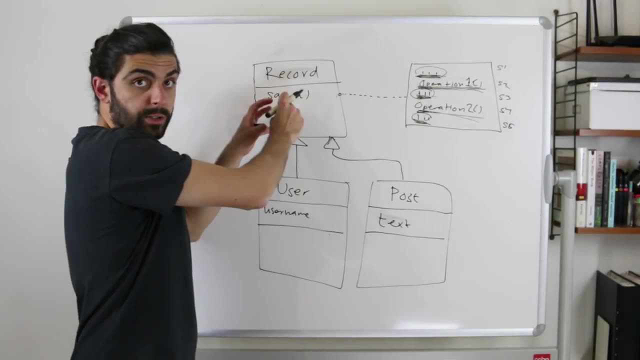 So let's just say that the so let's just say that that the attribute that it has is that it has a text, so you can make posts that have text and you can have users that have usernames, and both of these are records, because we have this save method. 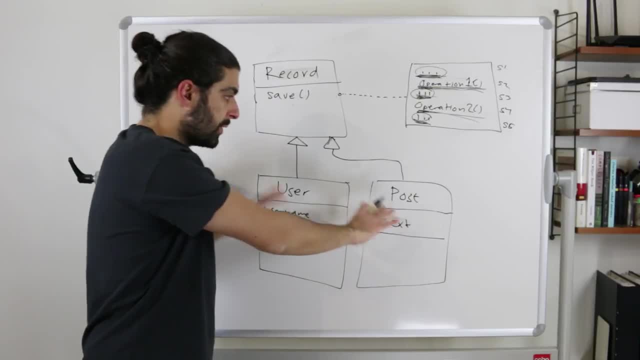 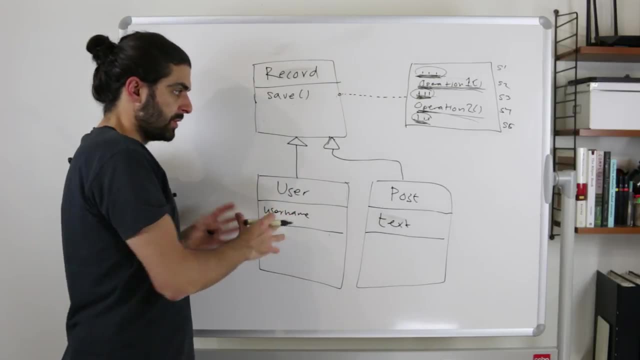 the save template method. that means that these both can be saved. but here's the thing, then. what we're saying is that maybe there is something that's specific to userness and something that's specific to postness that we can't foresee when we're creating the record. right, actually, let's. 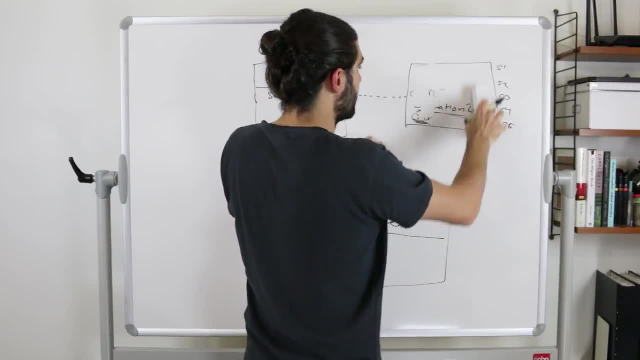 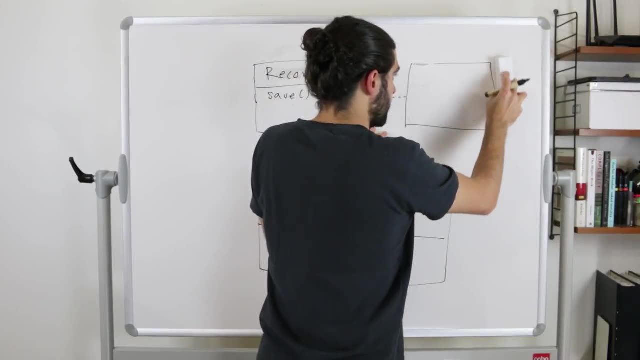 let's remove the contents of this, this thing here as well, like this peek into the implementation of the template method of the record. so let me remove all the stuff in here and let me remove these here. so the save, i mean it runs some kind of query to the database and we're not going to 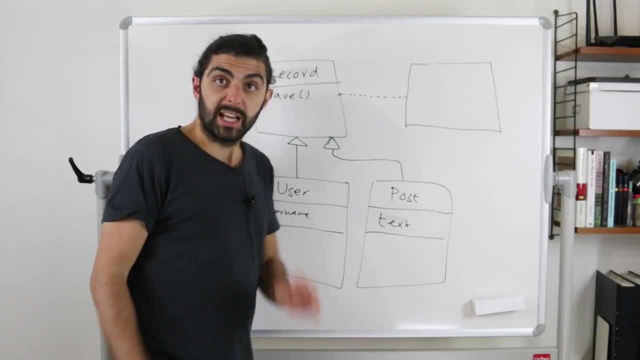 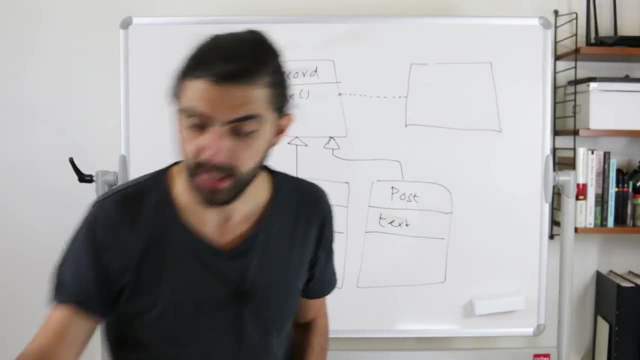 be concerned about that. but the point is that maybe we want to do something else, and here let's talk about hooks. so we talked about two different types of operations. again, as mentioned by the gang of four book. they talk about primitive operations, ie abstract operations, and they 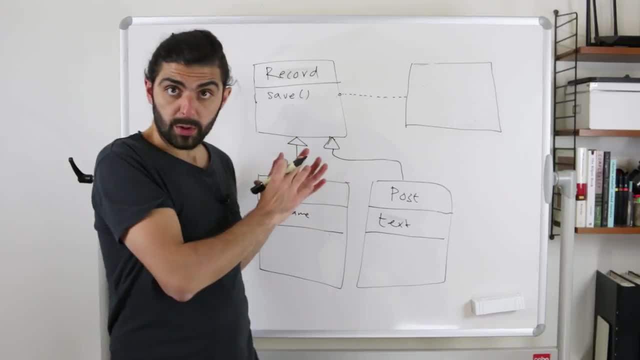 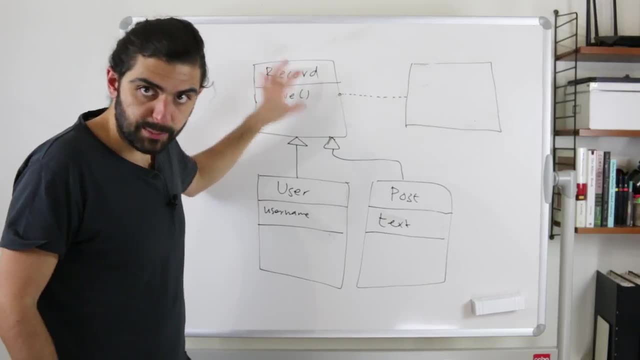 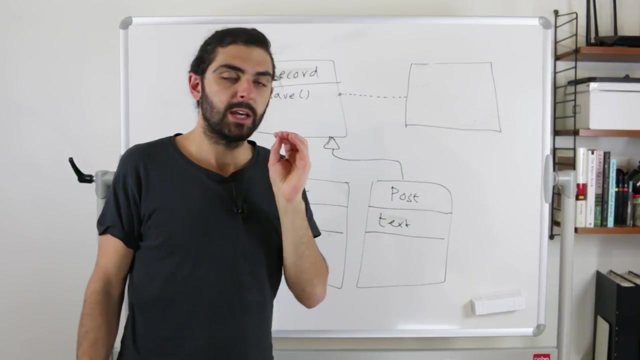 talk about hook operations. so what we looked at before was abstract operations, in other words primitive operations. it was operations that the record here, that the abstract class could not define itself but wanted subclasses to define. that's an abstract operation. but if you have a hook operation, the idea is that the record would supply an empty implementation, which means that 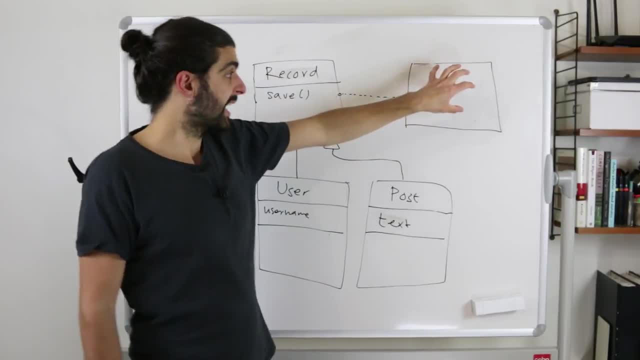 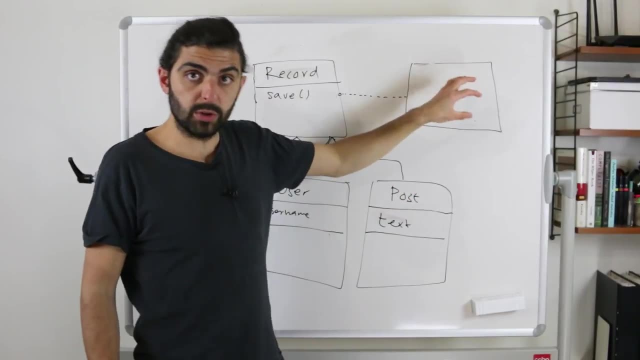 the record in its save method, ie in its template method, can make use of this hook method. it can call this hook method and it can call this hook method and it can call this hook method and it can call this hook method because it's not abstract, right? it's an actual method, so it can call the. 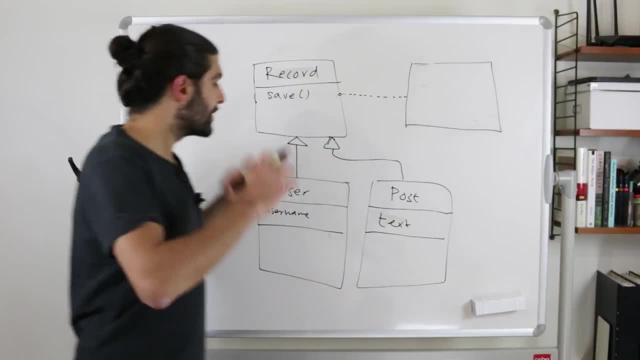 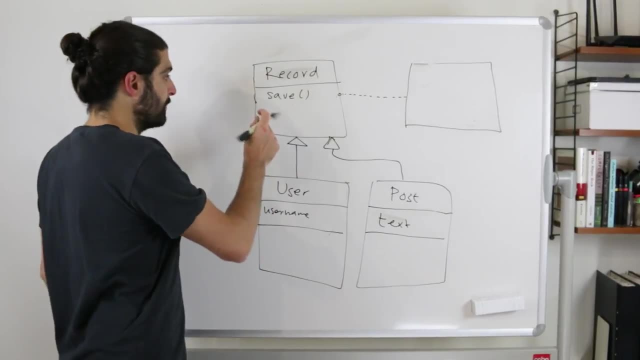 hook the hook method, but the hook method won't do anything, but you can still override it in the user in the post to supply an implementation. and if this sounds strange, think about it in this way: what if you would want to hook in to the life cycle of saving? so let's say that you wanted to. 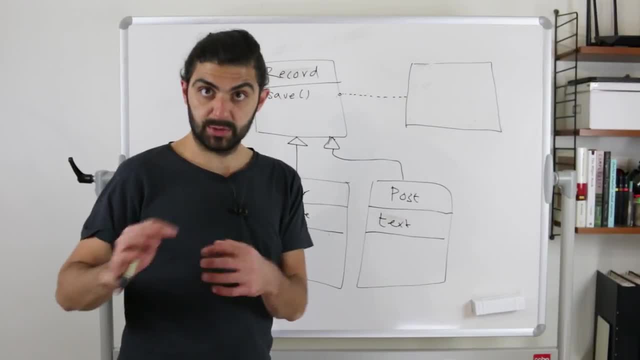 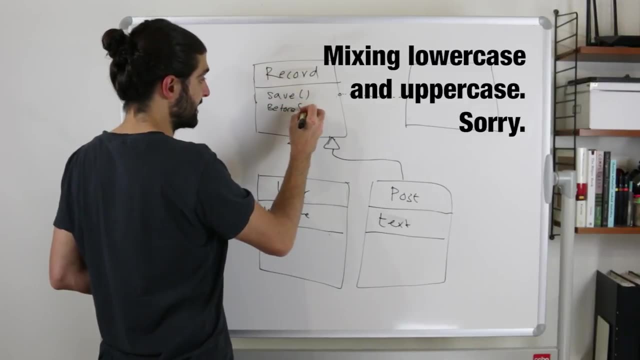 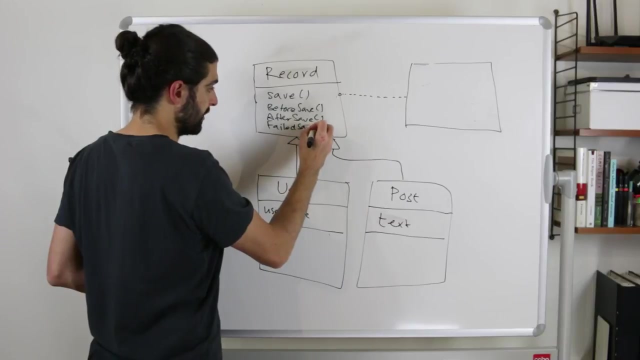 know when the record was about to be saved and when the record was successfully saved. so so then you can have two hook methods. you could have, let's say hypothetically, before the record was saved and after save, and let's even say maybe we would have a failed save method. and these are 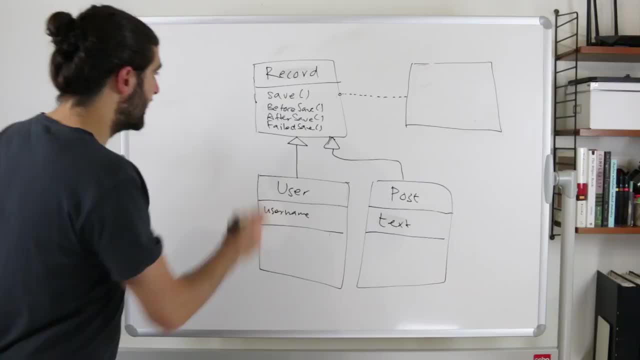 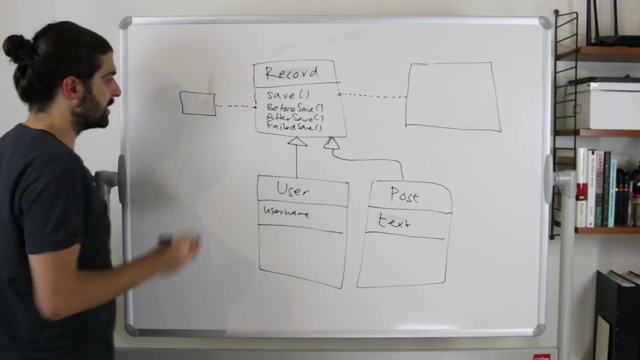 not drawn in italics. these are not abstract methods, instead the implementation for all of these. let's use this syntax again with like the circle and all of this, all of these dots, and then this box to show the implementation. i'll simply put a dash here to show that this simply has no 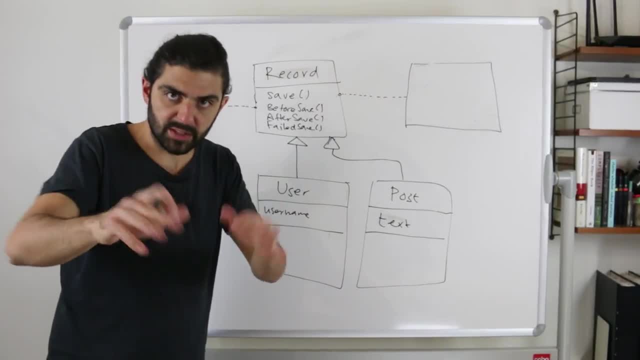 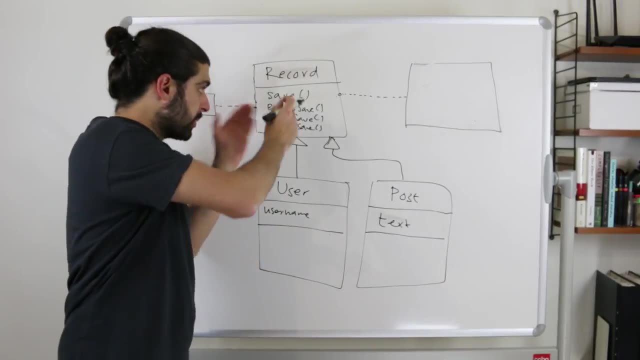 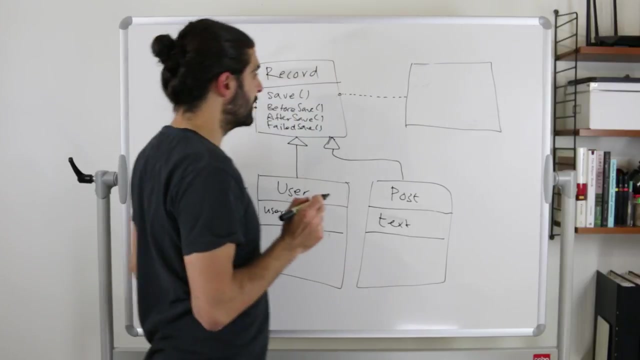 implementation. the before save does nothing. i mean it has an implementation, but the implementation is empty. so before save does nothing, after save does nothing. fail save does nothing. so neither before save, after save nor fail save do anything. they have sort of empty implementations. why? because then, when we implement the save method, let me put this: 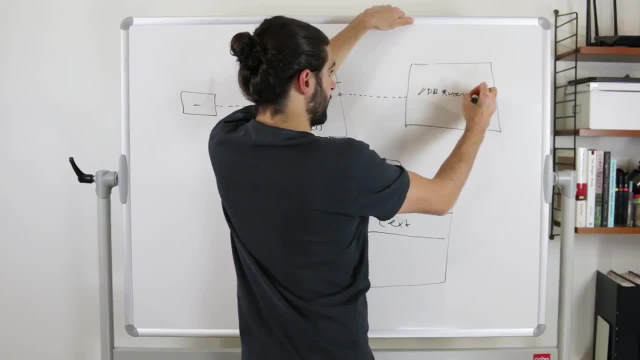 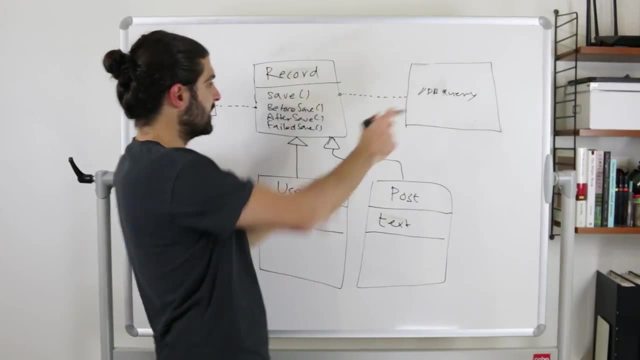 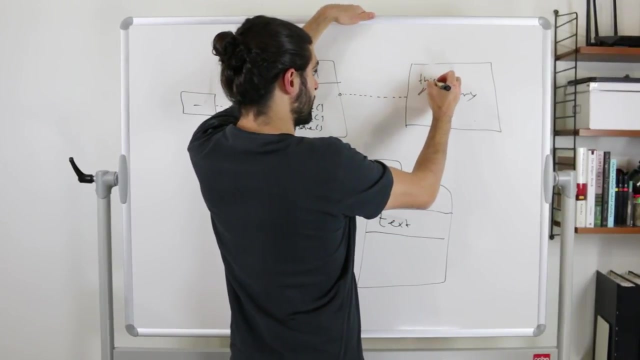 slash. slash here to say db query. so here there is some kind of complex database query that actually saves the record. let's, let's not worry about that, but before this, the implementation of the same method does that actual database query that will save the record. it can call this dot before. 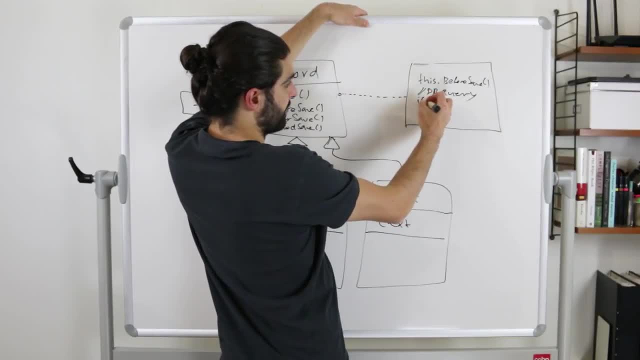 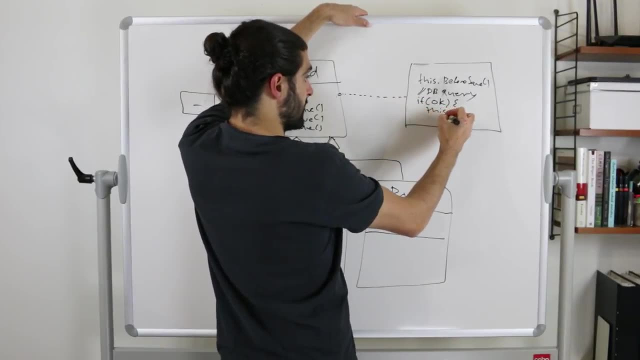 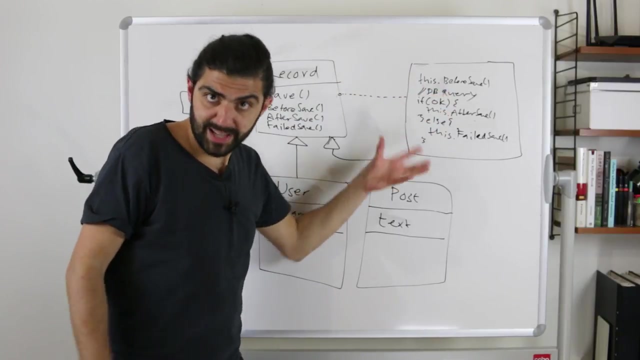 save and then after it it would maybe say: if okay, i'll just write if okay, in order to check whether the the query was okay, then it calls this dot after save and if it wasn't successful, right else, then we call this dot failed save. so i mean, if you think about it, this kind of becomes like events. 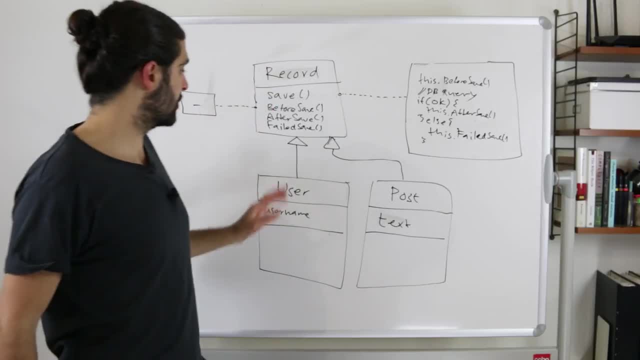 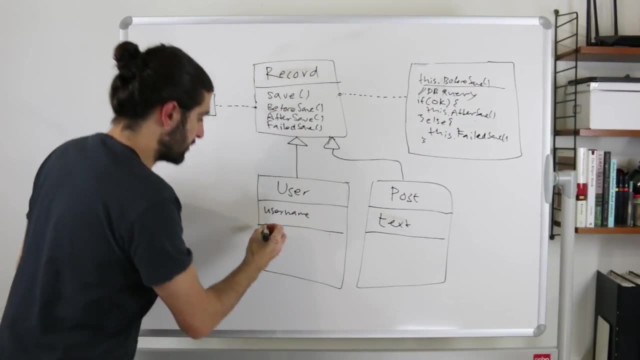 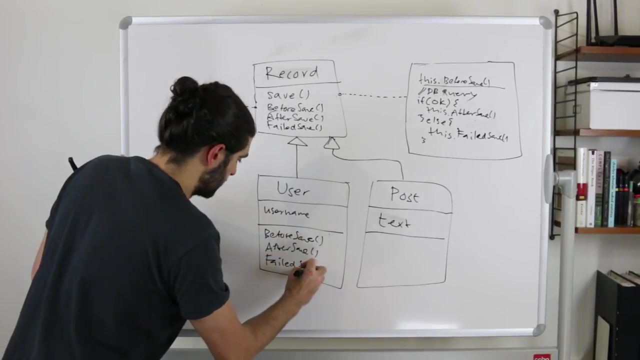 clearly events have other advantages or observer pattern have other advantages, but whenever the save method is called first, we do whatever the subclass says we should do before save. so sorry, i forgot to put here before save, after save and failed save, and actually i mean these need to be. 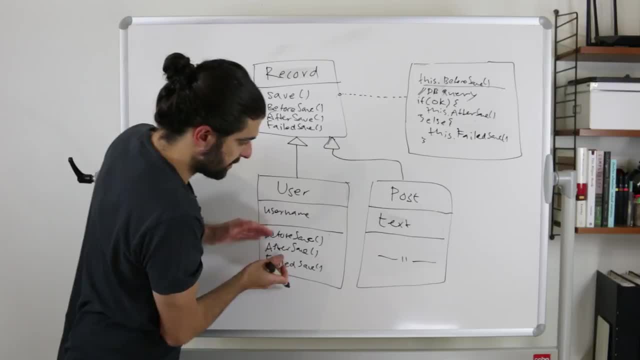 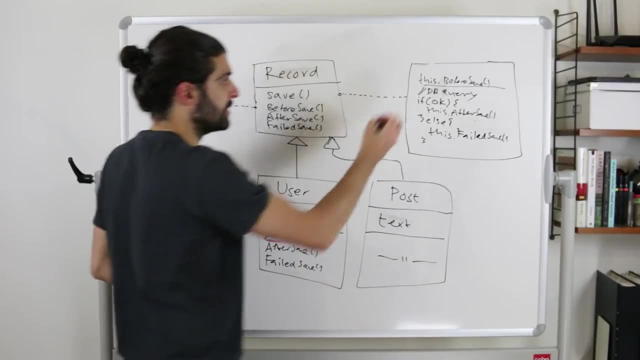 here as well, but i'll just type that to sort of indicate that, okay, these methods should also be here. sorry about that. so the whatever the user says should happen before save- before save will be run before we do what we are actually supposed to do. so we're going to do the same thing here. 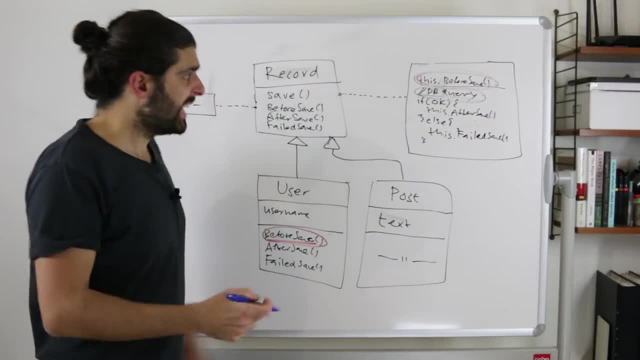 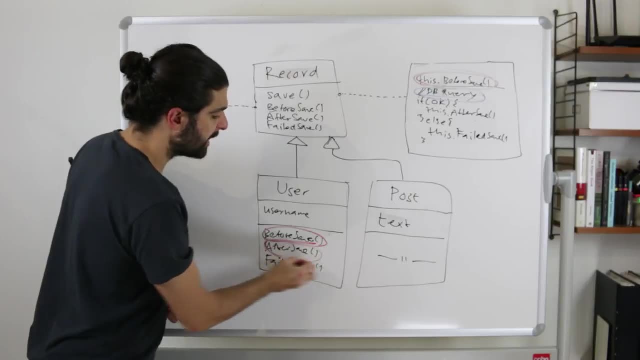 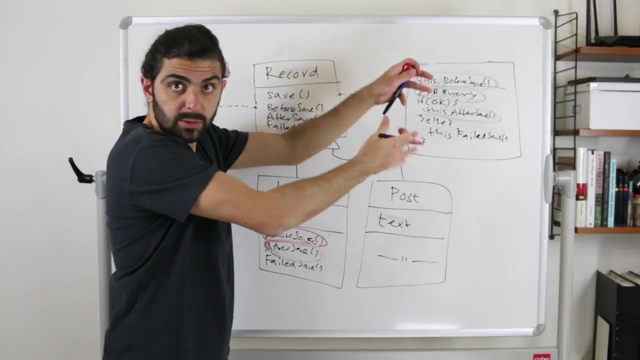 we're supposed to do, i mean before we actually execute this query, and then, if the query is successful, we will run whatever the subclass is specified that we should do after we save. so we run this after save method if it was successful. right, the algorithm, the algorithm, here the meat. 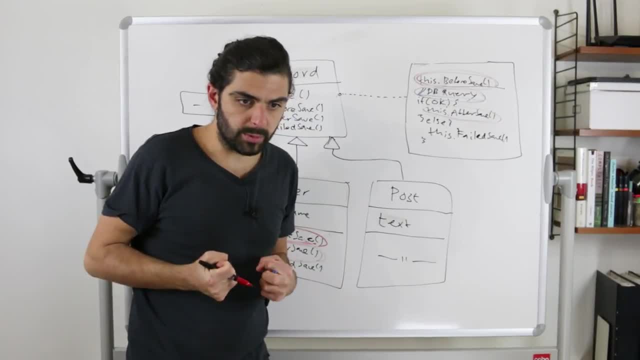 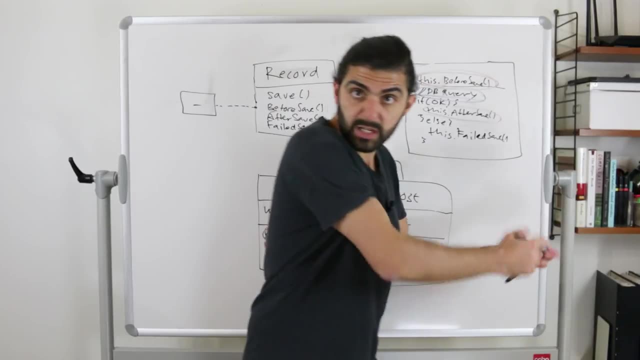 of the algorithm is that we're saying something needs to happen before we save. then we try to save. if we successfully save, we do one thing, but if we fail to to save successfully, we do another thing. but again, these three things: what happens before, what happens if we're successful and what happens. 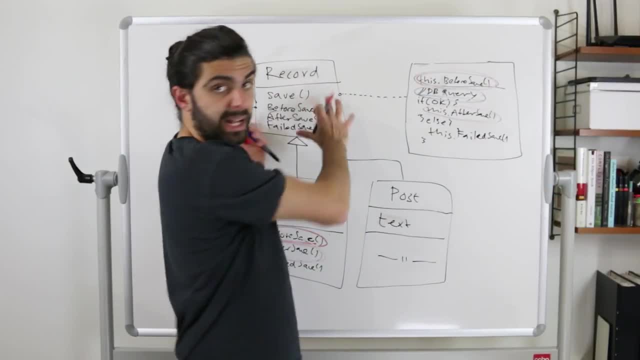 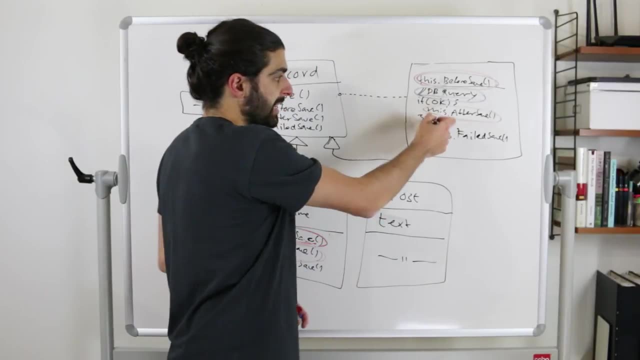 if we're in success, unsuccessful. these things you can't know at the abstract level, you can't know generally for all records, because different records might want to do different things. and then so if we fail, if we end up in the else branch, we will run failed, save. and then if we 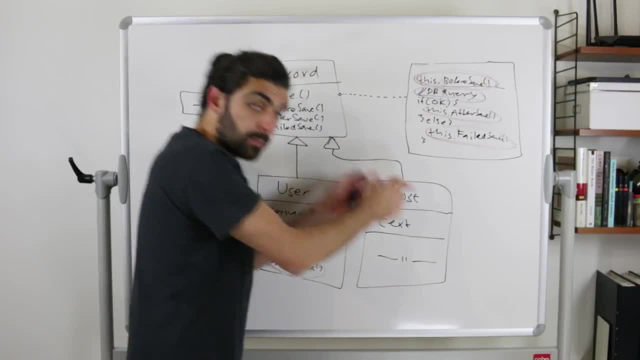 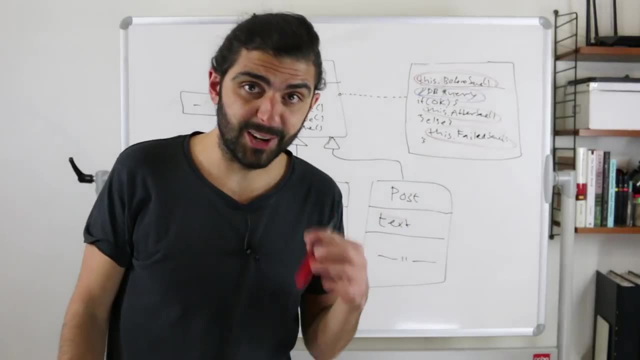 happen to have a user, we will run the failed save method. but if we happen to have a post, we'll run the failed save method of the post. and actually i mean, as i think about this when i'm looking at this, maybe it doesn't make a whole lot of sense with the sort of in a save scenario. 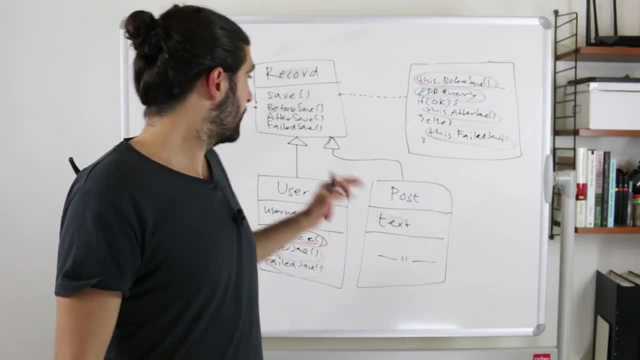 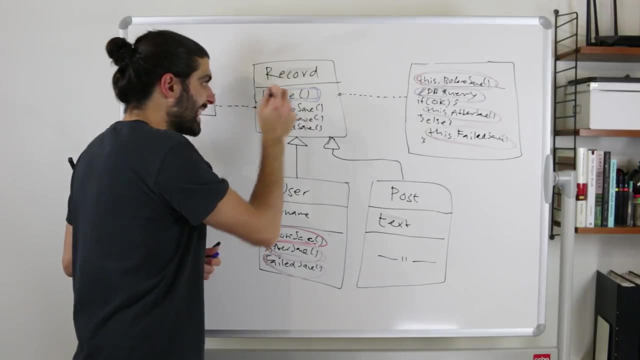 maybe it would make more sense to think of having hooks for validation. so let's say that. i mean, let's just be super explicit here: the save method, here, this save method, that's our template method. that's the template method, because this is the template, this is the thing that can have. 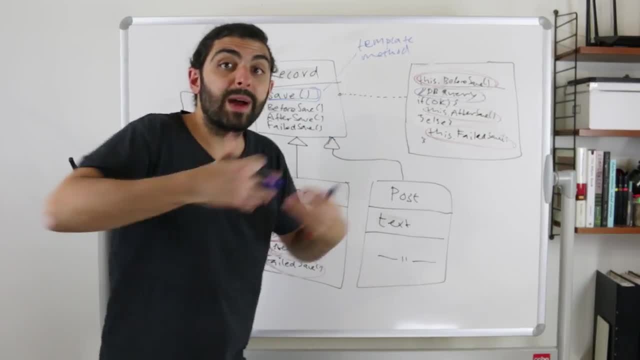 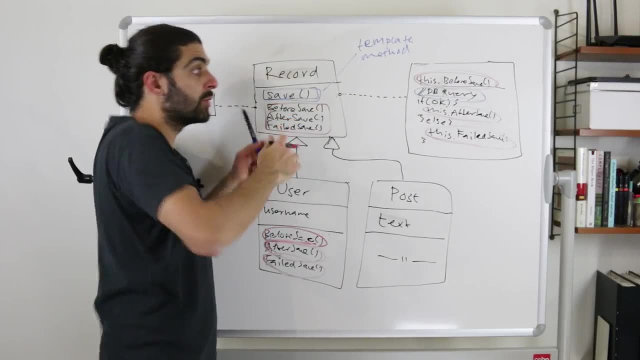 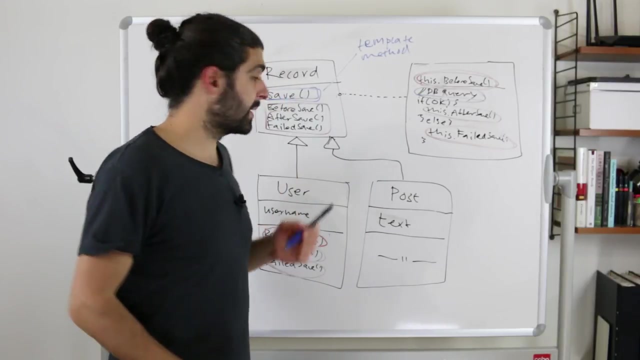 specializations, where the specializations are not created by overriding that method, but where the specializations are created by overriding the particular methods that are used within the template method. so, if we think about it, instead of thinking about save, let's think about validation, right? so what if this method was validate? so 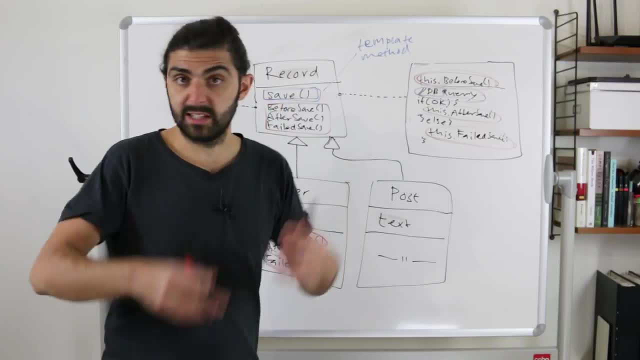 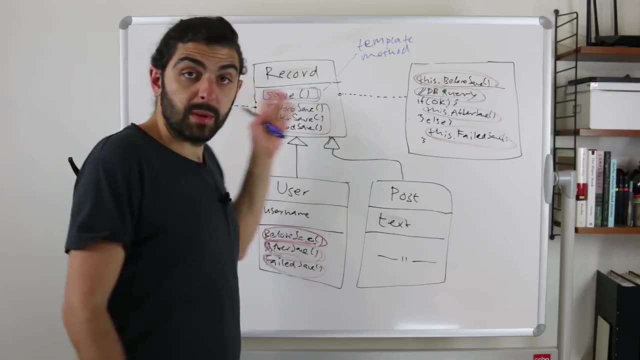 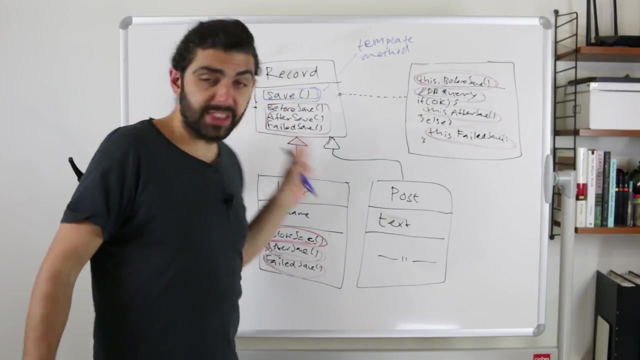 validate returns true if. if the record is valid, in other words, like: think of it as validate would make sure that your email is formatted appropriately and whatnot. and so maybe the save method is: is, is validate like it's. instead of saying save, it says validate. and then let's only think about the hook. 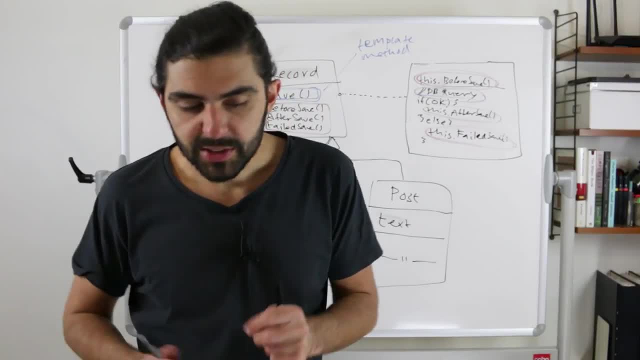 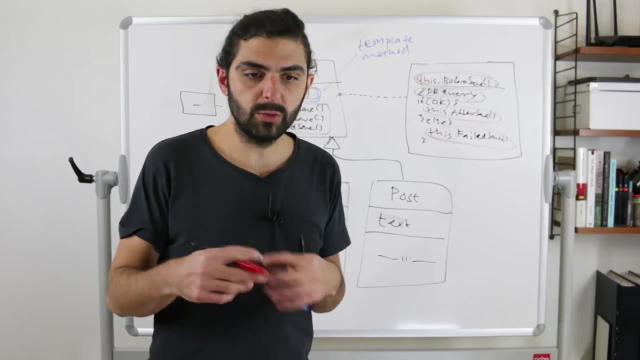 or before validation. why would we want to hook into that? i mean, maybe the scenario is this: maybe let's say that we have usernames right and there are some common transformations that we know that we can do to usernames to make them valid even if they're not valid. so let's say that, you know we 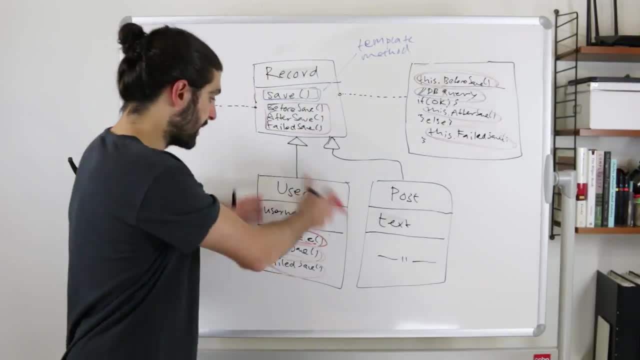 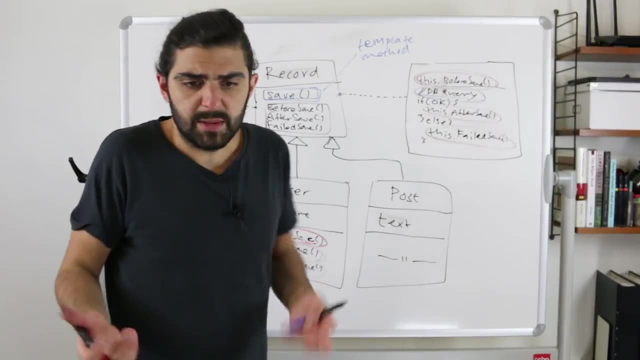 we disallow spaces in usernames and let's say we have a record, a user record, where somebody has typed in or i mean it's been instantiated with a username that contains spaces. then let's say: i mean, our default rule is that we just transform all spaces to underscores. 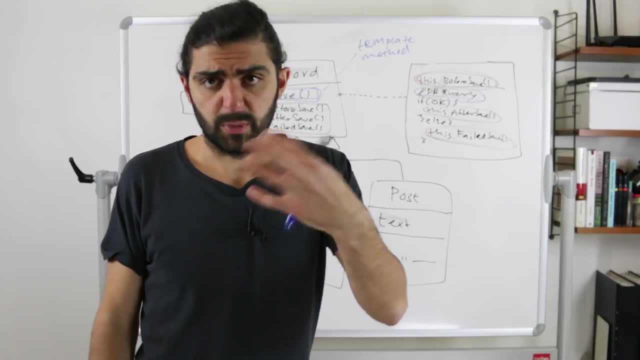 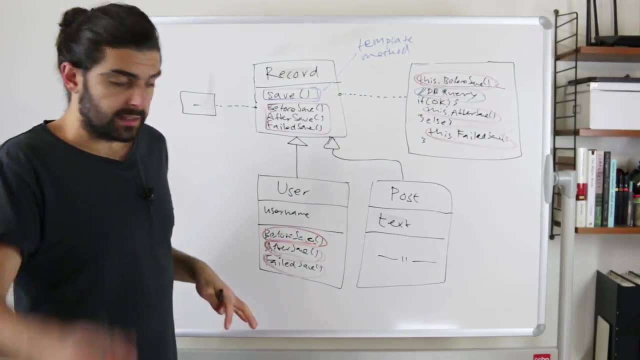 or all spaces to to dashes. i mean, don't think about this from a usability perspective. maybe that makes no sense in your scenario. that's, that's not what the discussion is about. let's say that that is your scenario, that that makes sense. then what we could do is, instead of putting that logic, 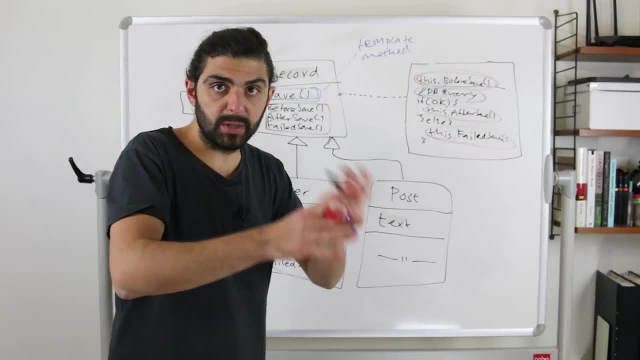 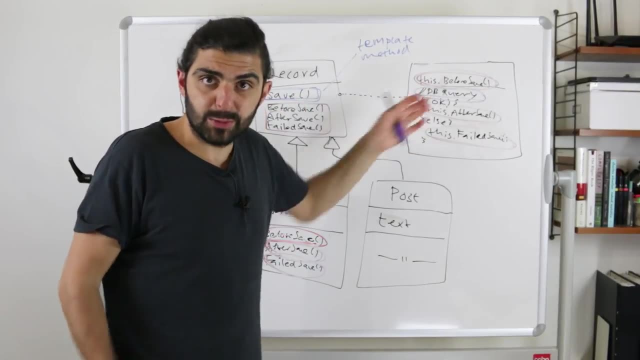 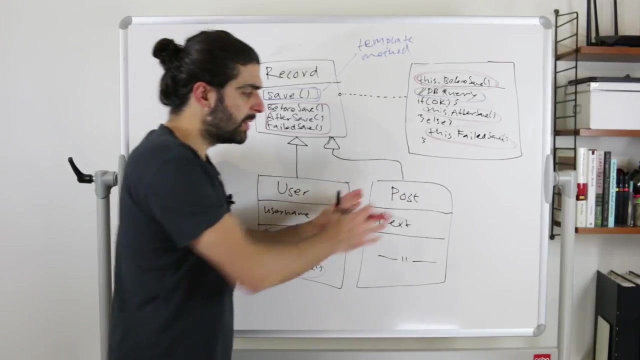 in the validation step right. instead of making that part of the validation, we could put that into the before hook before validation. so when we call validate, the validate template would first call before validate and in before validate we would do a few transformations that make sense within the user record, right. similarly, maybe the post can have that, so maybe the post. 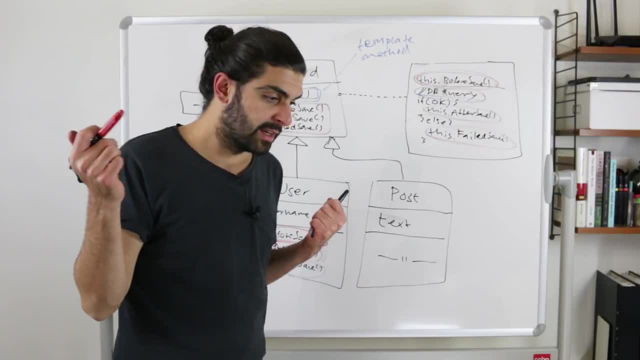 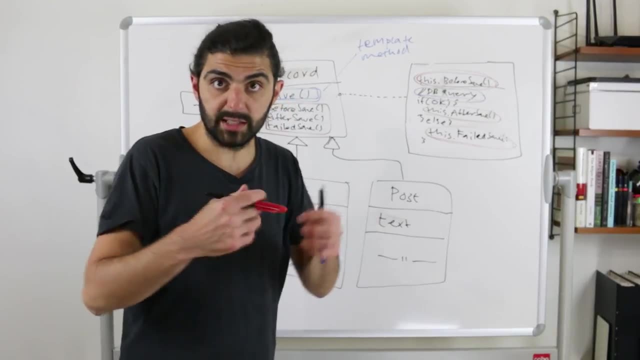 let's think about it. maybe, maybe the post contains uh. so let's say we're about to display the post on a web page and maybe the post contains html. so we need to escape the html right, like we need to make. if you're not familiar with escaping, i mean the notion of turning what could be misinterpreted- 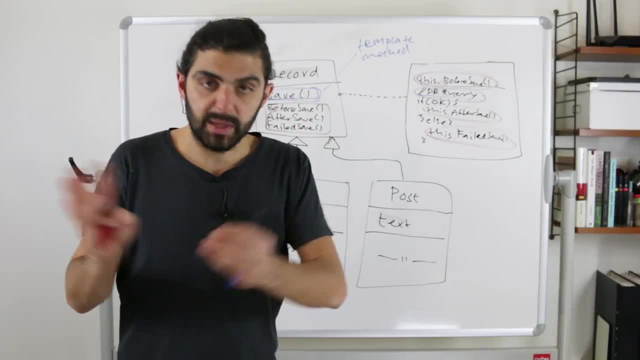 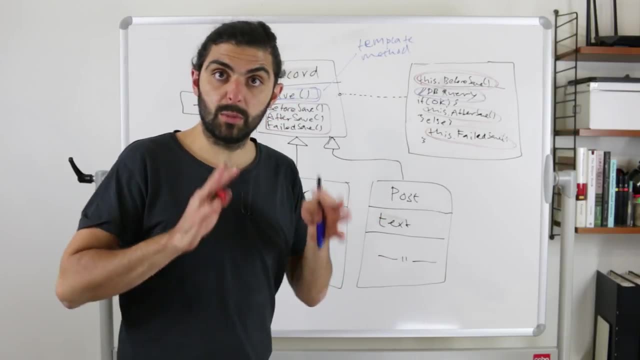 as executable code into what is unambiguously interpreted as text. so maybe that's something we do, like we do safe transformations of the text to make sure that we're able to make sure that there are no malicious code in the text. maybe that would be before validation right. 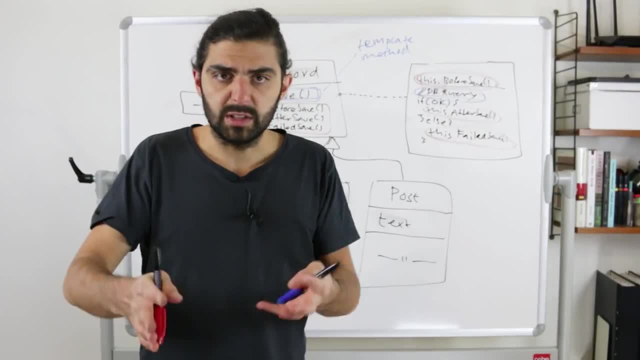 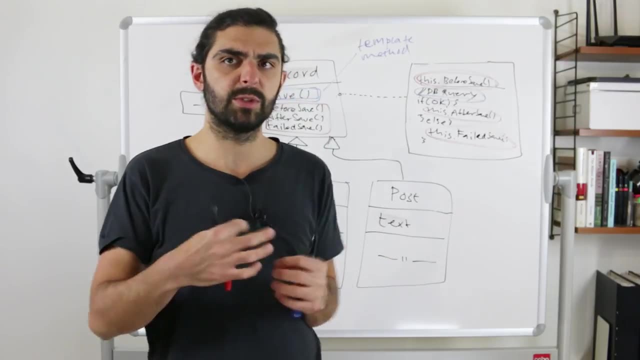 because that's the thing we can do. we can just apply it idempotently if you're, if you're familiar with that kind of thing, and it makes sense to do that before the validation, because if we didn't do that the validation might fail. but the validation would fail for a bad reason, because 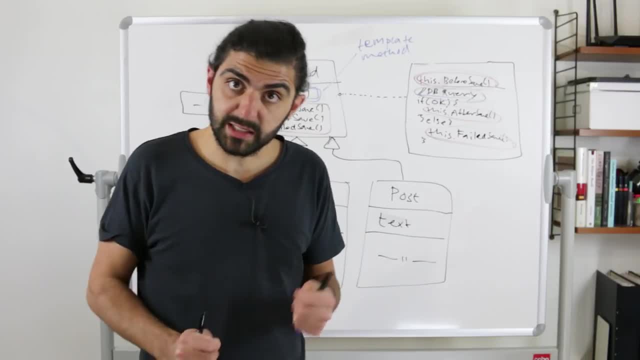 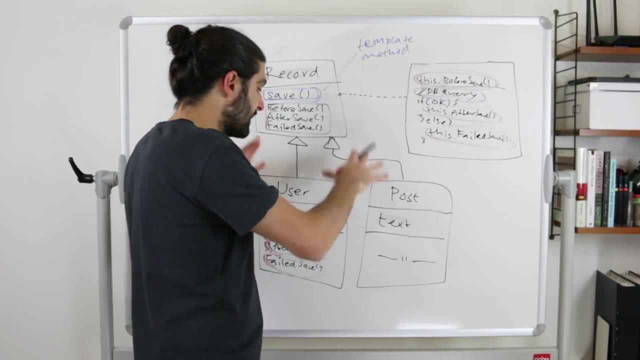 we could have fixed it such that the validation would succeed, but then of course i mean the notion of validation in this scenario- would be tricky, because then maybe the validation, the actual validation, probably also has to be delegated down to the user and to the post, unless of 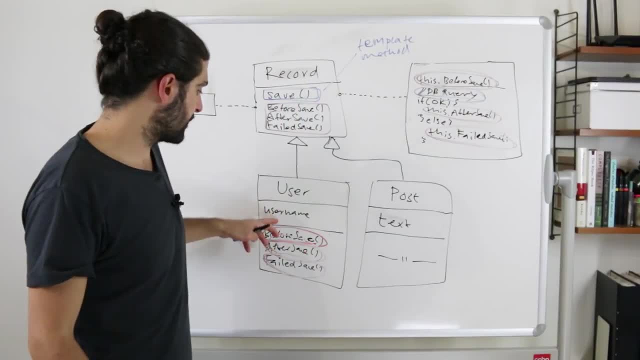 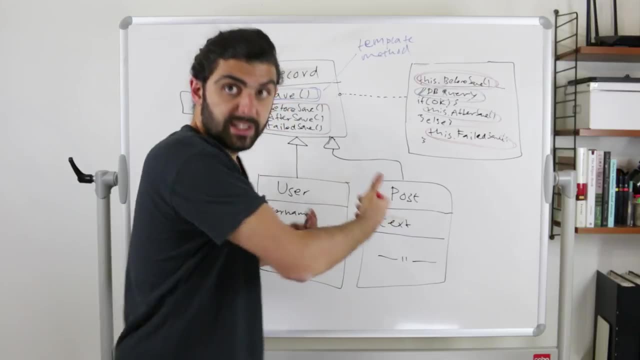 course, like if you're from the rails world, you know that you would probably not describe your properties, like username and text, as just properties, but rather you would use these helper methods that give you a lot more than just the fields. it actually gives you validation for those fields, but now, i mean, this is a totally different discussion. you could even 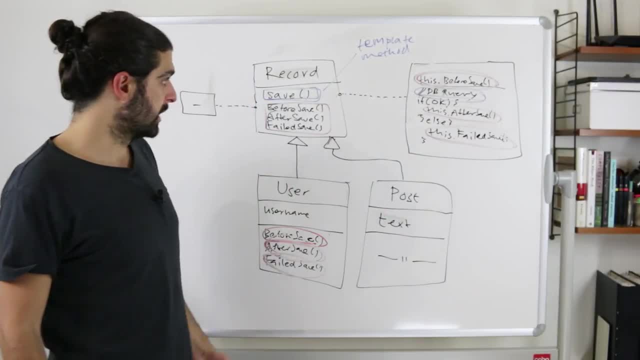 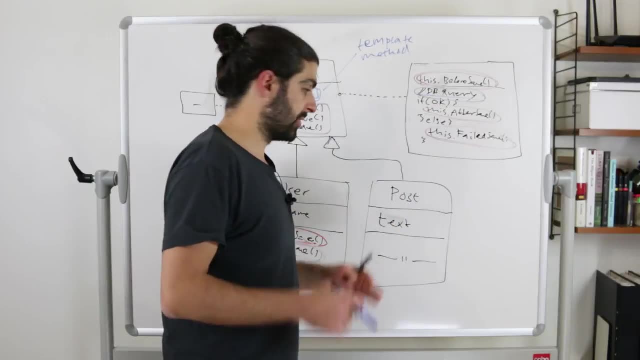 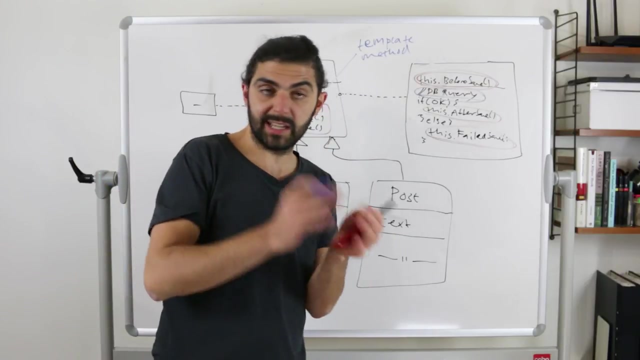 just make validation part of of the user and part of the post. so then the template method would simply just say: before validate and then validate. so it's just essentially making sure that you do those two things in that order and that you're separating the notion of before validation- like cleanup before validation and validation. 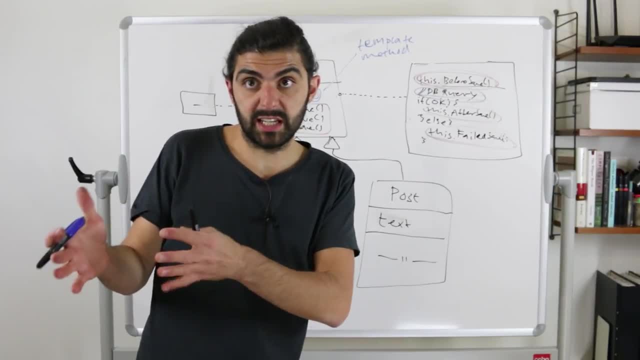 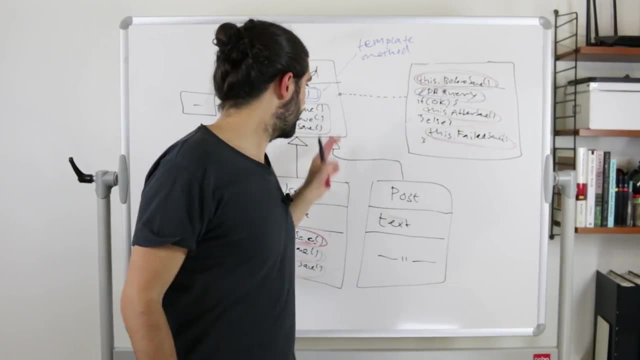 but then maybe you could do the same thing as here. so like maybe if the validation succeeds you would do one thing, and if the validation fails you would do another thing and all that. and then like maybe that starts to make a bit more sense, so that it makes sense that 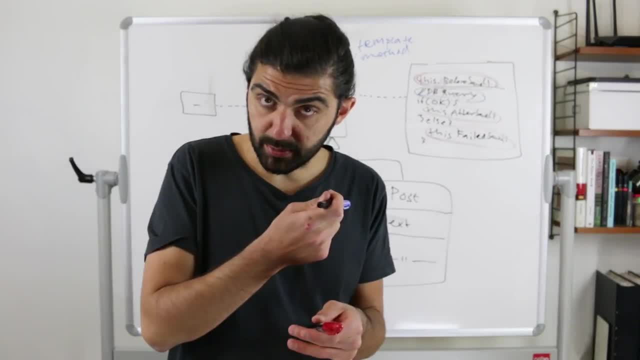 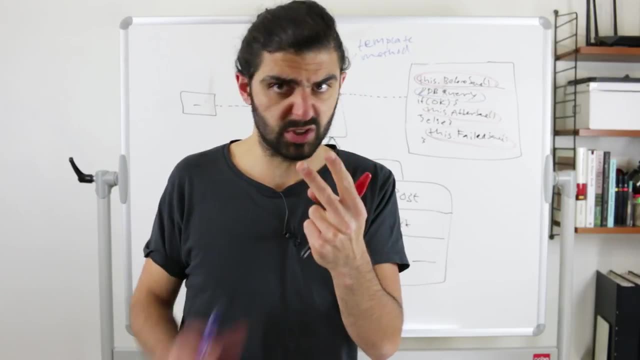 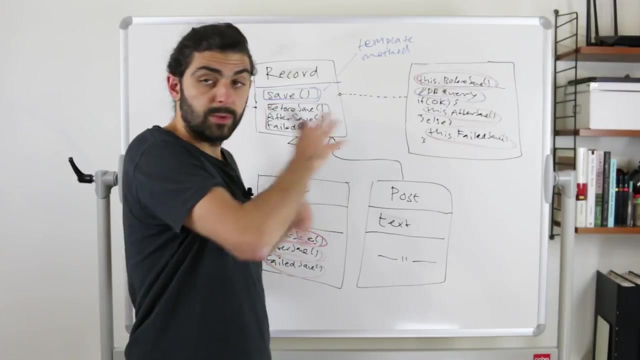 we're using the template method pattern anyways, i hope that example makes sense. before we wrap up, i want to tell you about one principle and then i want to super quickly look at some example code, just some pieces of it. is that, humorously, this book? and this book mentions that- using the template method pattern. 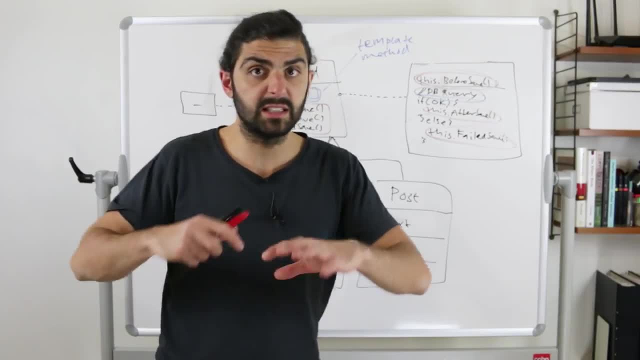 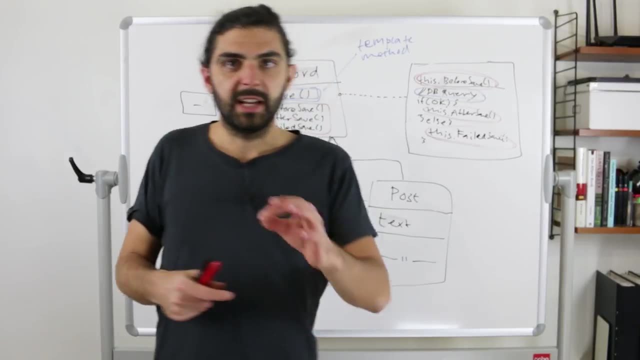 puts you in a situation where you're sort of inverting the control, as in dependency inversion right, you're inverting the control structure like you're inverting who calls who, in some sense- and i say humorously, because then they say: this is also known as a hollywood. 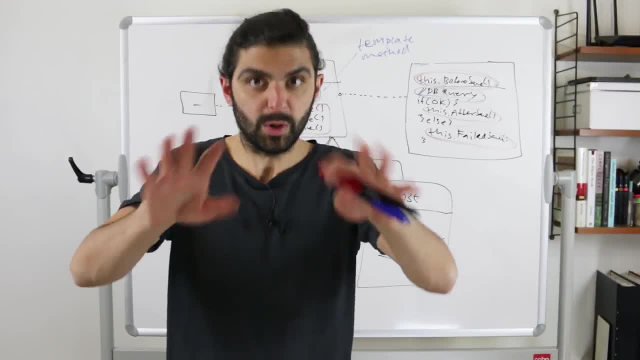 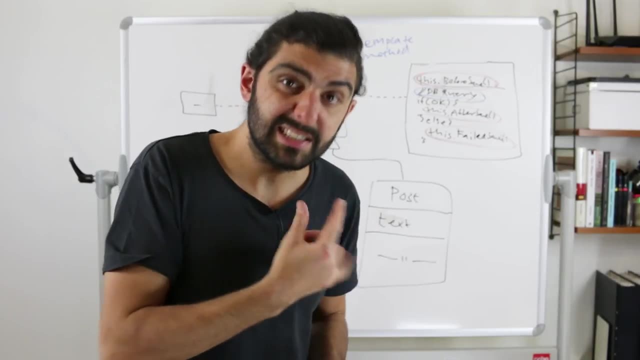 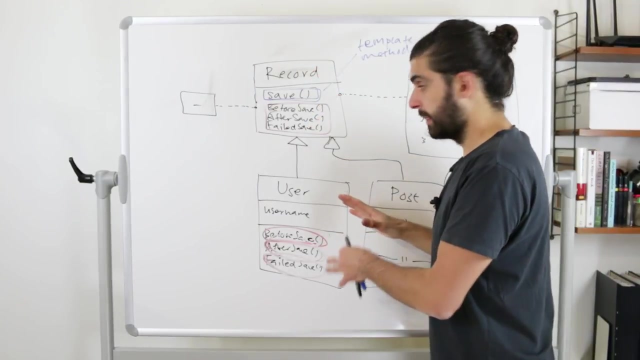 principle: don't call us, we'll call you. don't keep asking us if you got the job, don't worry, we'll call you, right or not. and actually i mean that's exactly what happens here. even if it's silly, i mean it's exactly what's happening. what happens here, right like record says: okay, user don't. 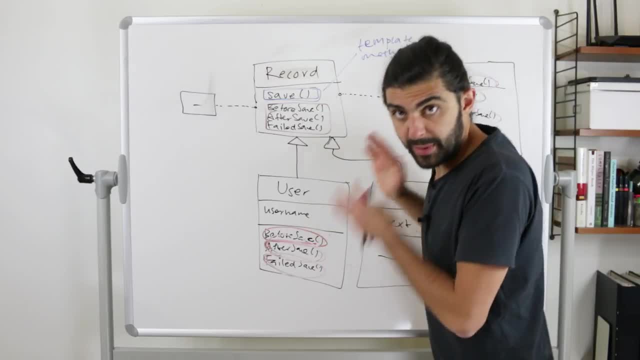 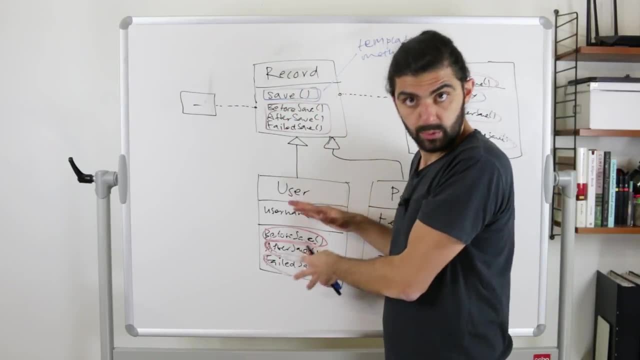 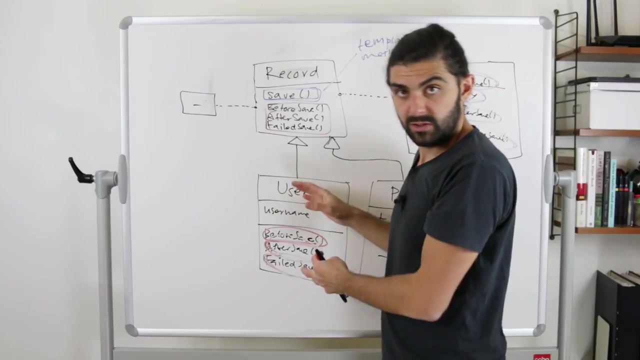 worry about whether i've saved or or whether i'm about to save, or whether i successfully saved or not. right, don't worry about that. i record will call you user when that happens. the abstract record will delegate down to the specialization user whenever it needs to, and this is the hollywood principle it's saying. 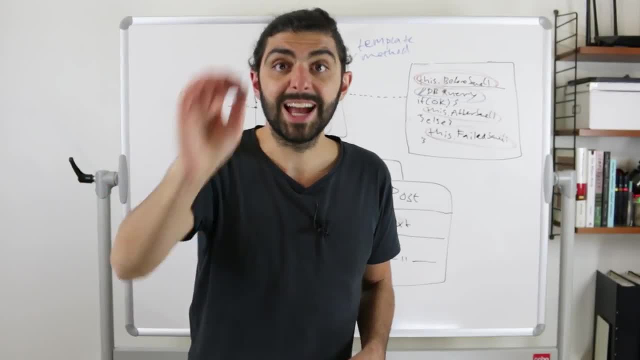 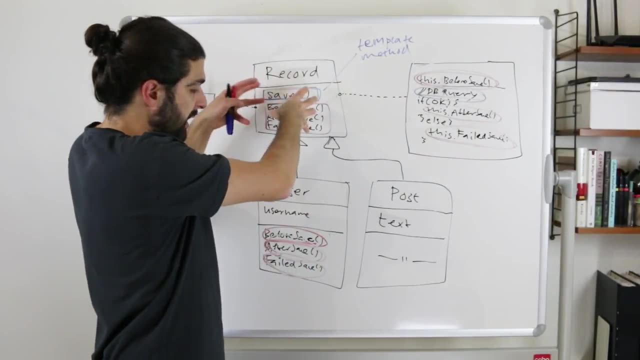 don't worry about asking me when you should perform this particular thing. i will tell you, i will delegate down to you, i will call you and that's the sort of inversion. so this more high level concept is delegating down to this low level concept instead of this. 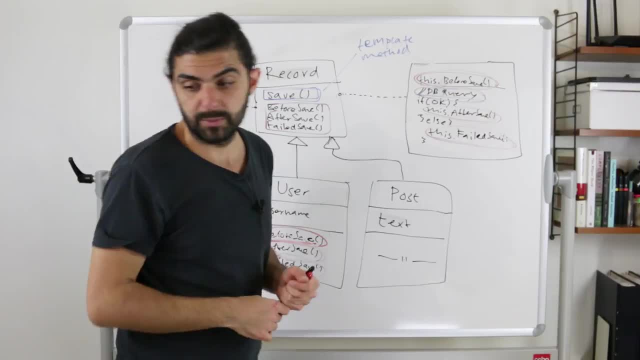 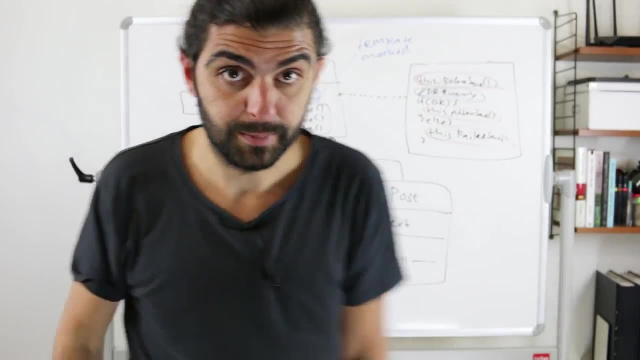 low level concept, asking the high level concept, and this is a deep discussion where you can dig down and talk about dependency inversion, but let's do about. but let's do that some other time. now let's look at some code, let's remove this. so, to keep this short and snazzy, 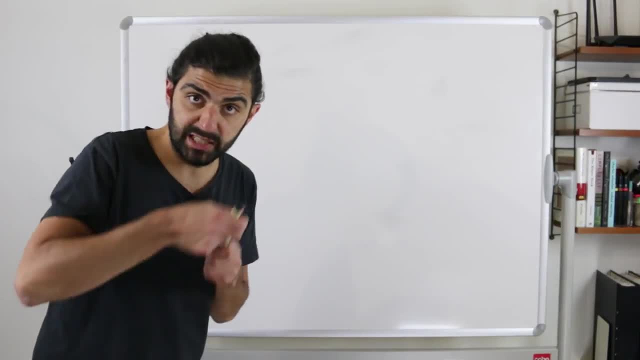 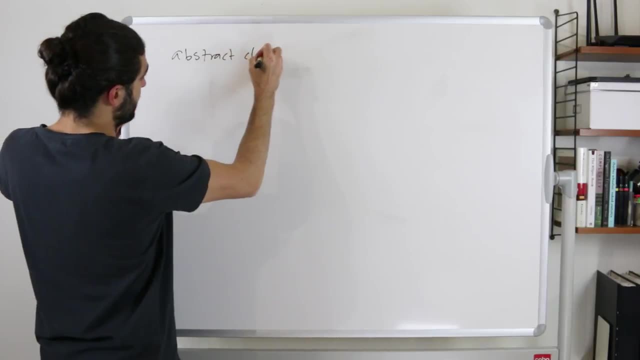 let's go to the next one and we'll only do sort of brief snippets and we'll simplify the scenario from before. but let's talk about, but let's use the record example. so let's say that we have an abstract class, abstract class called record, and what does this record? 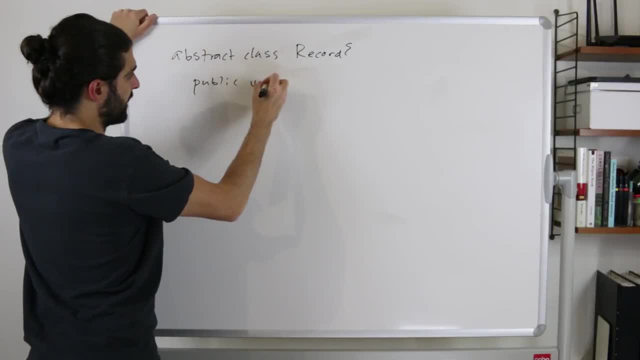 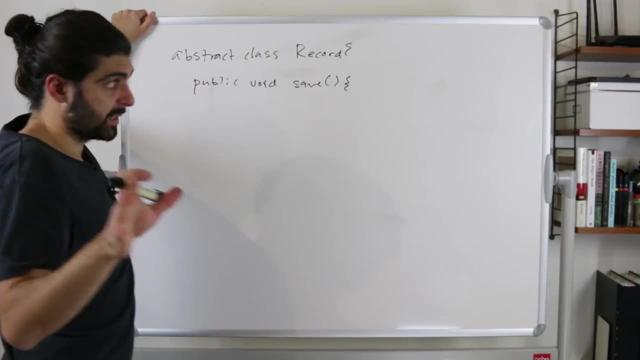 do well, this record has a public void method that's called save. let's use the save example, and what's the implementation for save? this is the template method. now, right, this is sort of the the box that we had here, the box that we had here with some implementation. let me 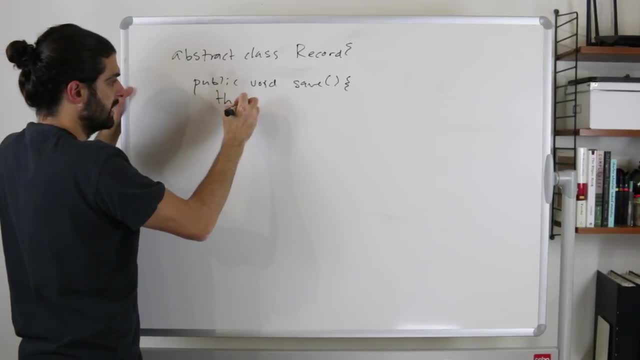 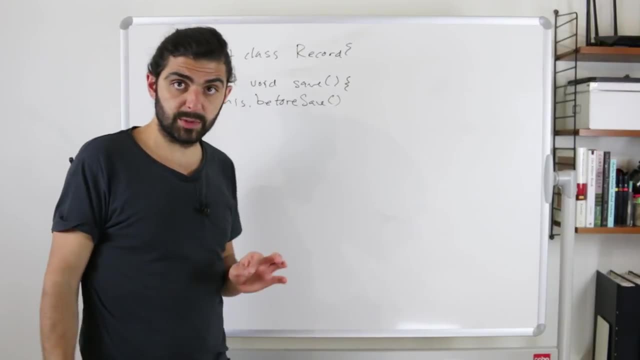 just say that what it does is that it says this dot before save, so it calls the hook. and then actually, let's redefine this. previously we talked about before save, after save, and all that and all of the examples that we took were all hooks. but let's also do some primitive. 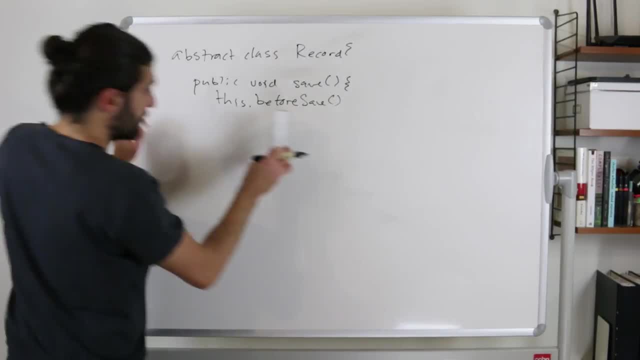 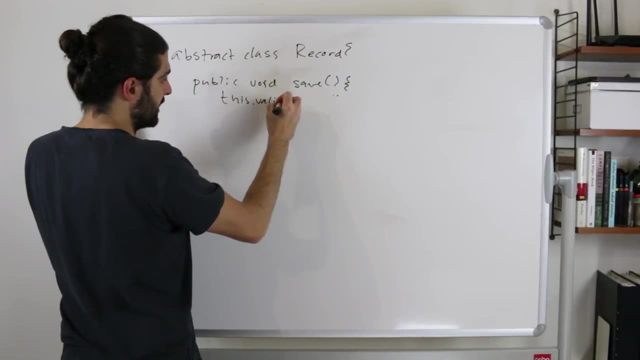 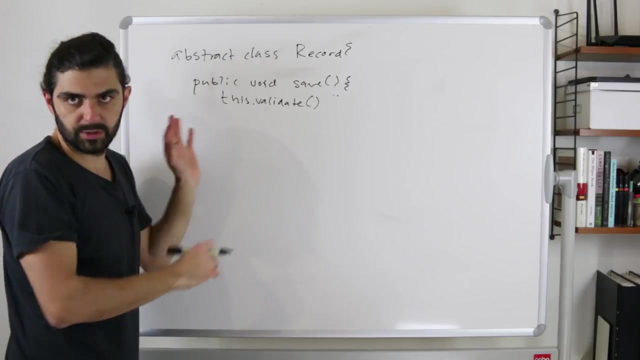 operations, in other words some abstract operations. so let's say that before you can save, you need to validate. so let's say this: dot validate. let's assume that validate can throw an error. I'm not necessarily saying that that's good design, it's just that makes me not have to. 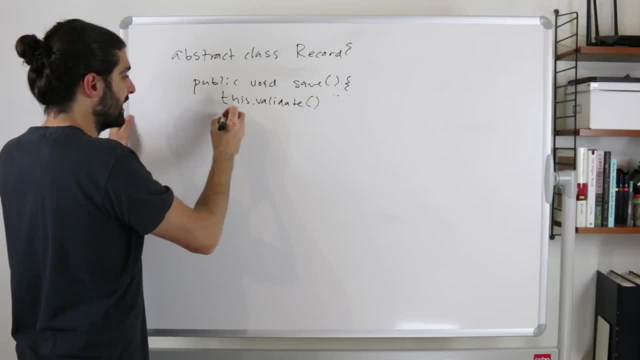 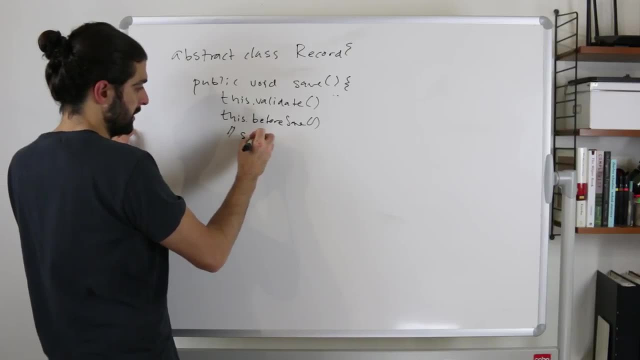 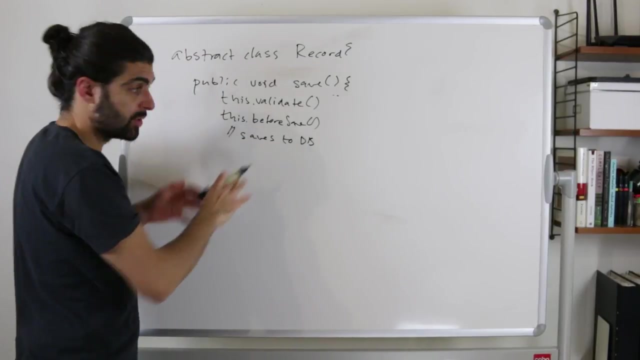 deal with the if branch here. so it's just an example. so this dot validate, and then we say this dot before save, and then the actual database query saves to db. so I'll just put a comment here, but I mean, clearly there needs to be an implementation here, and then we'll. 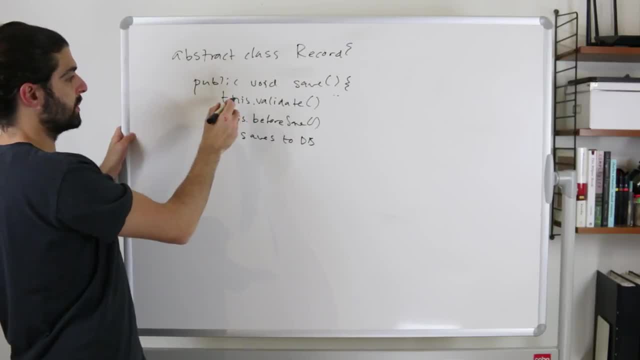 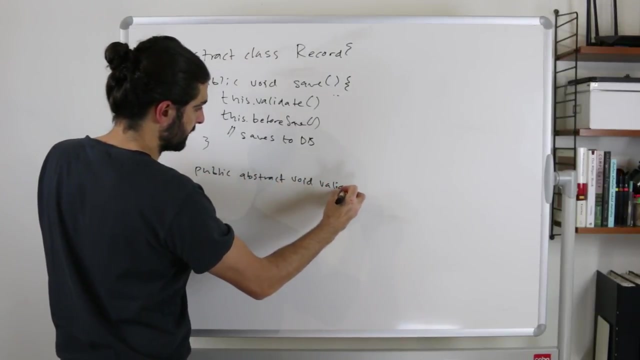 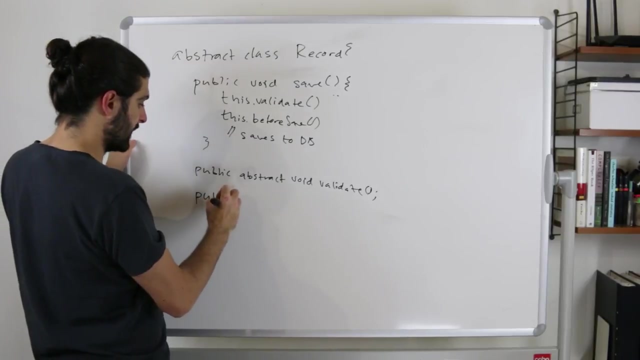 close this method and then this means that we need to specify validate right, and validate is an abstract method, so in other words, a primitive method that doesn't have an implementation in this record class. so so, public, abstract void validate, there is no implementation because this is an abstract method. then we need the method before save public and before save is a hook. 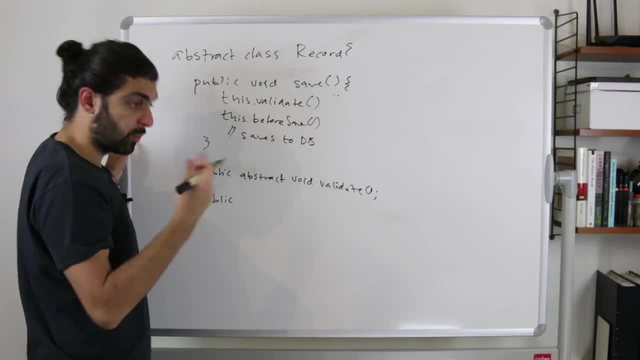 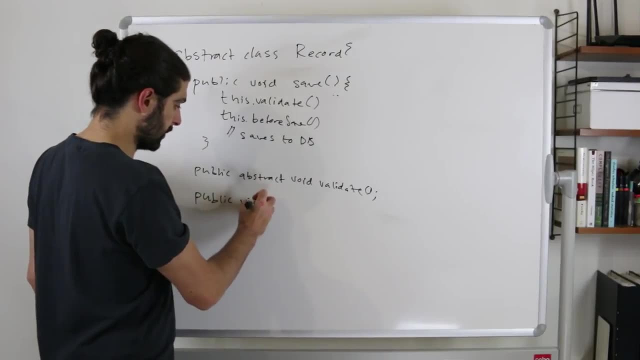 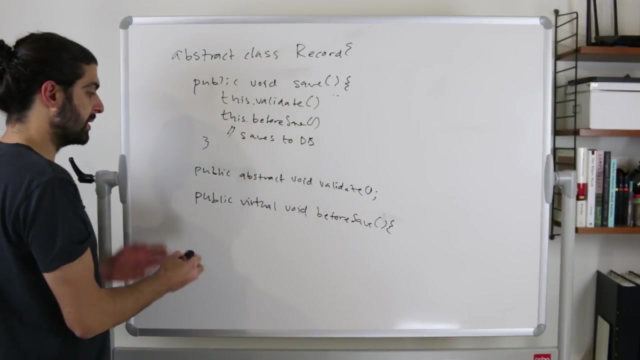 and because it's a hook, you might. it's an optional hook, you might not necessarily want to hook into it. that means we need to have a default implementation. but the default implementation is going to be empty public virtual void before save takes no arguments. but we open it for writing an implementation, but we don't. 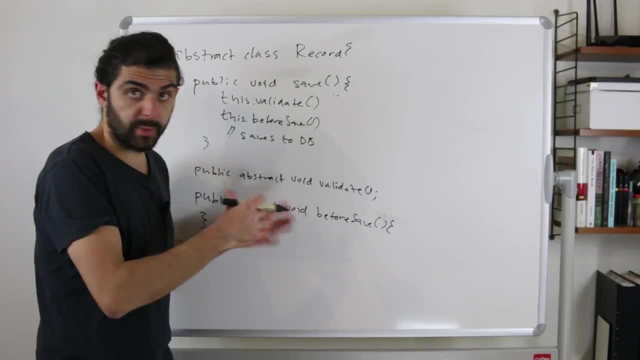 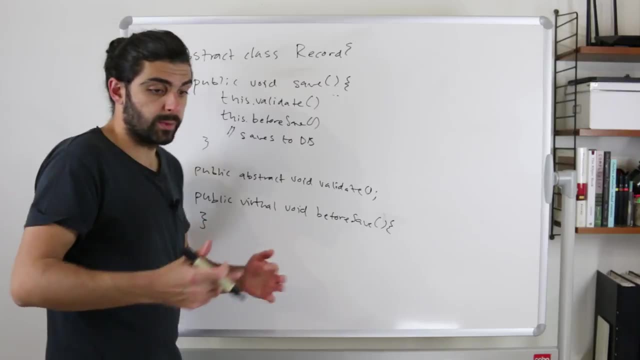 actually write an implementation. so the keyword virtual depends on your language, right? but I mean we market a virtual, we marked this virtual here so that it can be overridden in subclasses, in other words so that you can hook into the hook. but also I mean it's important. 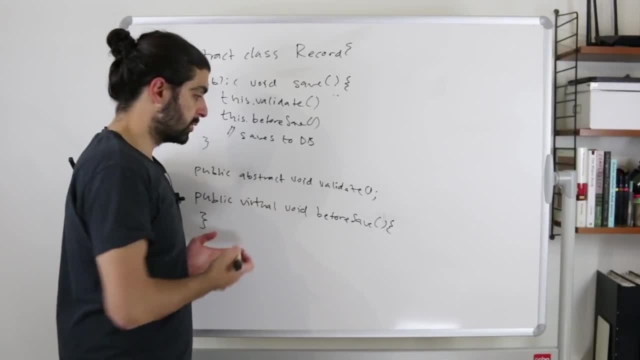 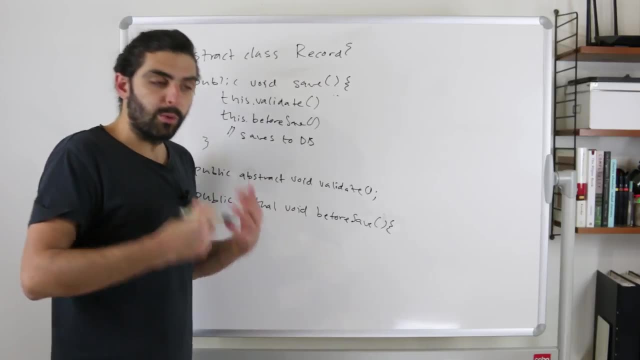 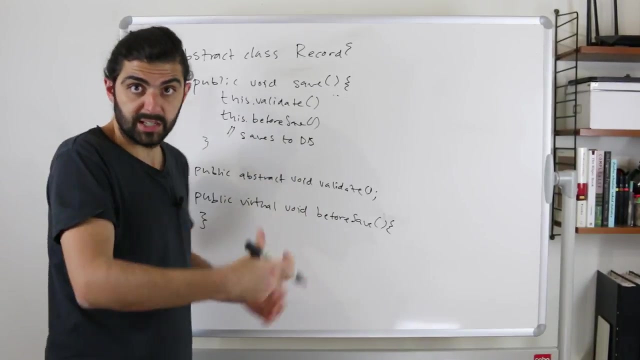 to mention that you could of course have like a default implementation here, so the virtual method could have an implementation, so that if the subclass does not provide an implementation or does not hook into the hook or override this particular method, then there is a base implementation, there is a default implementation that runs or that's used in lieu of or instead. 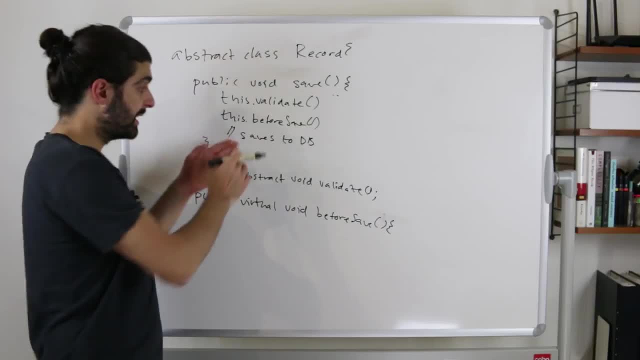 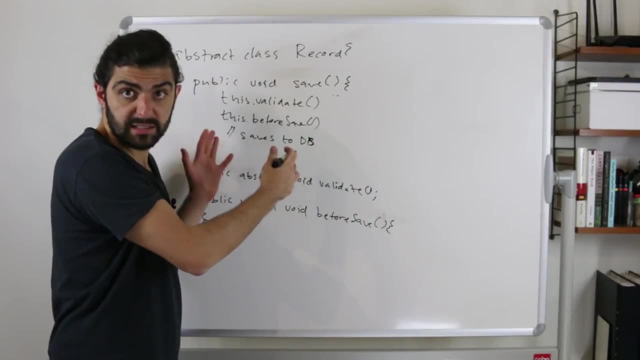 of the non-existent subclass implementation. okay, and then the. the third portion of this template method was that we saved to the db, and let's just not worry about how that is actually done, right? I mean, that depends, again, like the actual work depends, on your scenario, but this is the. 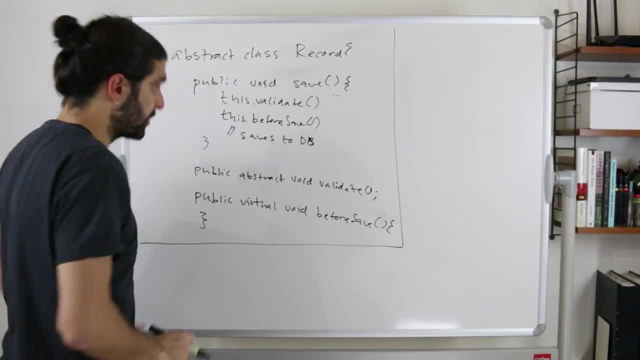 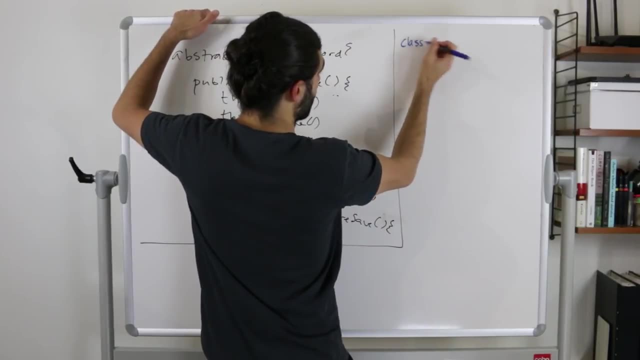 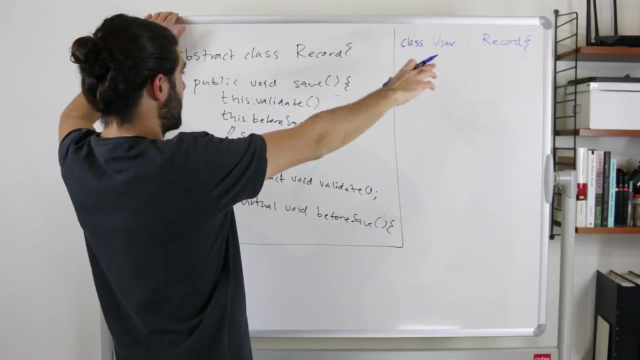 record class. that's it, and now I wish I would have left more space on the whiteboard, but life is life. let's now build the user class. let's try and build it here. so we have a class now, a concrete class called the user, and the user extends record, so the user extends from. 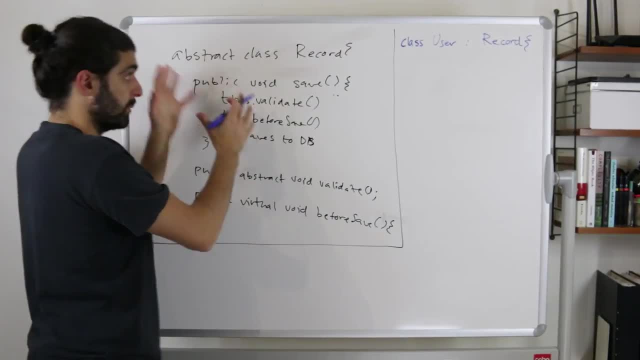 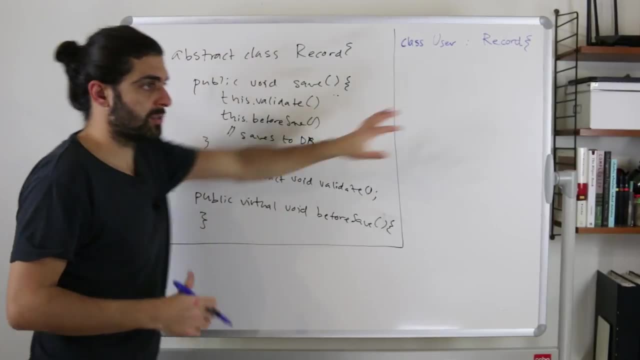 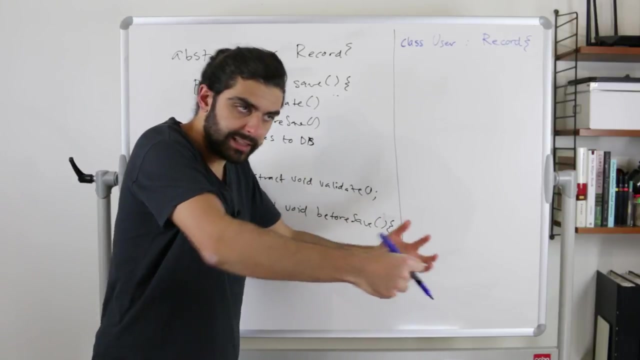 record right, which means that it will get this save method. record is the base of of users, so whenever you instantiate a user, you will you will be able to call save because users are records. user is a specialization of a record. user can supply further functionality, but it cannot. 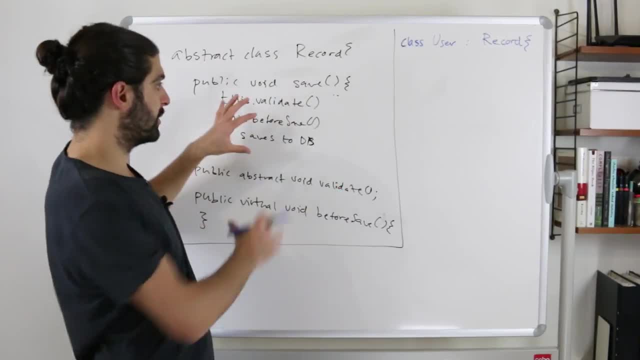 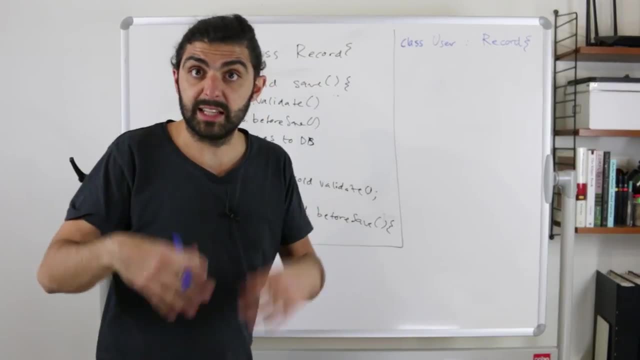 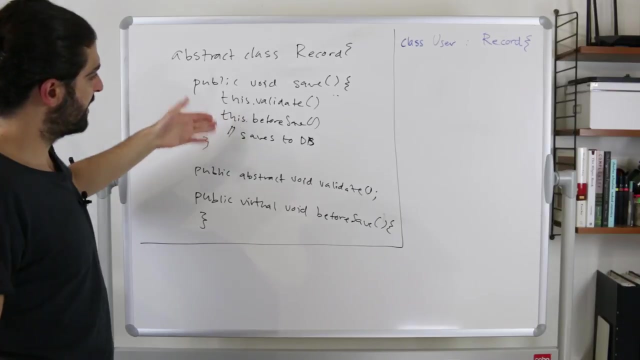 constrain what what recordness entails. so it can cannot remove the notion of having save. I mean syntactically you can, but Liskov substitution principle, semantically you shouldn't. so users are savable and when you call save it will call validate and before save and 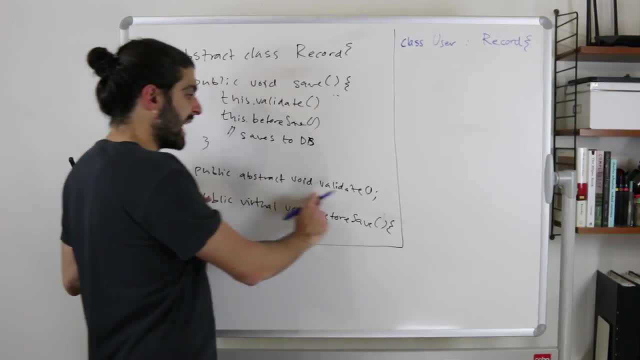 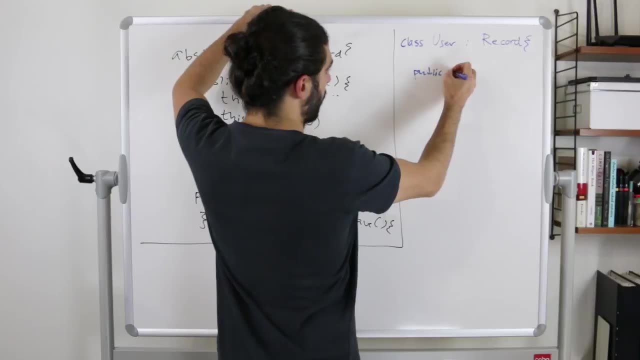 then it will actually save to the db and because we have this abstract method, we now need to override. I can't really remember the syntax of this, but let's just say that it's something like public override. maybe it's not like this, but but who cares? I mean, you see the point. 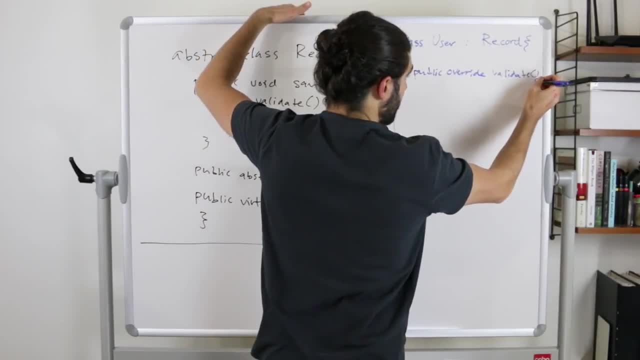 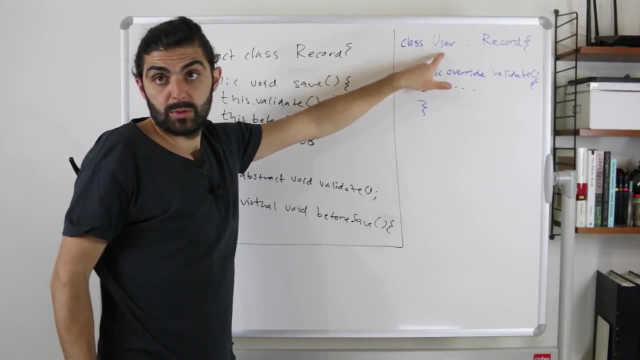 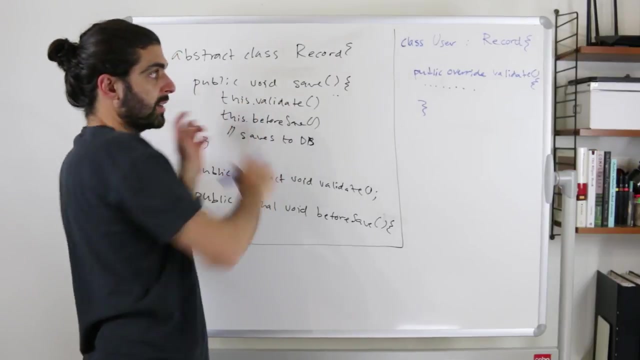 you override the method. validate takes no arguments. we open it up and then here you supply some implementation that is specific to the user. so validation, that is specific to the user record and this is why it's delegated down here in the user and not in the record. 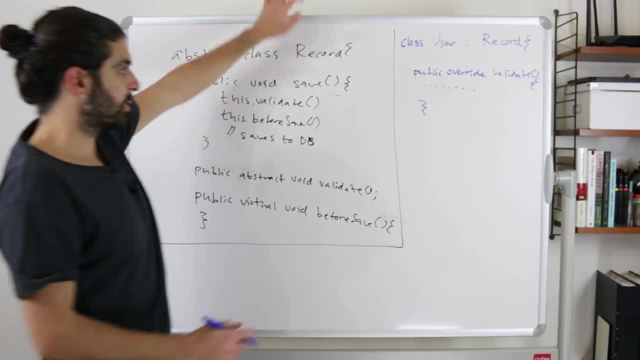 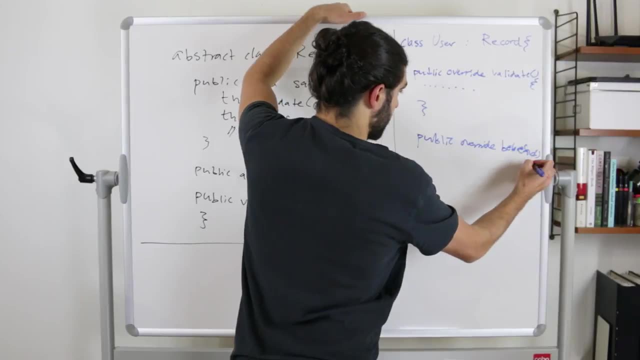 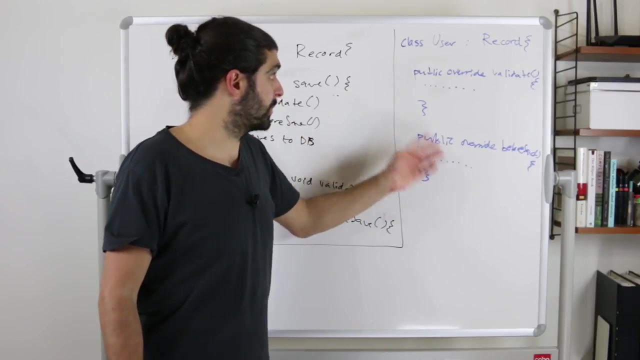 because it's user specific. then we have the hook before save and so if you, if we want to, we could say public override before save and open that up, and then we do something before save. maybe we- I mean, it was kind of a bad example because I don't really know what users would want to do before save- 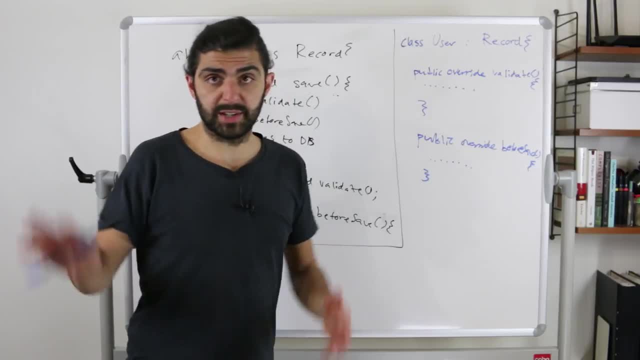 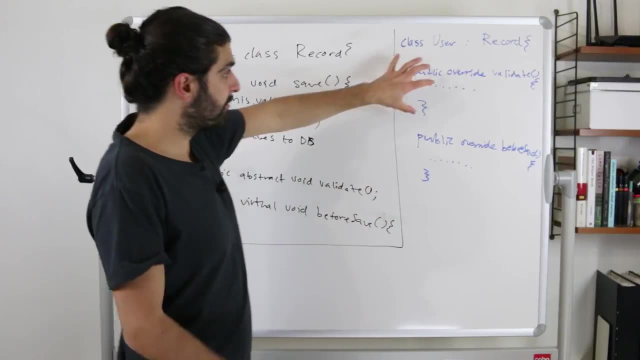 that's specific to users and not really specific to, and wouldn't be applicable for comments or something like that, I don't know. okay, but either way, I mean we have this hook that we can hook into if we want to, the validate thing we have to do, we. we have to do it because 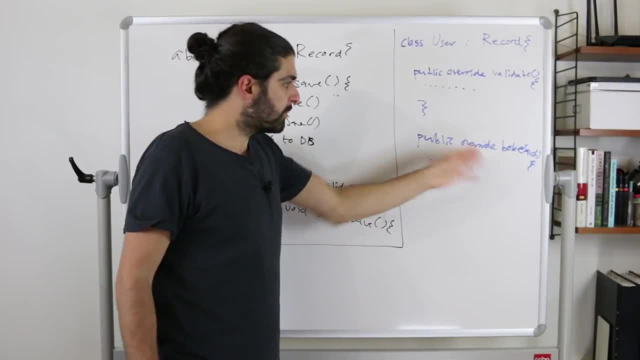 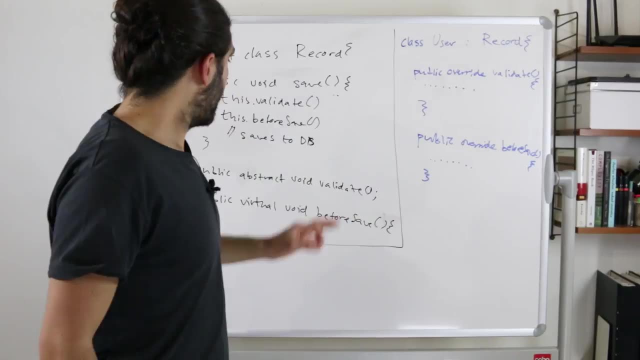 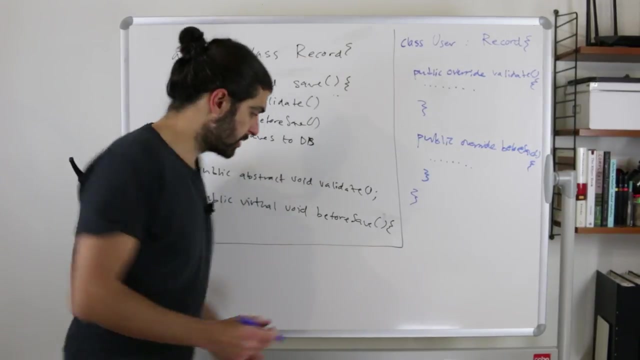 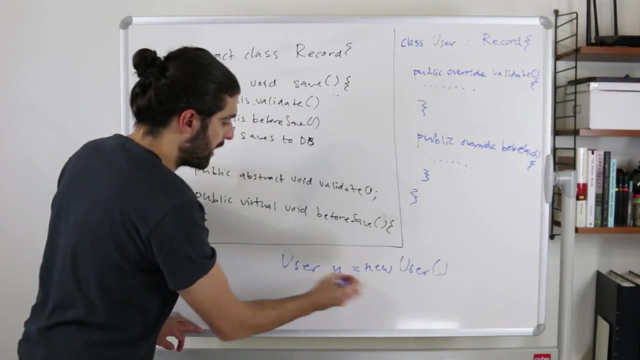 there is no implementation in the record. however, before save: We don't have to do. I mean, it's optional, It's a hook. we can hook into it if we want to. if we don't want to, No infinite reci värz, Then we don't. we have to do. anything more in the user class and we just close the user class and suddenly the user is saveable. so so we can say user, this just called u equals a new user. and now that's you. we can say U dot save. and when we call save, what will happen? let's trace it, the result. 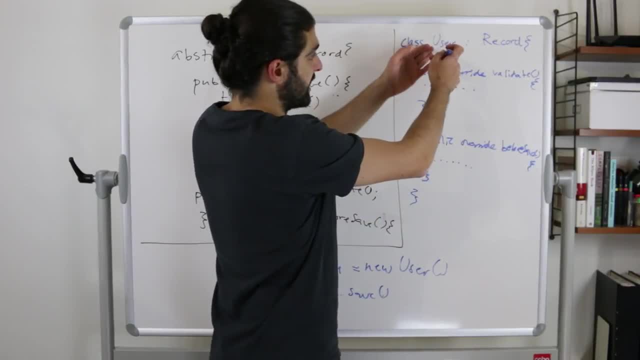 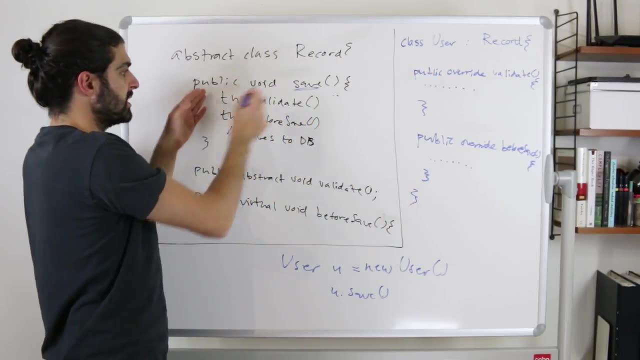 this: When we call save, we'll end up in the user and it says: okay, I don't have a save method. My base class has a save method. okay, Here's the save method. The first thing that happens is that: 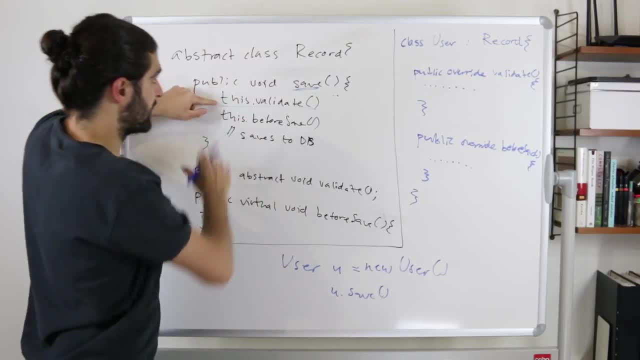 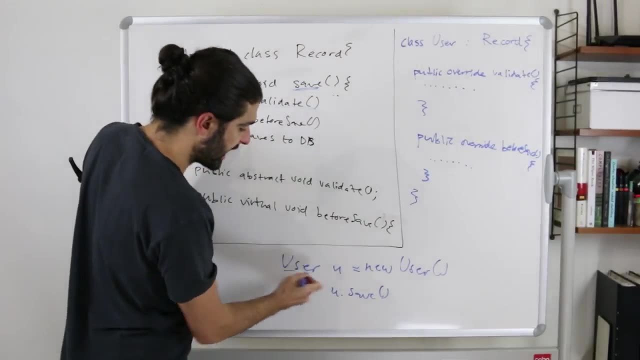 we say thisvalidate. Well, actually validate here is abstract. So I, the base class, don't have an implementation for the validate method. Instead, my specialization that you happen to have, ie the user that happens to have an implementation for the validate method. So we 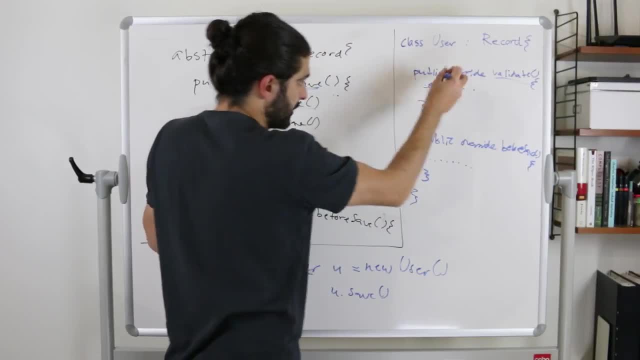 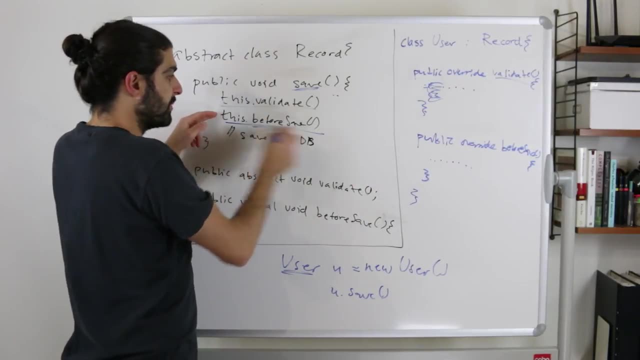 end up here in this validate and then we execute all of this code, whatever the validation does, And then when we exit that, we're back here in the save method and then we say, okay, do this before save, run this before save, hook right And again before save is virtual here. 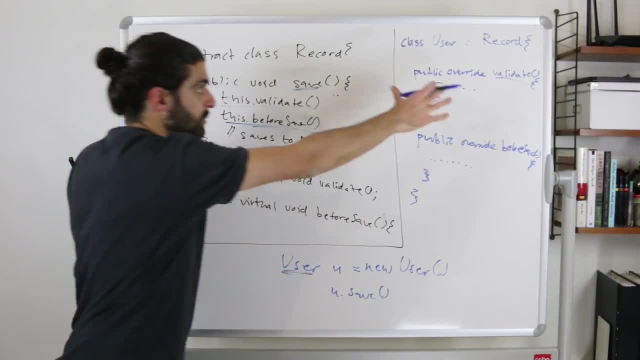 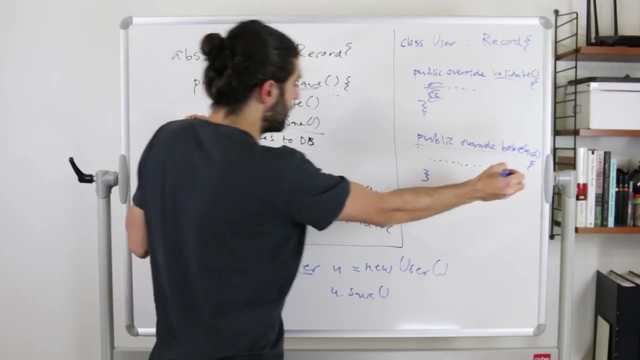 right. So there is an implementation. but because we're in the specialization, because we're in the user, we actually have a specialization here, an overridden specialization. So then we run this right, We run the hook And then when we exit this before save hook. 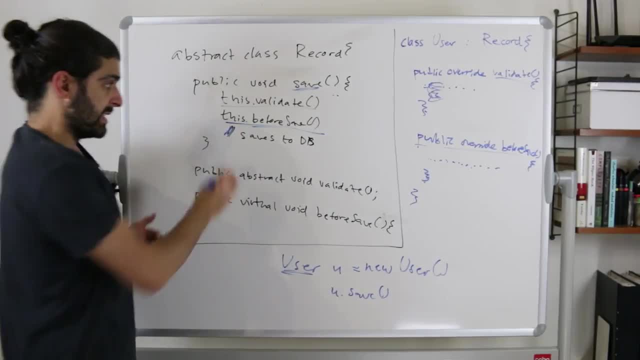 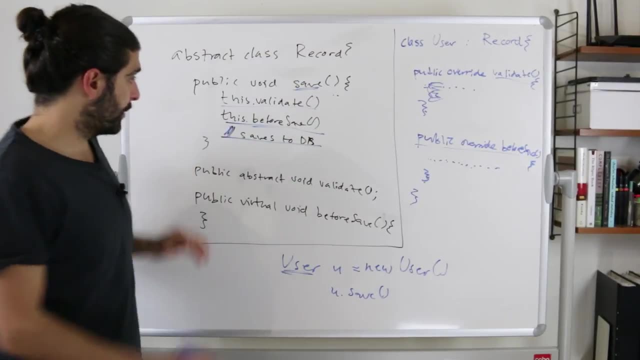 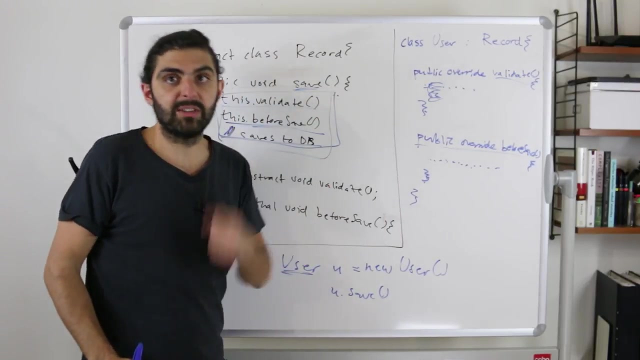 whoop, we're back here And now we're at this comment that says saves to DB. So supposedly at this point the record would be saved to the DB. But again we were able to keep this algorithm, this notion of first validating, then doing something before we save, and then actually 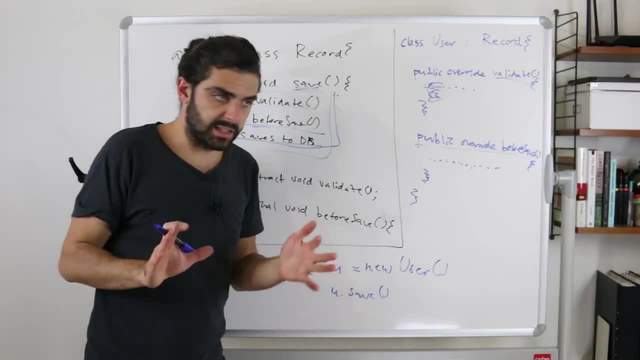 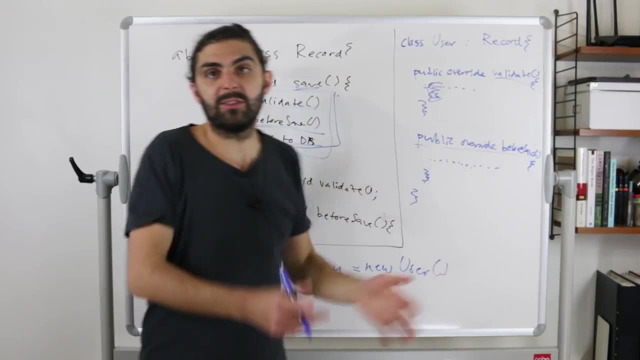 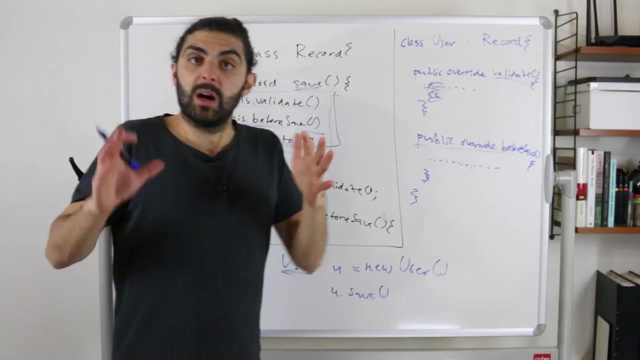 saving This structure, we were able to keep consistent without having to write that in the user, And when I say consistent here I mean consistent across this user and, for example, a comment And a post, et cetera. So, amongst our different specializations of the record, amongst our